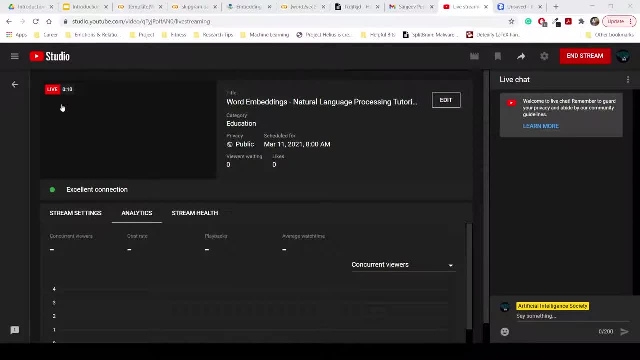 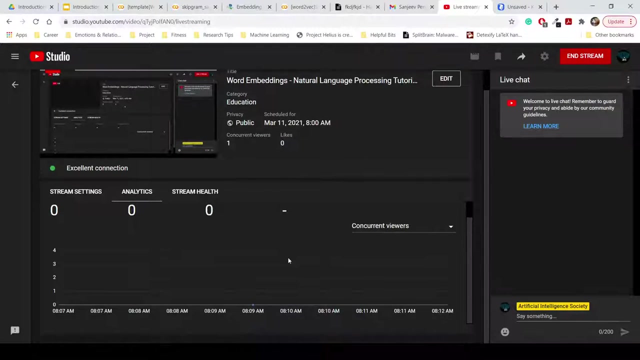 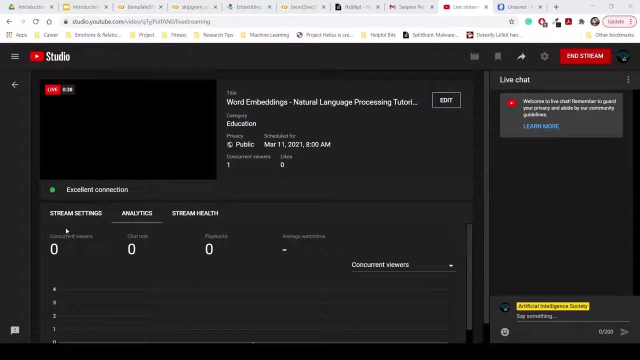 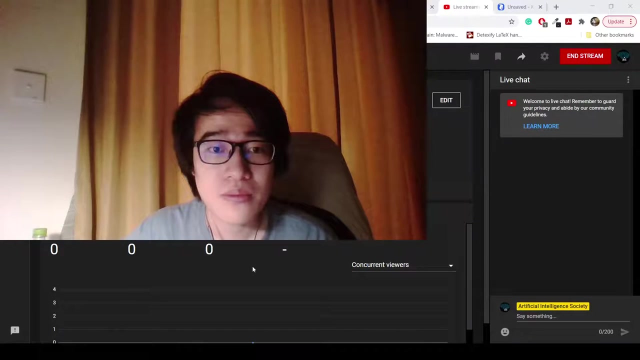 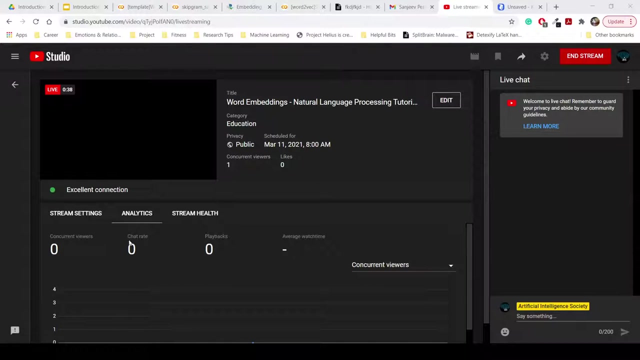 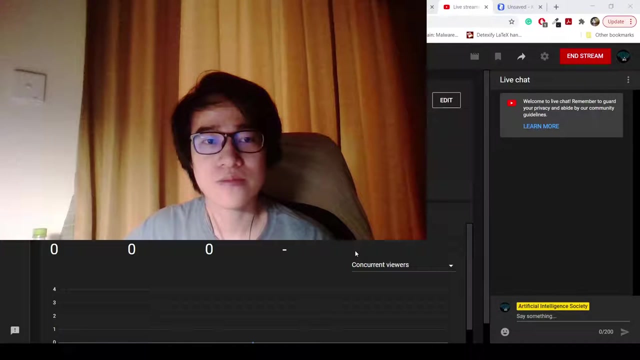 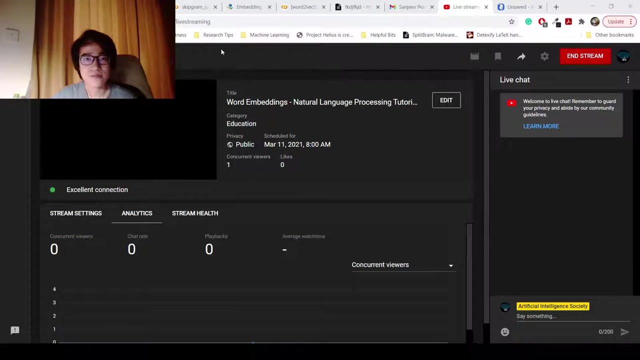 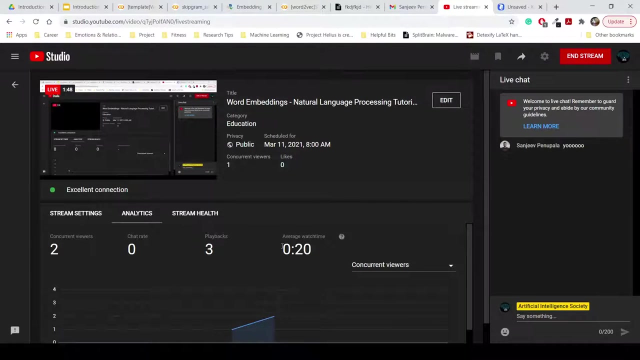 Okay, Okay. can everyone hear me? Can anyone hear me at all? Okay, I'm just like no viewer right now. All right, All right, Okay, so we are currently having three people on the stream. That's pretty nice. 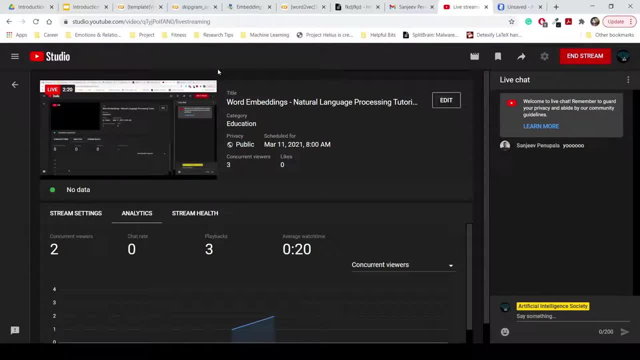 Hello Sanjeev. Okay, can everyone hear me right now? If everyone can hear me right now just like type something in the chat, like quite a bit at a time, I don't know. Hello, Okay, Sanjeev can hear me, That's nice. 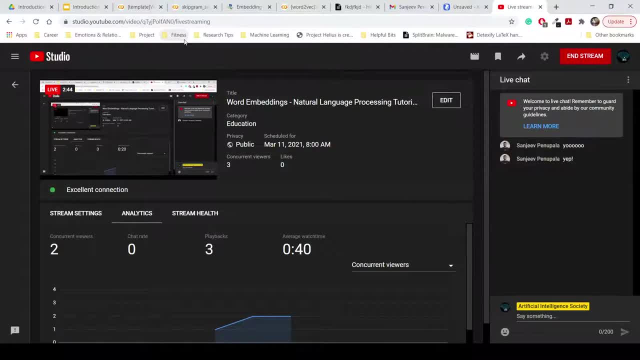 Okay, Joe, are you there? Yeah, so on today's workshop, Joe's going to, Joe's going to help us with the workshop, like answering the question in the chat and stuff like that. so, yeah, Joe, let me know if you like, if you are up and ready. 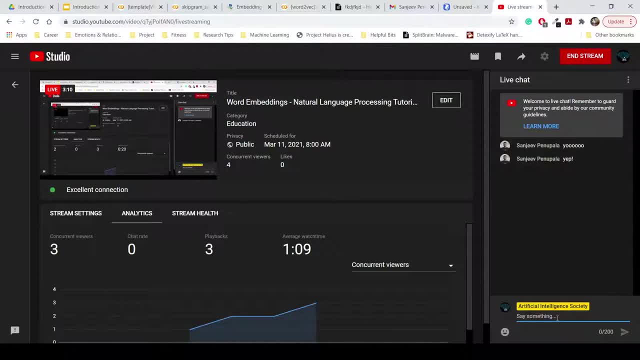 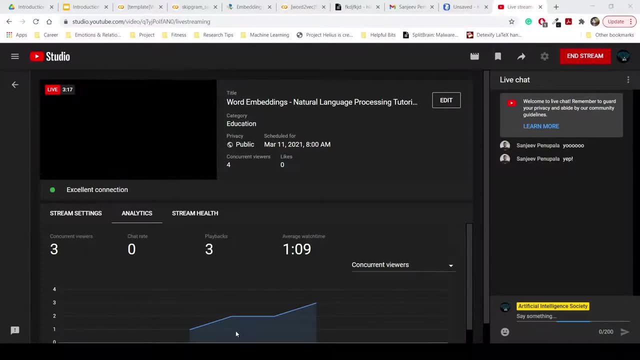 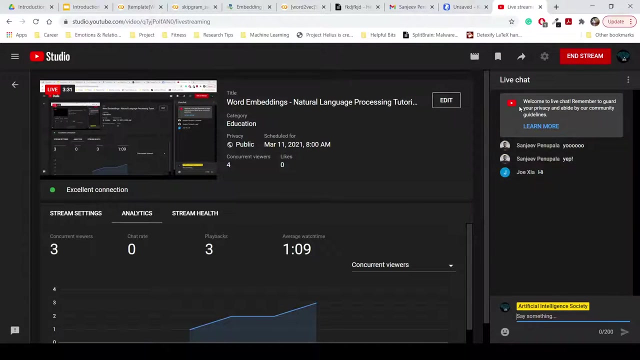 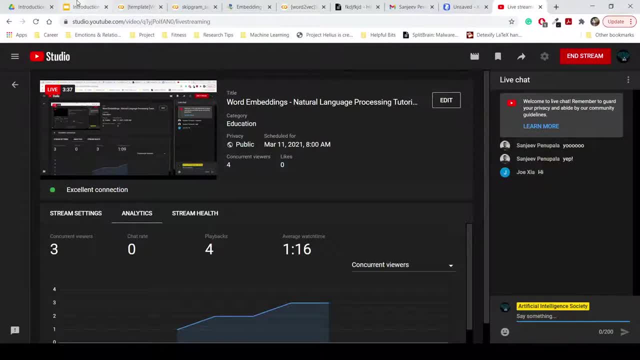 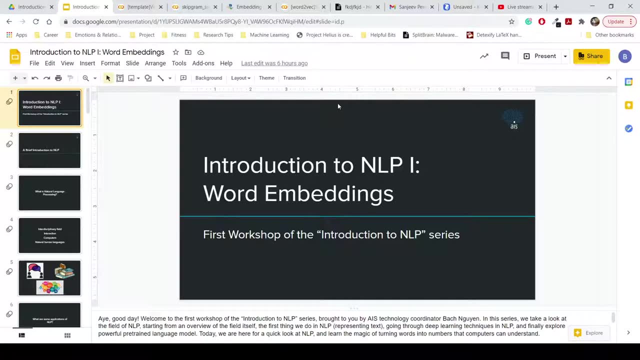 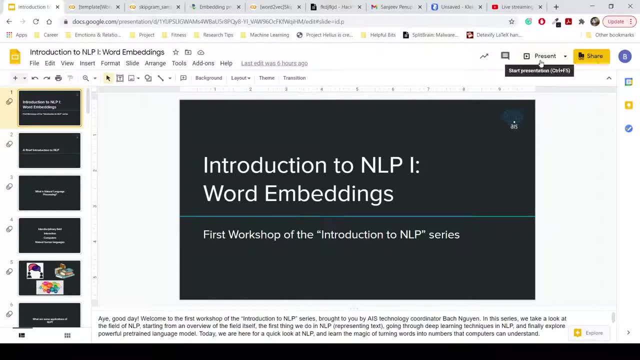 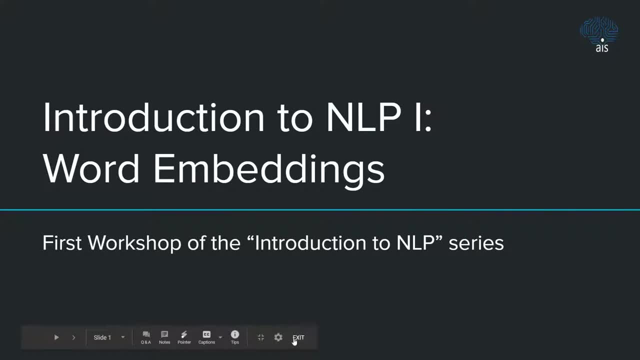 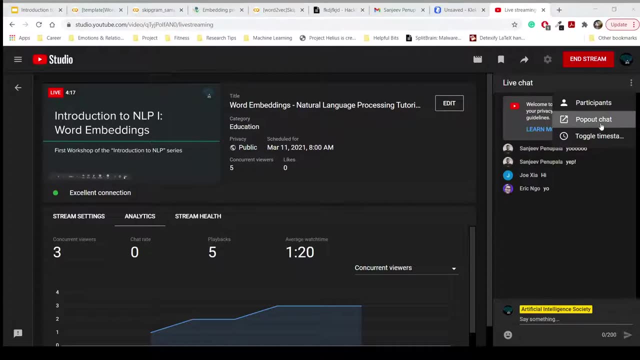 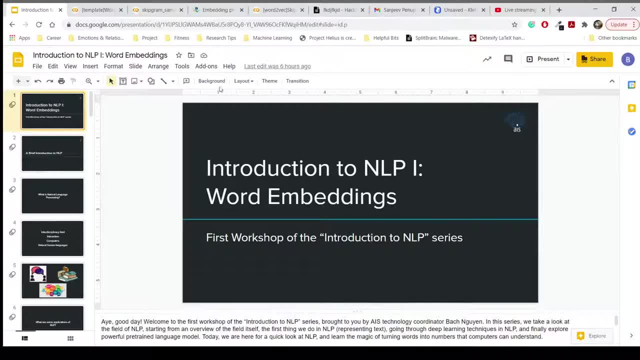 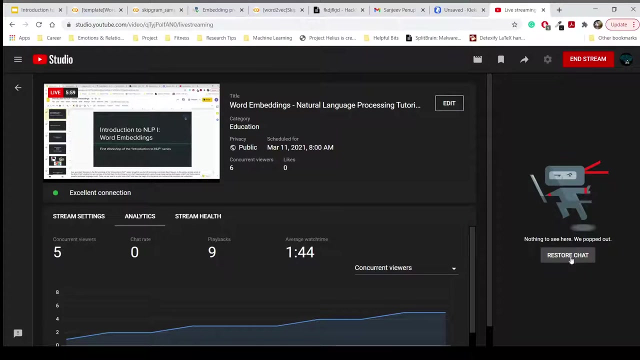 screen. so yeah, there's so many things grew up today so I'm so sorry. ready to start you, you can ask something with distortion, okay. so, Joe, can you like forward every single questions that everyone may have to be to the slack account to my? yeah, just I. 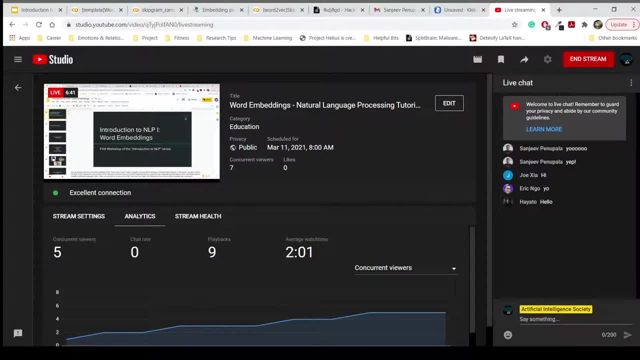 as a child something, because I cannot see your chat when I'm streaming. yeah, I'm sorry. yeah, it's for every single question to like the slack to to the side account, like that's like you send me a chest, all right. yeah, you've seen my in my. 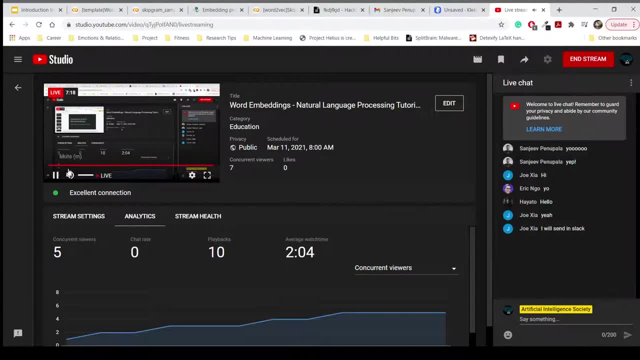 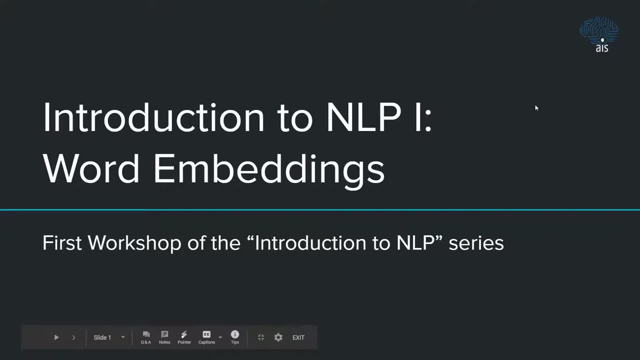 yeah, I'm in my all right, thank you. nice, okay, so we can finally start. we are 20 minutes late, so that's a bit bad, but okay. so okay, welcome everyone to the first workshop of the introduction to NLP series. and is brought to you by a. 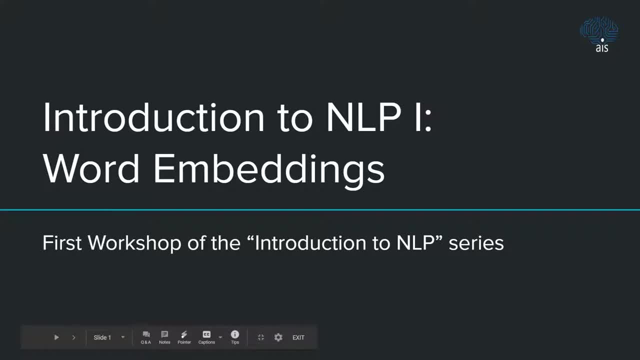 technology coordinator back when. so in this series we take a look at the field NLP, signing up for an OPM overview of the field itself, the first thing we do in NLP, which is representing text going through like d-learning techniques in the NLP, and then we finally explore powerful 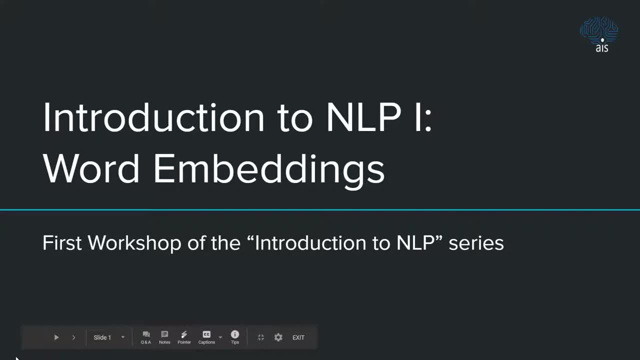 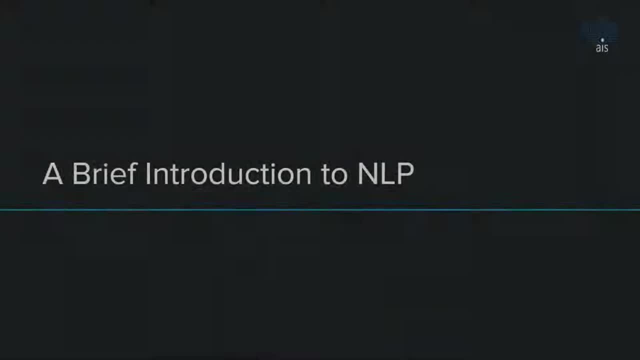 between model. So today we are here for a quick look at NLP and learn the magic of turning words into numbers that computer can understand. So before we begin this workshop with your introduction to NLP, we shall start off looking at an overview of NLP. 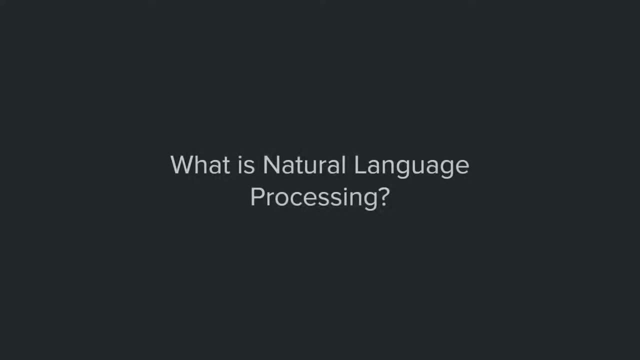 So how can we define the field of Natural Language Processing or NLP? NLP is an interdisciplinary field concerned with the interaction between computers and natural human languages. So what we mean by natural human languages are something like conversations, spoken language and written language, as in books and news. 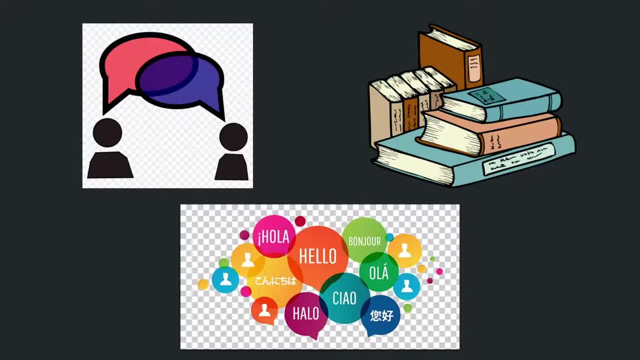 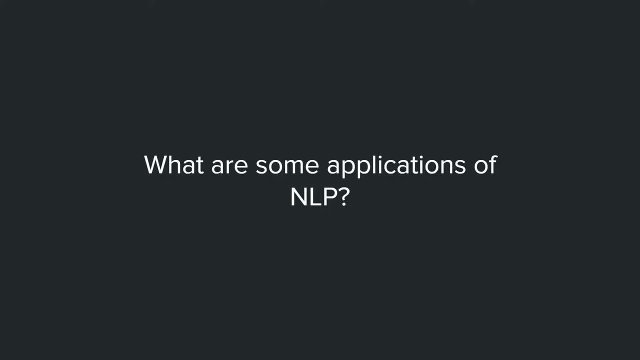 And also English, as well as our international language, are also counted into this group. So we usually have some combination of things like written English or conversational Chinese. So now that we have answered the what question of NLP, we move on to answer why of NLP. 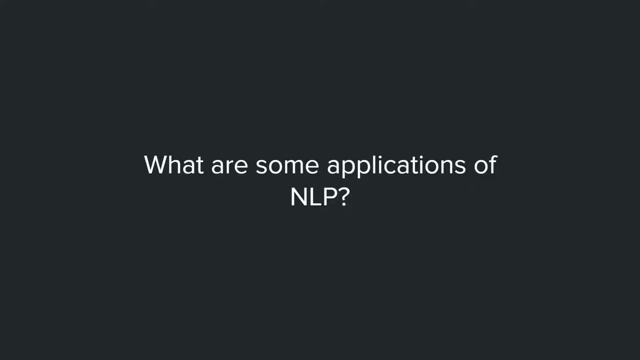 So where can we find NLP? in either industry or in our everyday lives? So let's start with NLP. What is NLP? What is NLP? So one very useful task of NLP is conversational agents, also called chatbot. 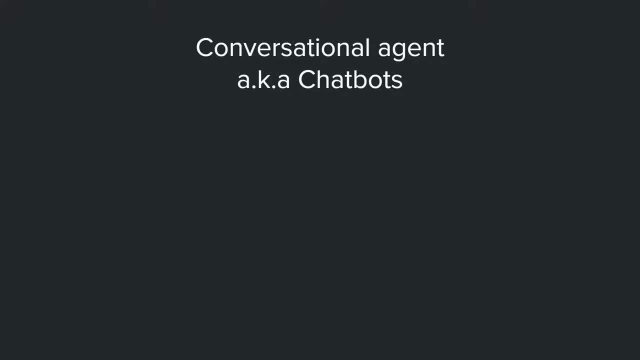 If someone here have seen, like 2001, A Space Odyssey, then they will know that Hal 9000 is a very, very capable AI. He is like he can speak and understand perfect English and even like comprehend emotions in the speech. And also something that's more close to everyone here. 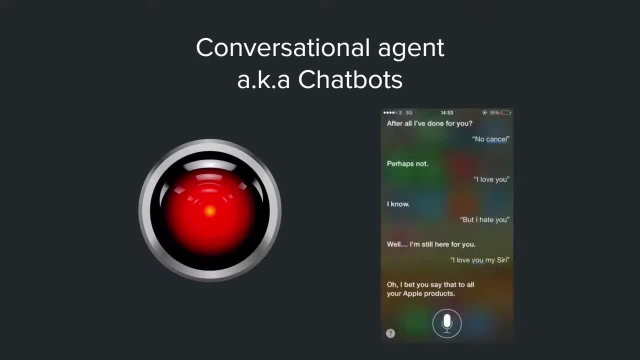 It's probably something like Siri, a virtual assistant featured in most Apple products, And yeah, yeah, it's available in your pocket And it is a form of conversational agent. It's very fancy way to say chatbot. Another popular language related text is machine translation. 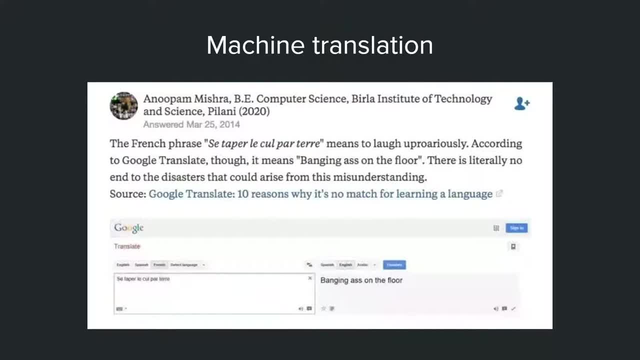 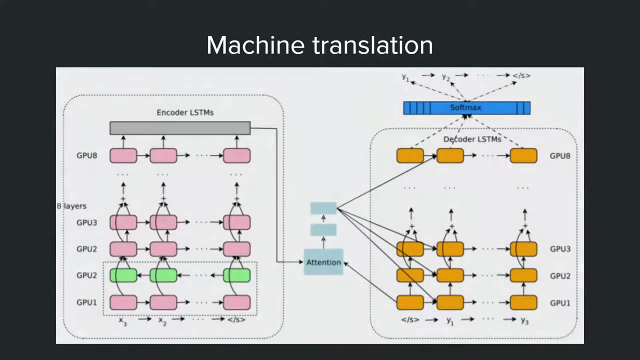 So machine translation is like nowhere near being perfect, but they are also nowhere near being simple. So we have something, a model that looks like this, translating, like translating language in like a really slapdash way, but is actually a model that looks like this, costing a lot. 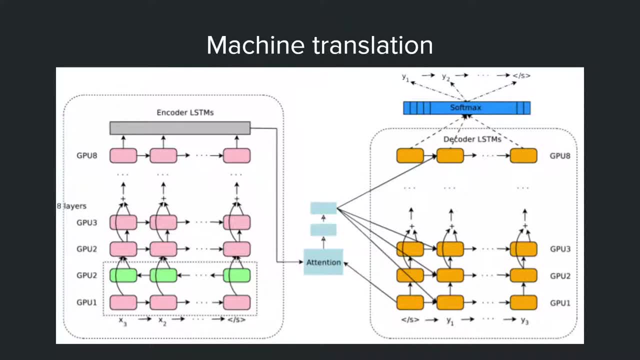 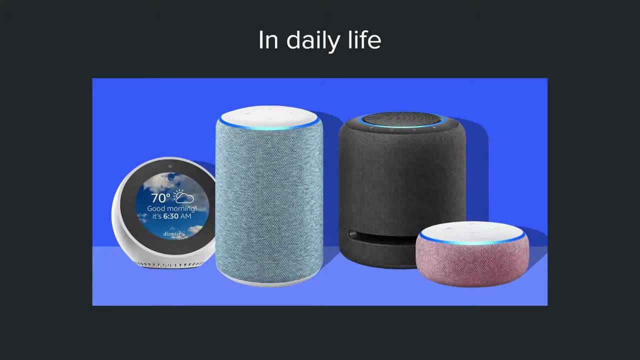 of computational resources and is host on like a really big corpus of data. So we improve language models and more data. machine translation is gradually, gradually getting better. Okay, Traces of NLP in your everyday life can be found everywhere. So from smart home accessory to automate answering service. 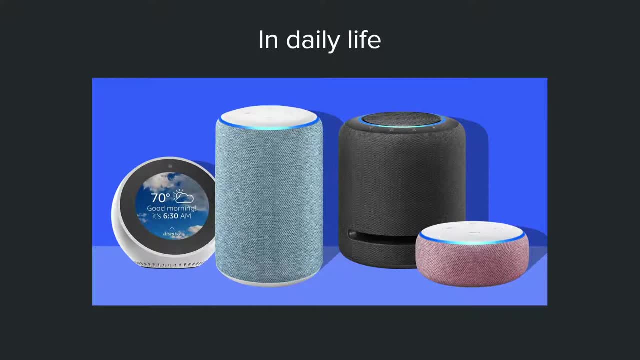 So if you call the bank and you hear like a bot answering your question and like hearing to what you have to say, redirecting you to correct people, that's an application of NLP. So, even like for Siri inside your pocket phone or something like that, NLP has been powering. 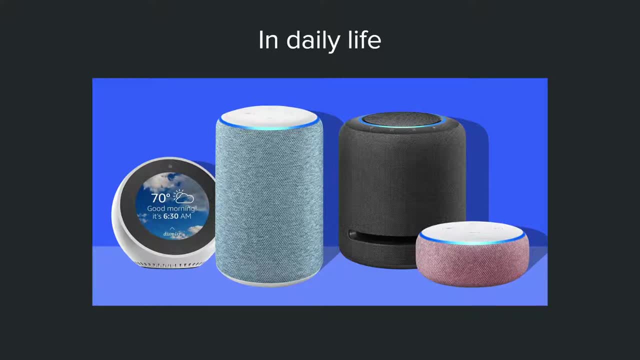 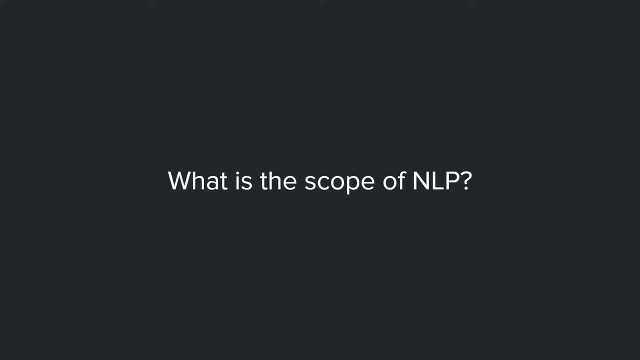 like many aspects And like many technology corporations, consider NLP development a priority. So the field of NLP is not typically defined into subfields, but rather that NLP tasks that address some of the goals of NLP. So that's how the scope of NLP is defined. 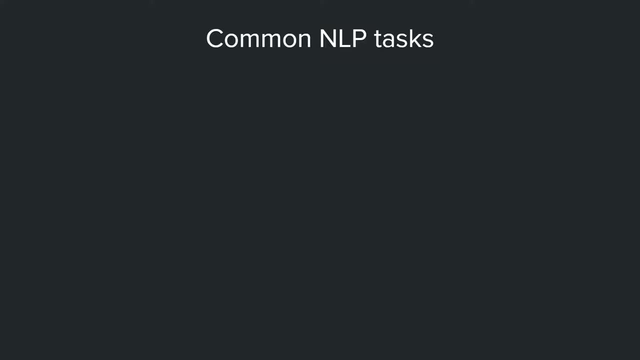 Some NLP tasks have direct real world applications, while others serve as like sub tasks that are used to it. So for example, in solving larger tasks in NLP. So in NLP we typically have like tasks that are basically to end goal of NLP but we address 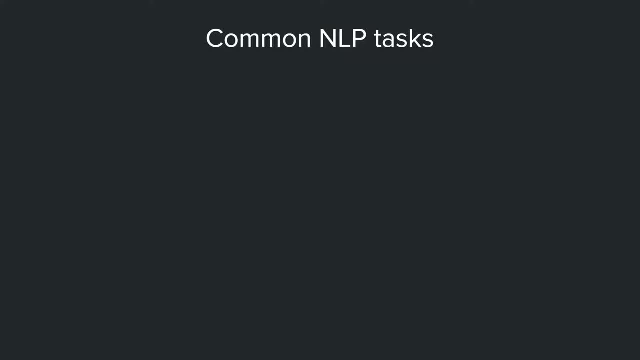 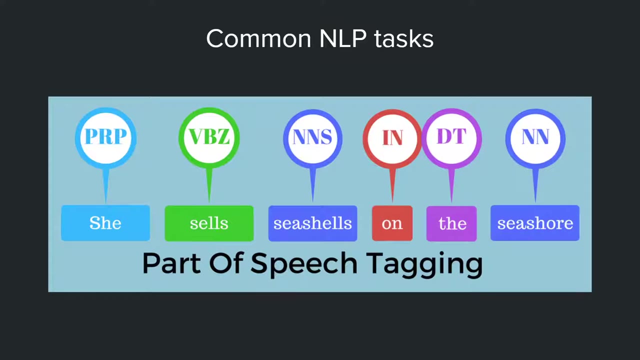 try to address these big tasks like smaller tasks. So common NLP tasks include post tagging, past part of speech tagging, which is basically just determining which part of a sentence is a noun, a subject, et cetera. We have text summarization. 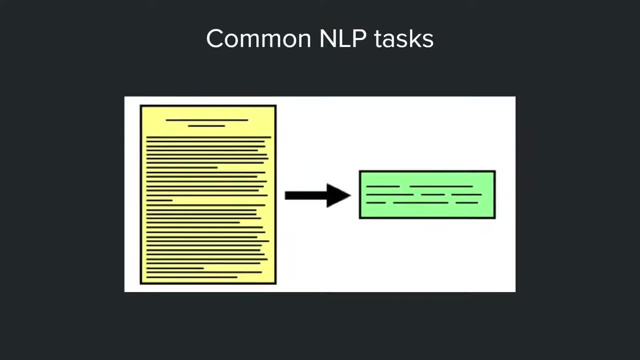 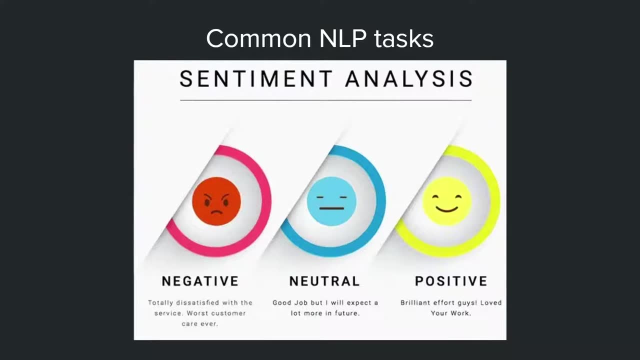 We just basically systematize. Okay, It's summarizing text And it's typically very helpful for providing abstraction of libraries or providing like product description on Amazon for books, of course. And finally, what sentiment analysis? So sentiment analysis is basically identifying the polarity of a piece of text. 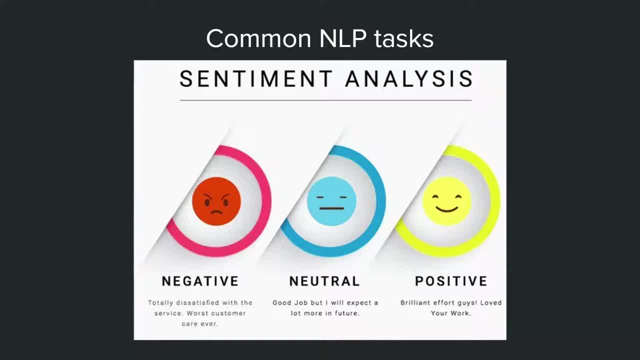 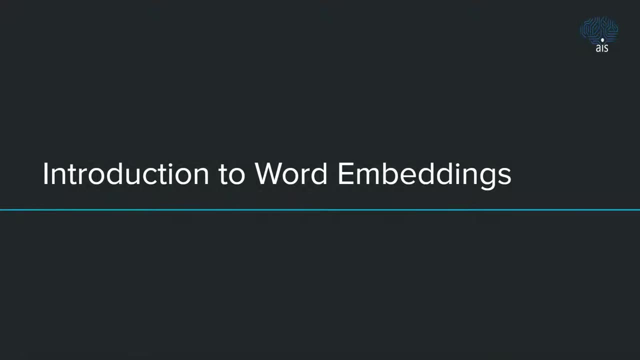 So if you have like a piece of text right, You want to know if it's negative, neutral or positive, And it is incredibly useful. It's very useful for identifying public trends and for product marketing. Okay, So now that we have taken a look at like an a broad overview of NLP, we will start to 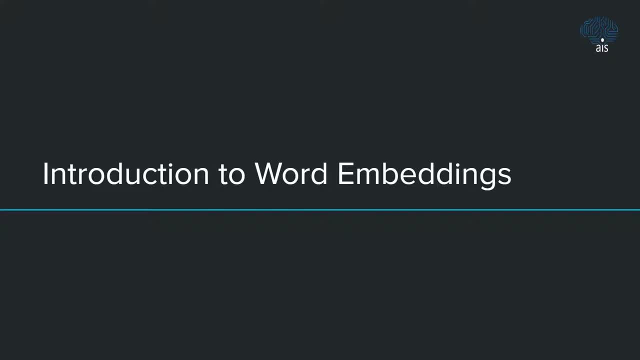 look at something that most of you guys are going to take a look at like the main focus of today's workshop is like an introduction to word embeddings. All right, So word embeddings is like kind of like an abstract term. It's like an abstract term. 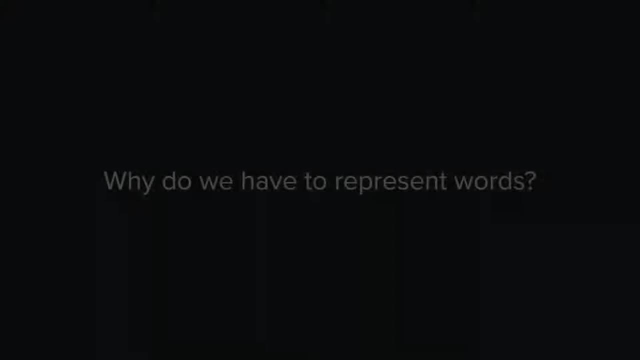 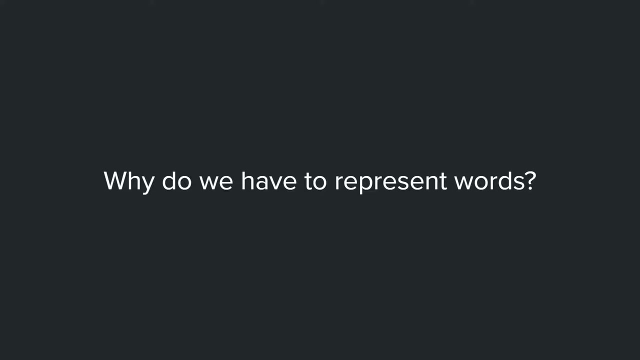 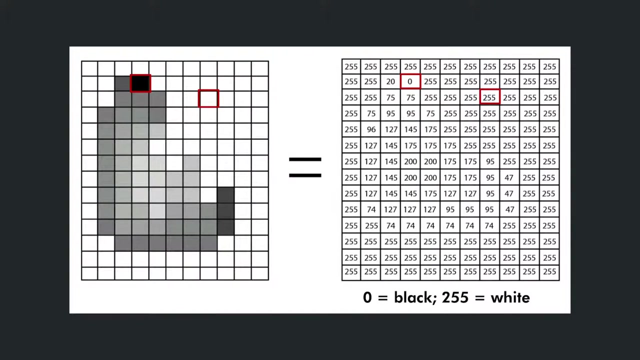 Okay, So it's a form of word representation. So the first question is: why do we even have to represent words, right? What's the point then? So why image data can be effectively and efficiently represented by pixel values. So if you have an image, you can just decompose them and like have every single pixel on the 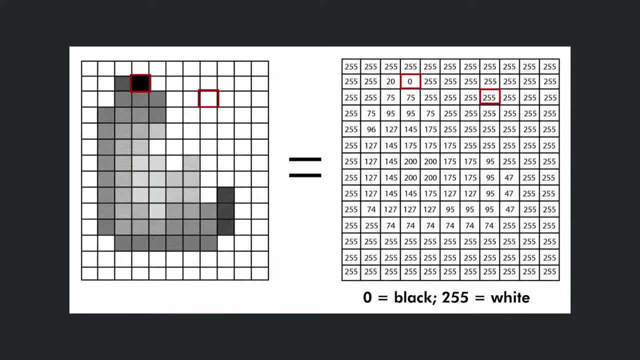 image being like a value, like an integer right, Or a set of three integers Uh, And then you can just convert the RGB values of that pixel before um takes uh for text information. It's not like capturing the meaning of the body of text, like an essay or a book, right? 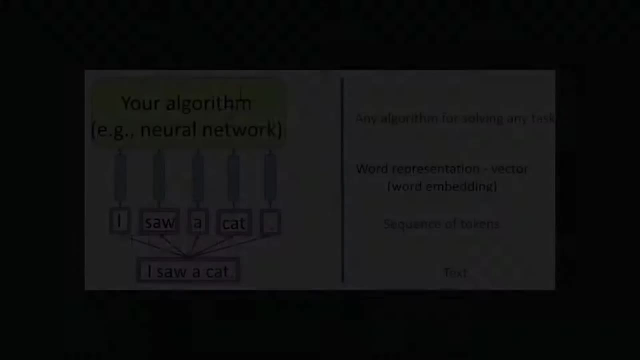 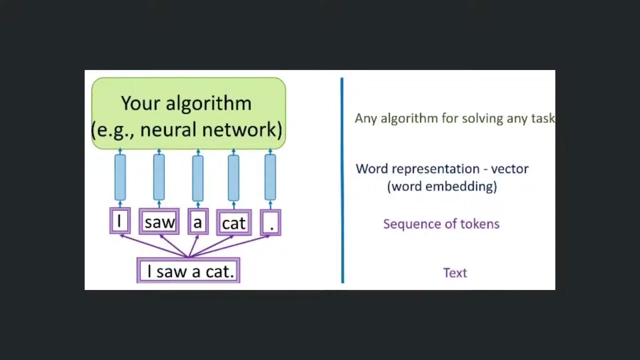 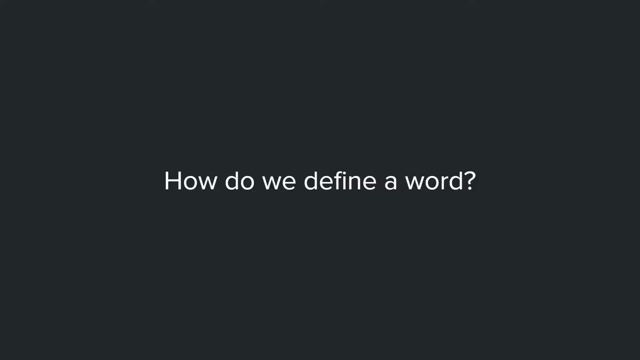 It's not that simple. So, therefore, we'll find a way to represent the meaning of a text body, starting from representing the meaning of individual words. Uh, then, how do we represent the meaning of a word, or, in other words, define a word? 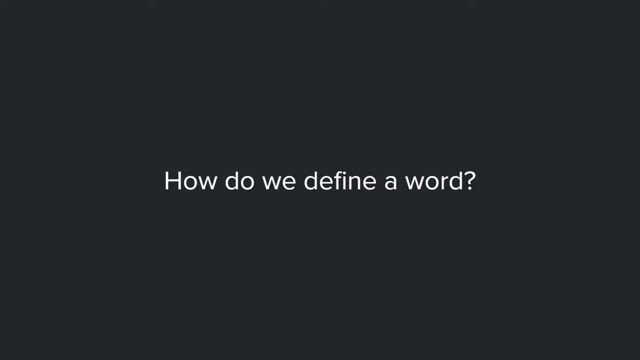 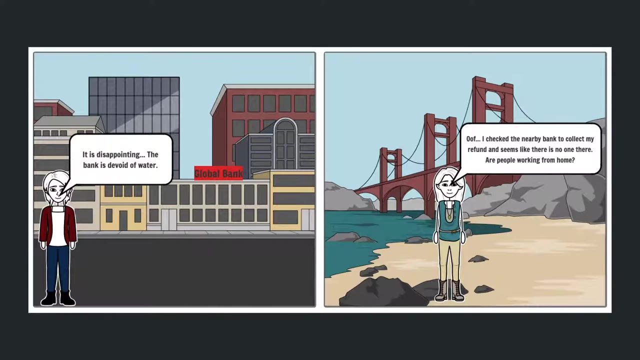 Okay, So the meaning of a word can be defined in a very practical way, which is it's real world usage context, or how we understand a word in our newspaper, in our conversations. So in this case we can see that word bank has two different meanings. 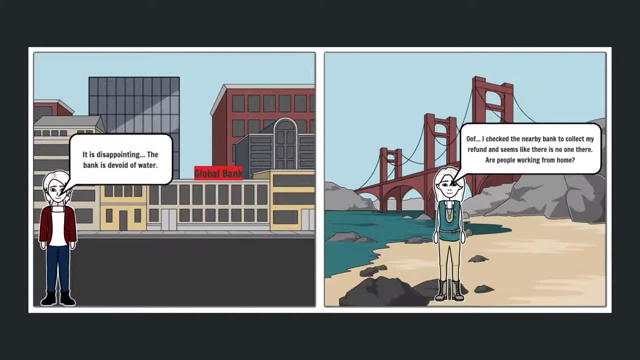 One is talking about a financial institution and the other is talking about a geographical feature- Uh, in this case, we can see that word bank, Uh Uh, different situations in two different contexts, and that's how we define the word, and so one natural consequence of that is that words that occurs in similar contexts tend to have similar. 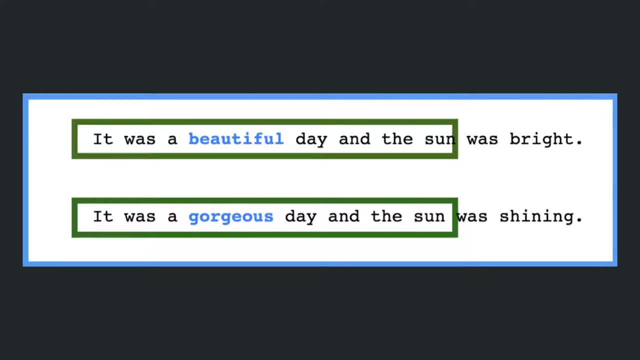 meanings. so, and also over time, the usage context of work can change and so right is meaning a word that's really popular nowadays and we don't really know the meaning. we haven't have a clear meaning to that word. like 10 years, 10 years ago, right, this suddenly became a word that kind of like. 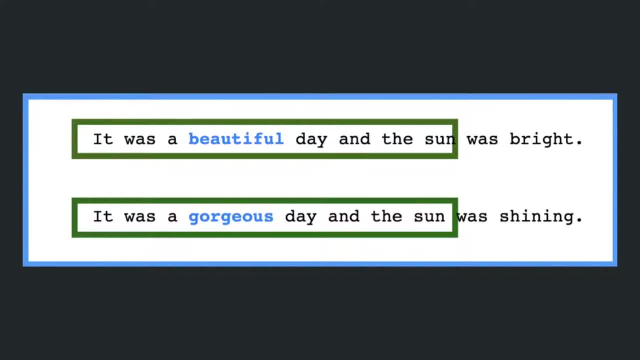 define how you just throw something, maybe quite a bit finally, or even throwing something like it doesn't need to be an object, it can be your classes. and so the current best model for kind of like um defining the semantic of this word and can effectively deal with these kind of word meanings, we call them the vector semantics model. 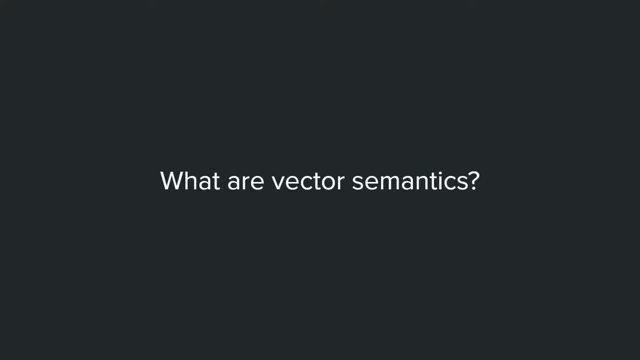 so what are vector semantics? so spectra semantics is a practical way to represent words based on the real world usage context. better semantic is like a combination of two intuition, the first one being the distributionalist intuition, a method of defining a word by counting what other words occur in its environment, in this context, like around it. 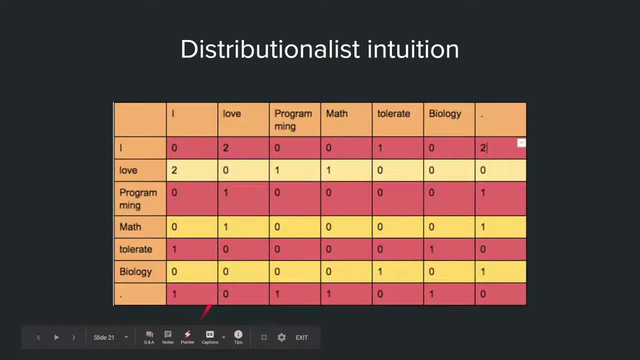 in this instance, right um is our pointer here we can see that word love here. oh, the word love here frequently occurs. neither work, i is like two times, like almost the highest number in in table. and so that's our distributionalist intuition. the second intuition is the vector. 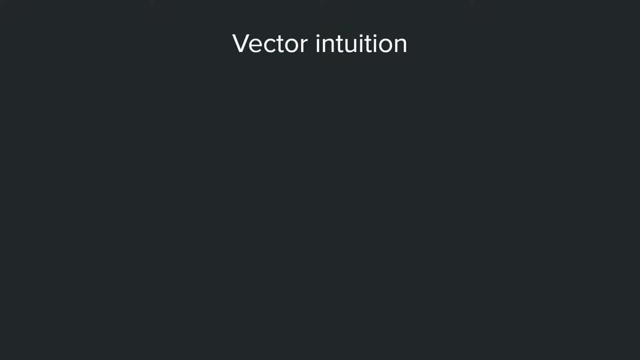 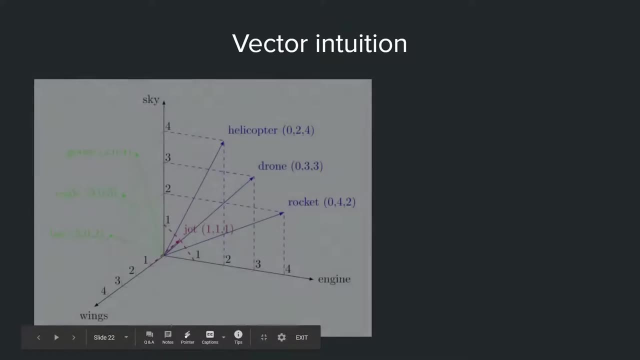 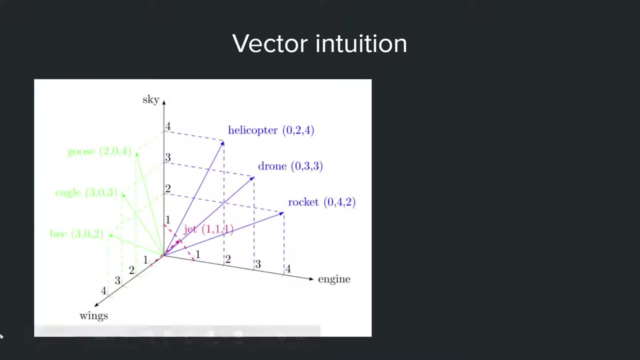 intuition, in which we define the meaning of a word as a vectors, a list of numbers and a point in n dimensional space, um. so this might sound a bit abstract, so i just take a very specific example. here we have a wood rocket, right? so we, here we have a wood rocket, which is defined by 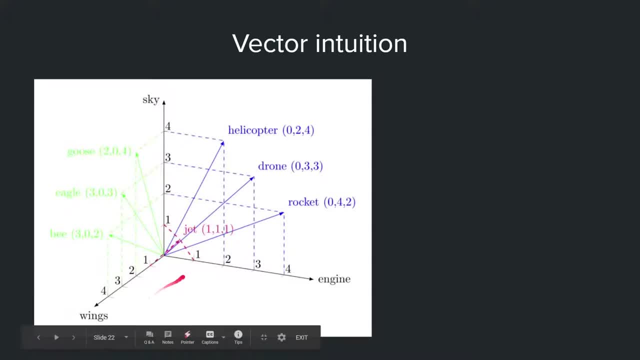 three attributes. uh, the first one is the wings. so it doesn't have wings, so i will say that it has zero wings. uh, skies, it's kind of like, okay, it's rockets are in the sky and you're supposed to find it. so it has a lot of sky. we have four sky for it. so we have four here and for engines. 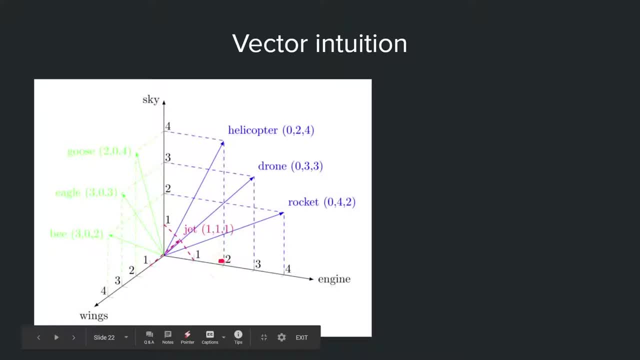 the rocket basically just powered by engines. so we have two of them here. it's defined by two of engine and that is what we call embeddings vectors for representing words, because the word is embed in a particular vector space. what with similar meanings tend to be really close to each other in the vector space. so we can see. 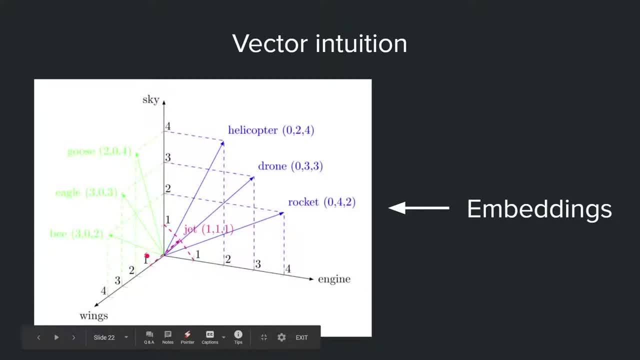 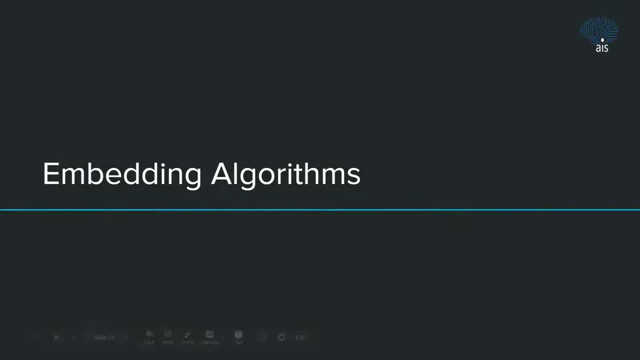 that what are like kind of similar right so drones already in the same domains with rockets- a really close rocket here. so now that we have our vectors, how do we create them? we move on to learning about embeddings algorithms. the fundamental ideas being behind embeddings is representations of word similarity. so how can we represent word similarity? 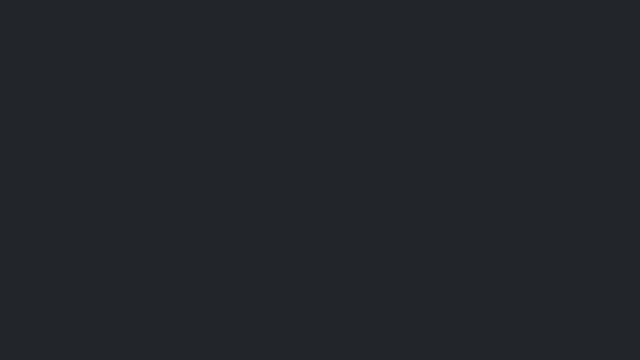 because we define each word by the context around it. we need a recurrent of of the context of each word, right, we need to know what kind of words occurs around the word that we are looking at, and so we have something that do just that, called to call occurrence metrics. 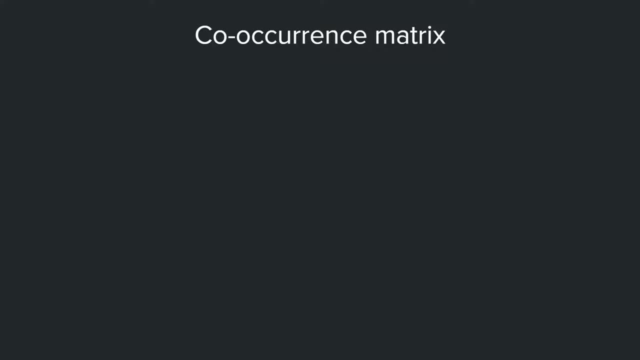 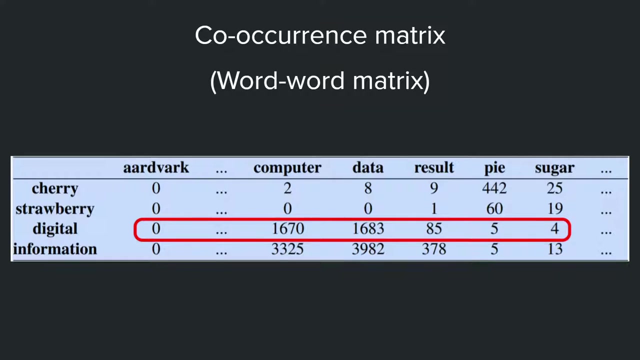 the kind that the particular types of co-occurrence metrics that we care about today is the word, word matrix, which we cut, which recurs the frequency that two words are in the same context in some training corpus, so the context of that training corpus of that word can be as large as the entire document. so you have: it occurs in the same document in the. 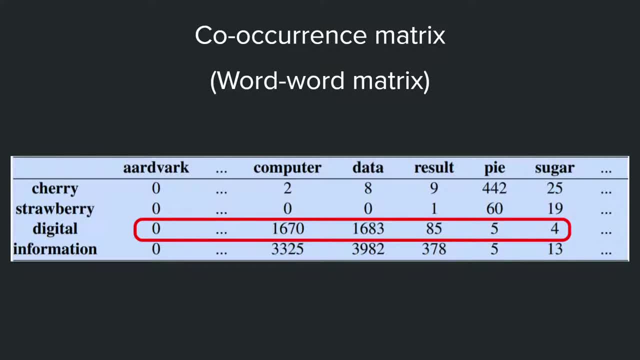 same story, right, or in the same book or, more commonly used, would be like a certain window around the word itself. so for example, like two, two words before word or two words afterwards, and we take that, that windows out to be the context. so here are the co-occurrence factors for forward in the wikipedia corpus. 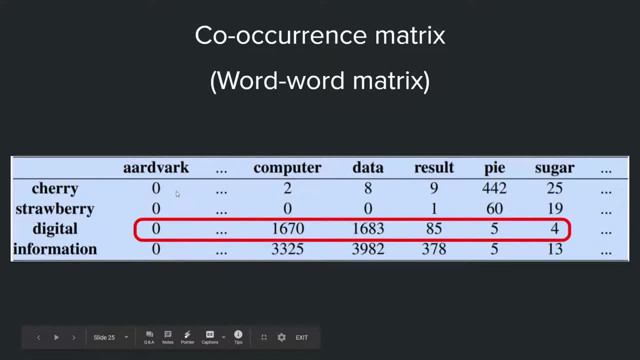 we can pick dimensions um, so in reality it's even not going to look as nice as this. we just picked like this dimension because these are like what we want to demonstrate here. so note here that the word digital is really high into, into other words, computers and data right and 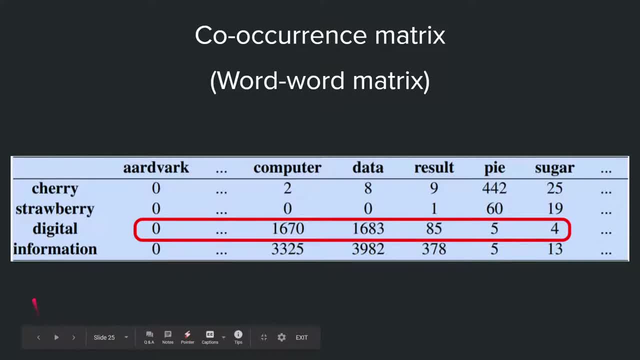 we can see that we have like a really closely related word to digital um, as you may know, um. so note that the real factors we have many dimensions because we're comparing each word to every single other word, we're counting them to every single other word in the vocabularies. so how many words? 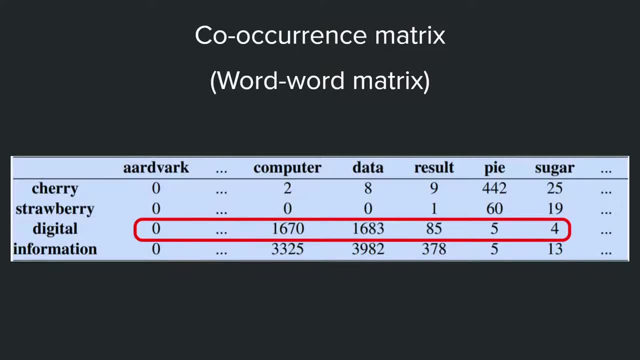 you have in the like the number of words that you have in the vocabulary of training corpus. we have that many vector dimensions, right? so imagine we have like ten thousand of them. we have ten thousand of our dimensions, not like six on the data, but we take a look at that layer. so now that we we can 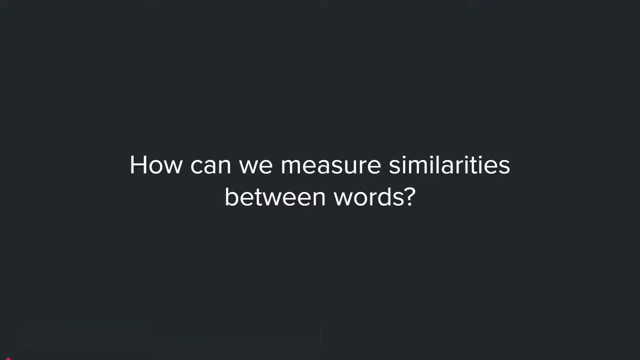 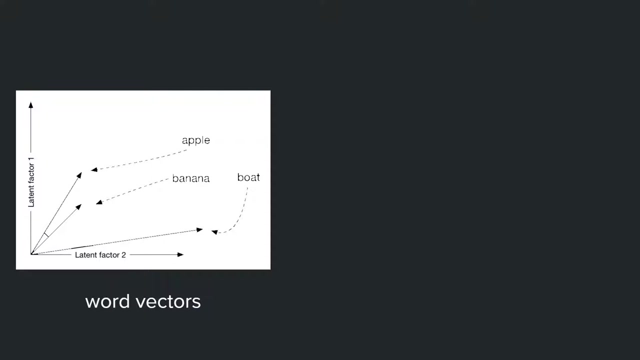 represent what similarities? how can we measure the degree of similarity between two words for our embedded purposes? uh, so, to define the similarity between two words, we need a way to take the two word vectors, which which were generated by the matrices that we just take a look at and calculate. 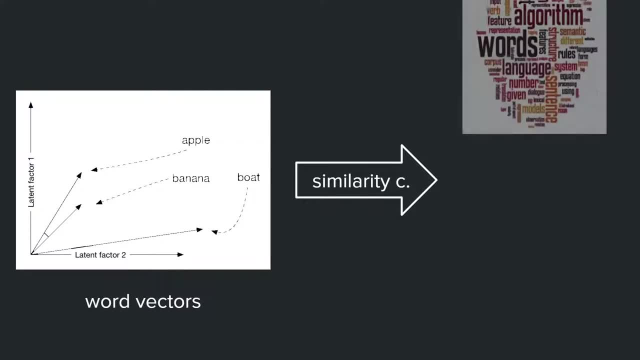 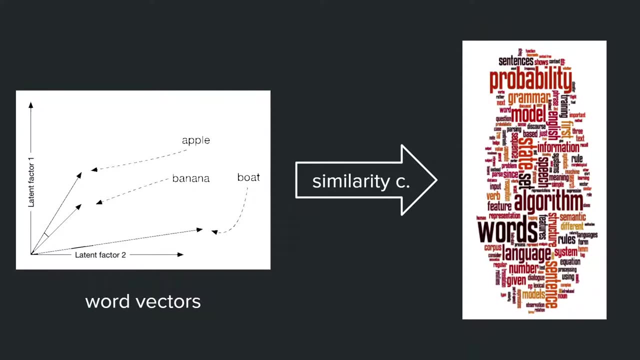 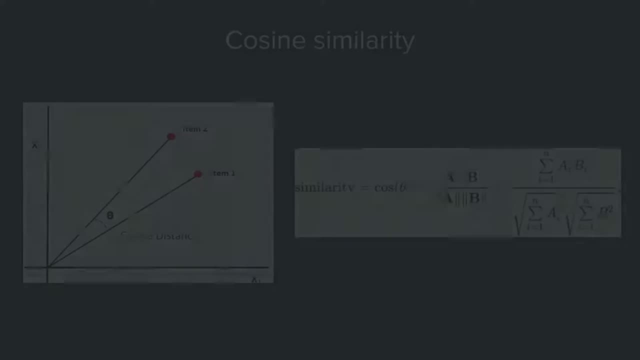 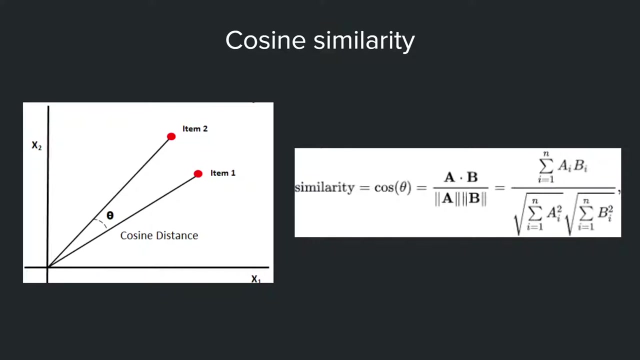 our vector size. so let's take a look at some of the different videos we can use to create this able, and these are the measures of similarity based on these vectors. so when we talk about similarity between two vectors right, one that naturally comes to our mind is the cosine of the angle between them. so it is a variation of another similarity measures, that's. 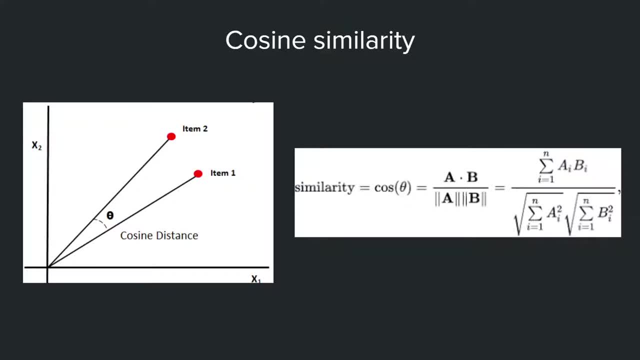 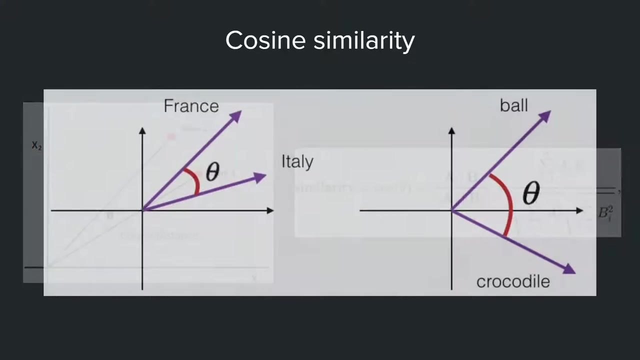 very typically using nrp. this probably kind of sounds familiar to you, um, but like, yeah, so what we see here is the formulas to calculating the cosine between the n, the cosine of the angle between two world vectors, and that still seem a bit abstract, so i present here a more intuitive example. uh, so we can see that. 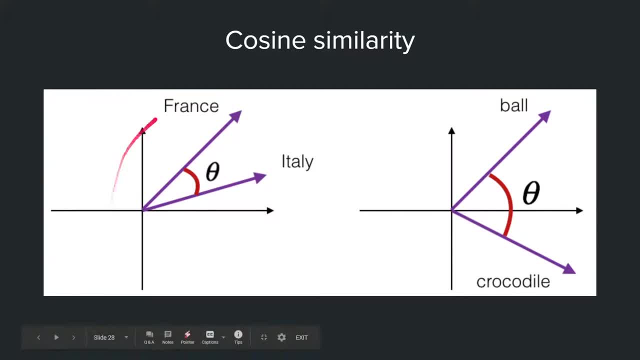 the world factor frames and the word rate of italy here are like quite similar, right, so the angle between them are really close to zero and the cosine is like close to one, naturally, but like, on the other hand, we have to affect the ball and crocodile, which is like not similar, obviously, and 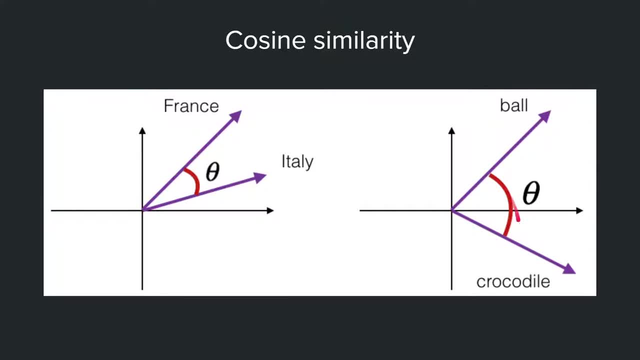 uh, they are. they are like they're having a, an angle that's like close to 90 degree and thus, uh, the cosine is like close to zero. so the part that we can see here is that, like to more closely, like the more closely related these two vectors, right, the smaller angle between them and the smaller. 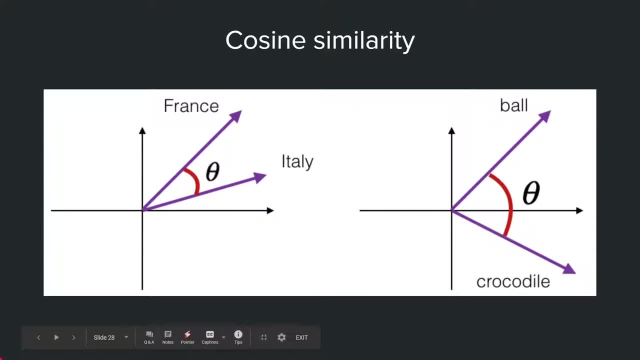 view and the symbolic angle between them. the smaller the cosine values, so well. cosine values typically range from zero to one. they cannot go from below zero, since our world frequency is not negative, and we can see that the higher the cosine values, the more similar the words are. 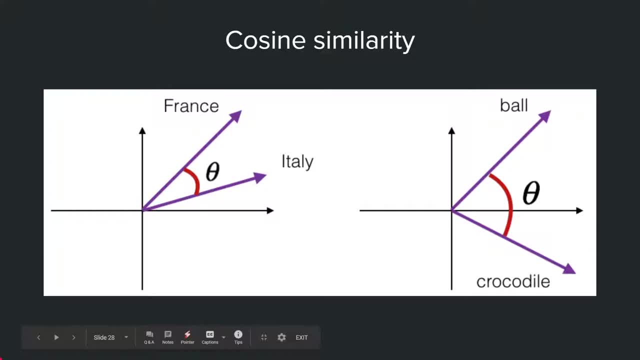 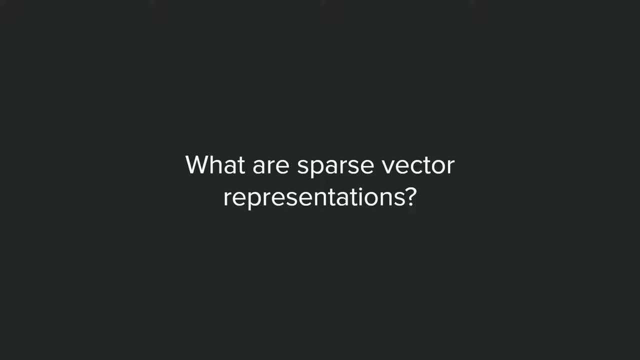 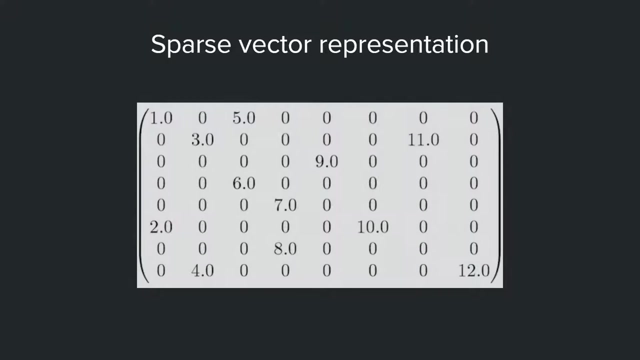 so we already have here a similarity measure. uh, okay, so now that the kind of world vectors we've been looking at are some examples of sparse word factor representations, so what exactly are sparse factor representations? a typical co-occurrence matrix looks like something like this: right? 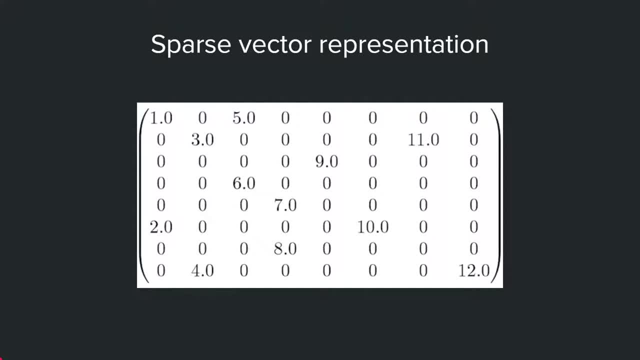 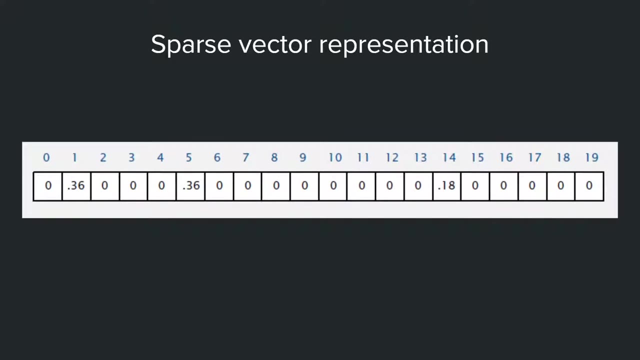 with most entries being zeros, since each word can co-occur within a few number of other words in the entire vocabularies. so, and as a result, um, a typical world factor extract for the matrix will looks like this, which is kind of gross because you can see that the vector is really big. 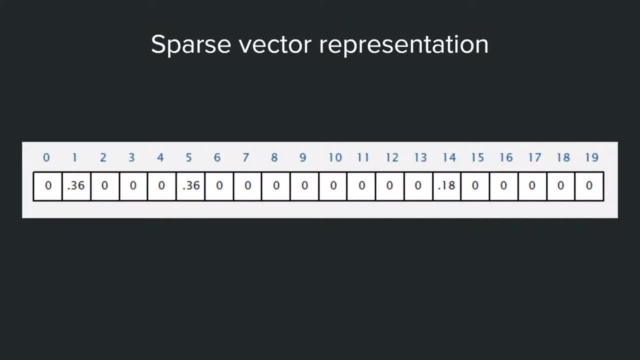 right but non-zero. elements are few and far between and sparse representations are pounding down values. for this very reason they increase the verb-factor- Dafna two with saving and increasing it. in daily hind구 bullets going along, new elements and sparse representations are troublesome for this very reasons. 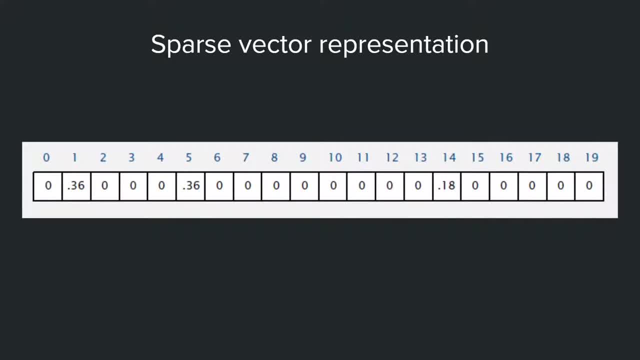 Sparse representations are troublesome for this very reasons. they increase the feature space of the machine learning model and ultimately increase the model complexity and chance of overfitting. and trust me, if you have been like in machine learning for a while, you don't like overfitting. 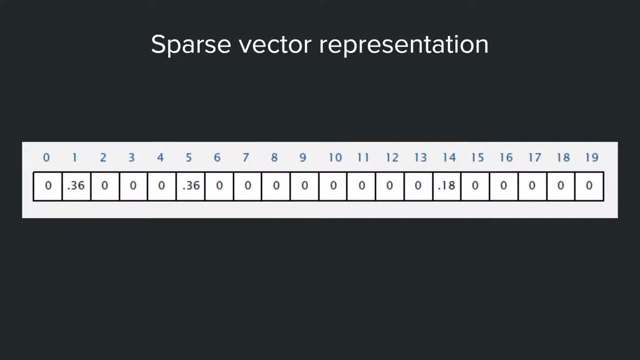 even when you start out you really don't like overfitting and, more importantly, sparse, vector may leave out important word meaning informations, remember. another goal for us- to represent word as word embedding is to capture the informations, like the immediate informations of the word itself. so consider the case of one hot. 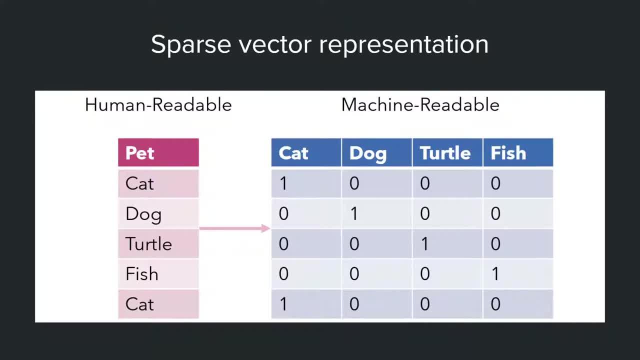 encoding where each word vector is positive on the worst unique index in the vocab, in the entire vocabularies. so here we have like, so we have like each word, right, we are encoded with like a single vector, like a single values are vectors. so for example, cat is a vector one, zero, zero, zero. 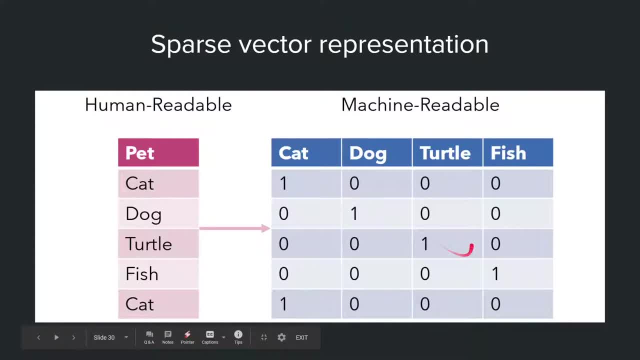 uh, dog is a vector zero. i'm sorry, my pointer is switching out. dog is the vector zero one. oh, oh, so you can see here that each word is encoded by an unique way, but it gives absolutely no informations on how the word cat might be related to dog or any other animals. right, because all you know is: oh, it exists as a thing. 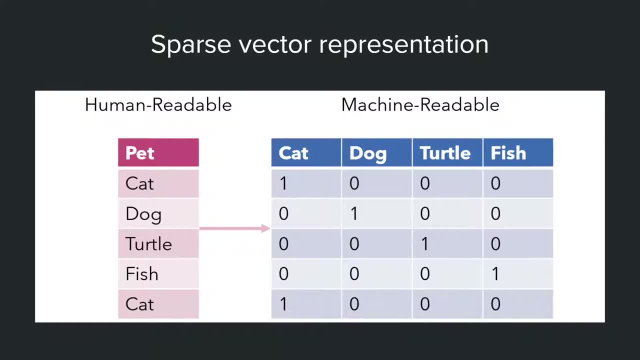 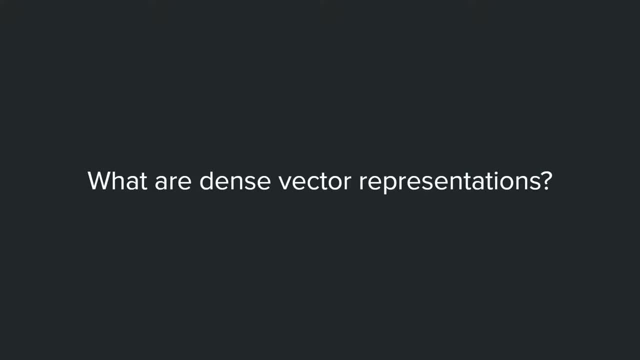 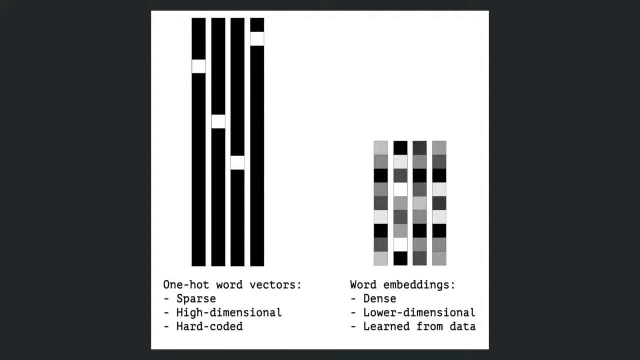 but how, how it is related to others, right? okay, now that we have learned about the limitations of sparse representations, we move on to take a look at dense vector representations. yeah, it's opposite of sparse representation. dense vector representations is a form of representations that relies on short vectors. 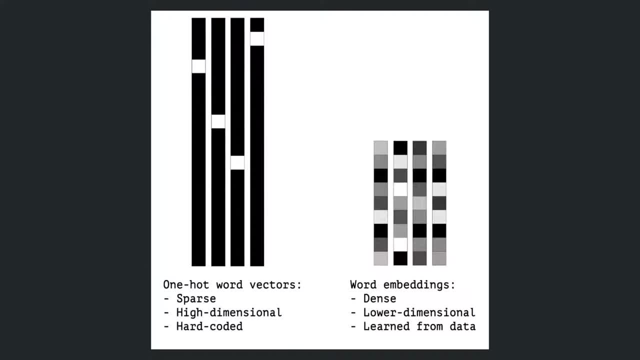 so it's like 50 to a thousand unit long. that's what we define, what we call short, because the long, sparse vectors are like thousands, like like a couple dozen thousands um in this wrong right. so that's way longer and they're also really dense vectors. so most values in uh in vectors are non-zero vectors. 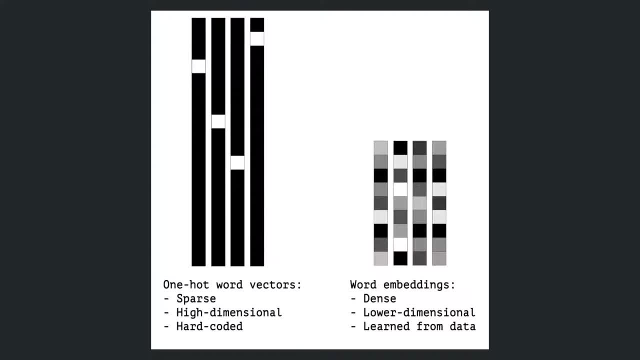 meaningful values. so, more than merely condensing meaningful word similarity, information, dense representation can be learned directly from text, and that's what we really care about. we can learn this kind of word meaning: um, yeah, so, yeah, so, if, yeah, that's correct, if the angle is zero, two minutes are really similar and 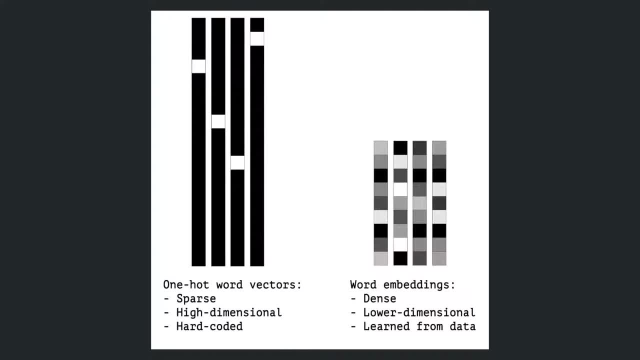 the cosine? uh, then would be one. you got it. um so, let's go, let's continue. um so, dense representations can learn this semantic information directly from text, right, and it can represent them in the form of closely related low dimensional vectors. so that's what we're going to talk about in this. 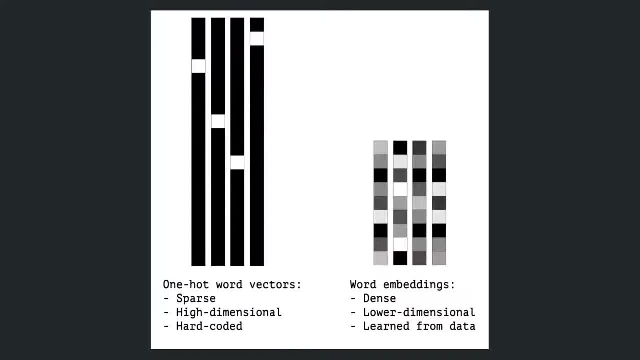 video. so let's move on to the next part of the presentation, and we're going to talk about how we can learn this semantic information directly from text. right, and it can represent them in the form of one really popular one, very, very popular dense representations method is called word2vec package. 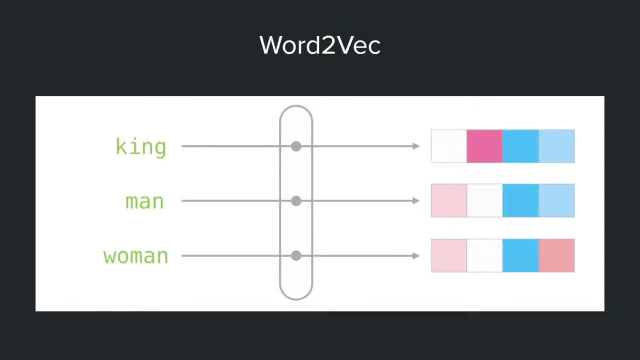 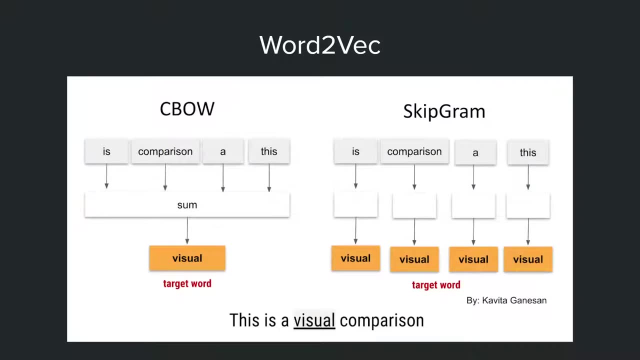 you've probably heard that before if you um read some stuff about nlp, and it is a package of embedding algorithms containing two embedding algorithms called the continuous bug of work and the skip ground method, and today we'll take a look closer, look at like the skip ground negative sampling method. it's very it has a very fancy name. 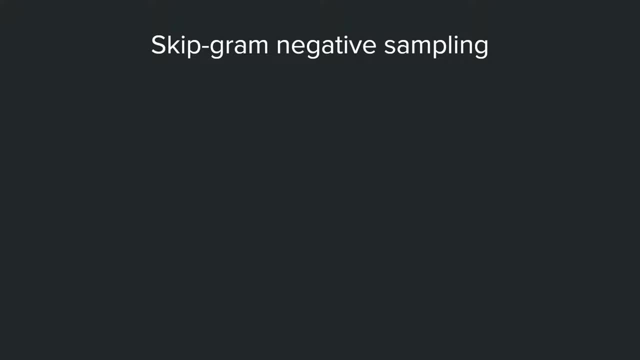 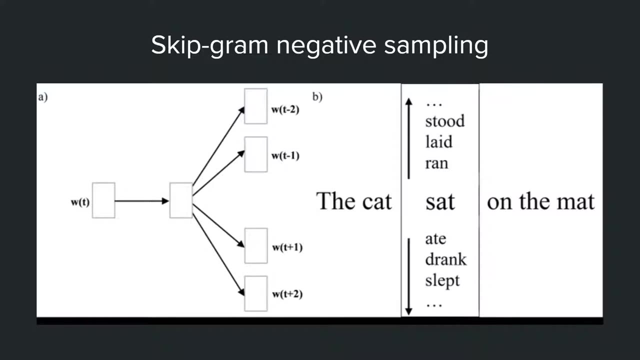 so the intuitions of word2vec is that we train a binary classifier to predict if sat is likely to show up near cat um. the classifier is incredibly simple to train because we can just have the surrounding text as the training conference um in this sentence, right in particular, if you want. 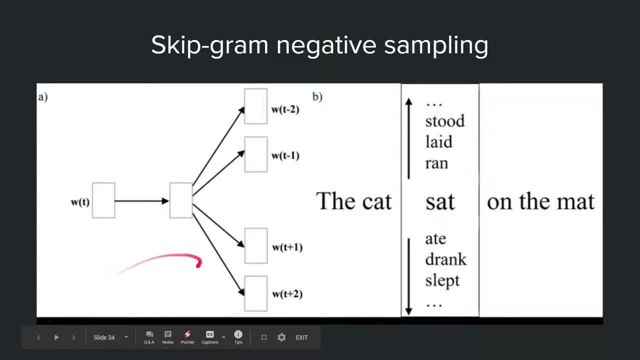 to take, like if you want to take um, the training example for cat, you can just take the word near it here, like sat and t as the supervised classifier model label as positive sample right and we can use that in the supervised learning algorithms. and so the intuitions of skip gram is. 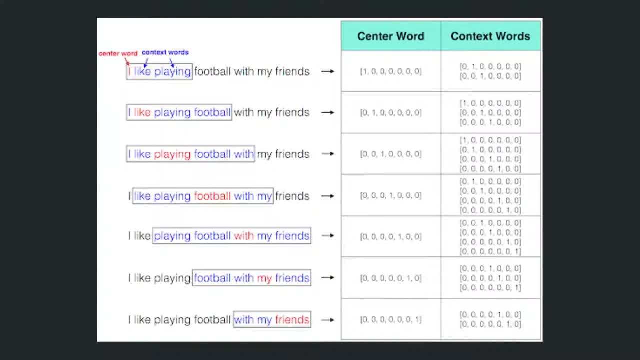 first we treat the target word and the neighboring context word as positive samples. other words in a lexicon are randomly sampled to get negative sample right. um, in other words, you just take everything out of the word that we have not seen yet in our process sample as negative sample and we can just take them from the, from the vocabulary. 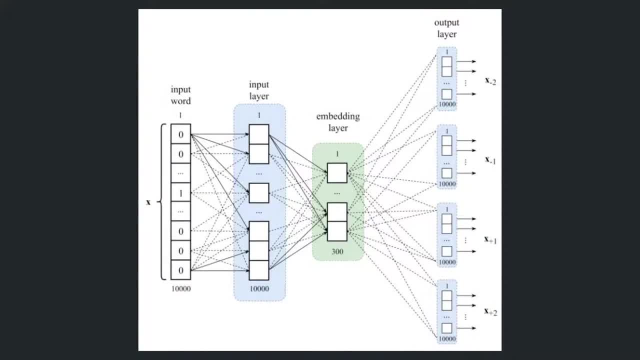 and then we use logistic regressions to train a classifier to distinguish these two cases. and finally we use the hidden layers, regression weight, also called here the embedding layers, with as word embeddings. so you can see, here in the network it's embedding layer, here that we will take as our final word: risk representation. 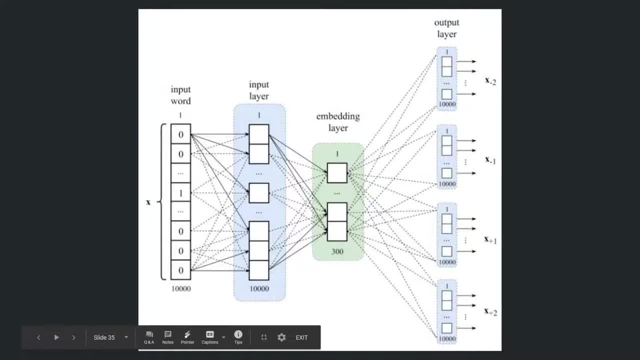 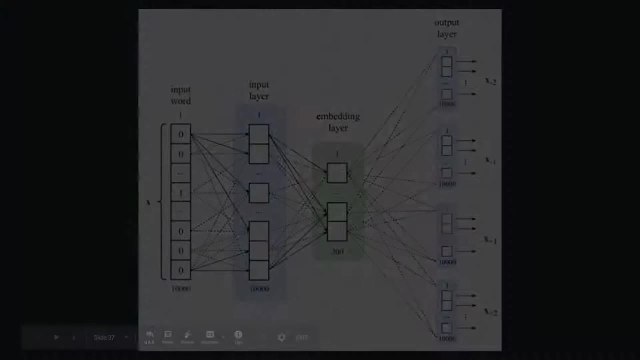 okay. so now that we know the intuitions of this uh, of skip gram, uh, we actually just jump straight into like coding it right now. so i'm hope, like everyone, prepared for some coding right today. um. so okay, uh, excuse me, i just- oh, sorry, it's spoiler- um. 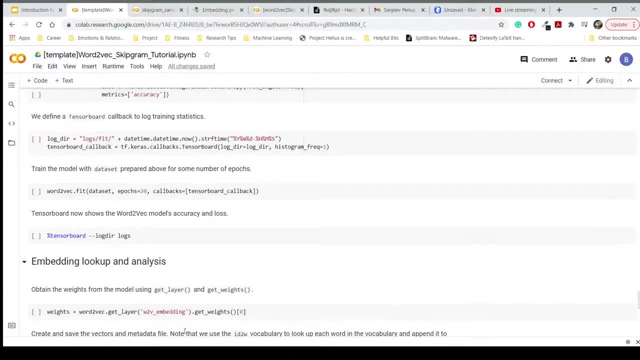 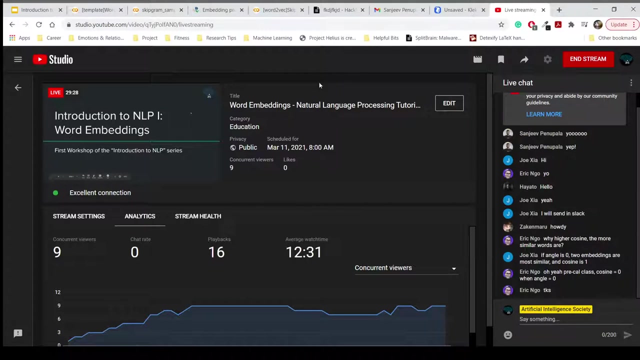 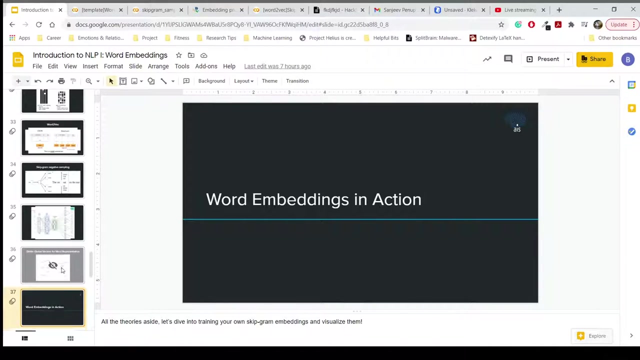 uh, i post, uh, the link to the coding template here so everyone can take a look at it. why is my camera on? okay, that's. that's a bit weird, because every time i try to go to the borders of the window, it just glitched the hell out of me. 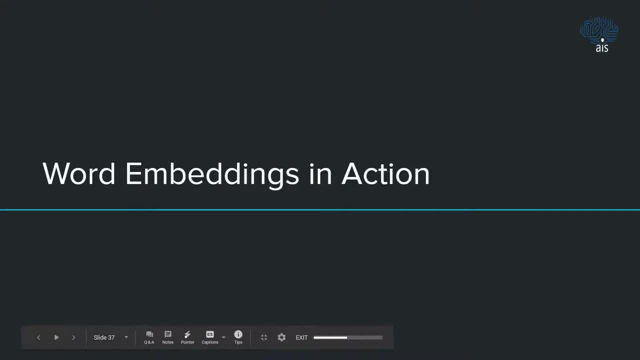 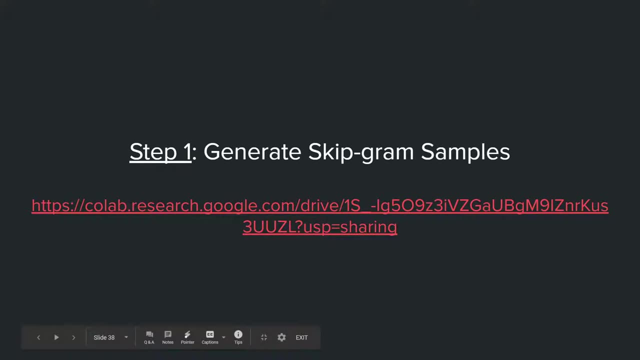 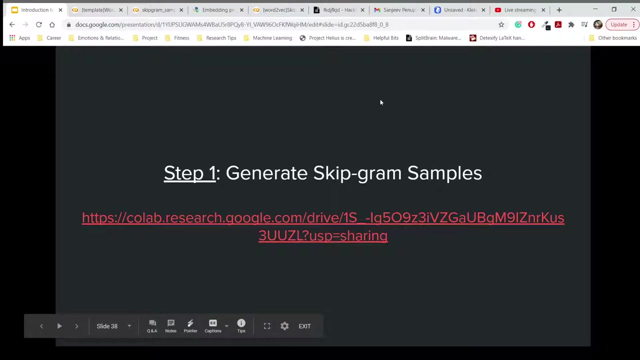 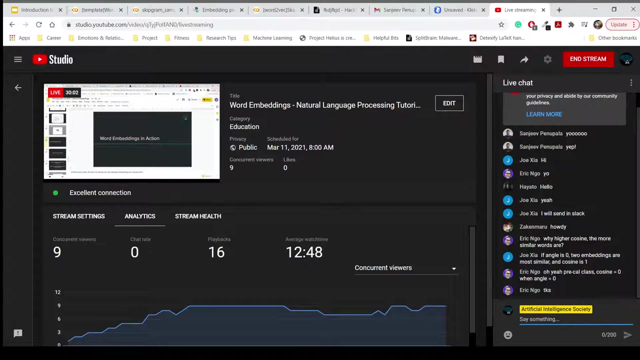 yeah, you see, all right, um, i just have a link here, so i just let me copy it. please let me copy it, okay. copy link address. um, so i just post it in the live chat, okay? um, it is sorry. yeah, so i post, uh, the link to the number on in live chat and we're gonna take a look at it. 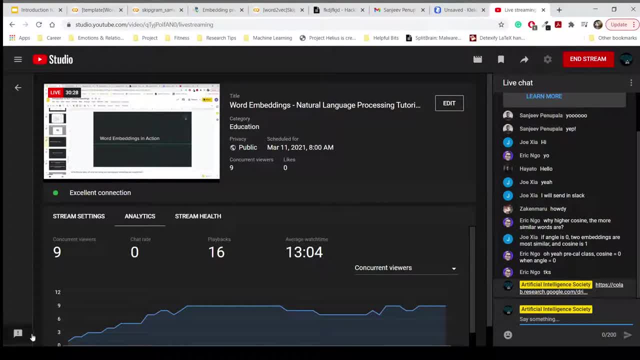 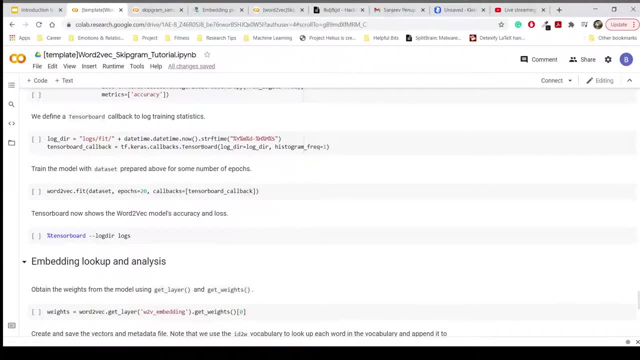 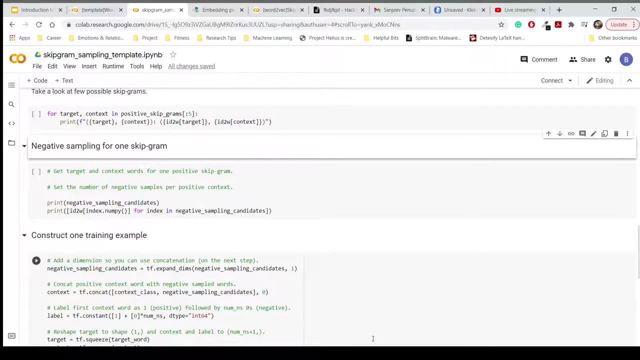 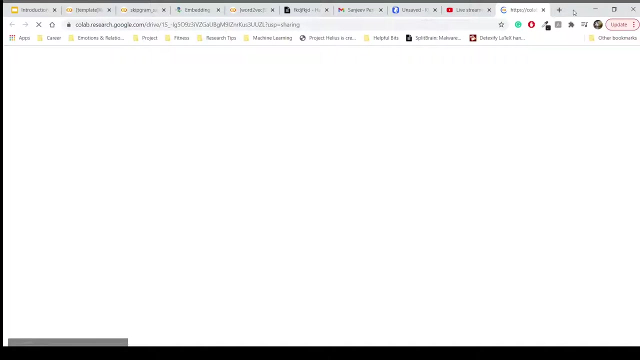 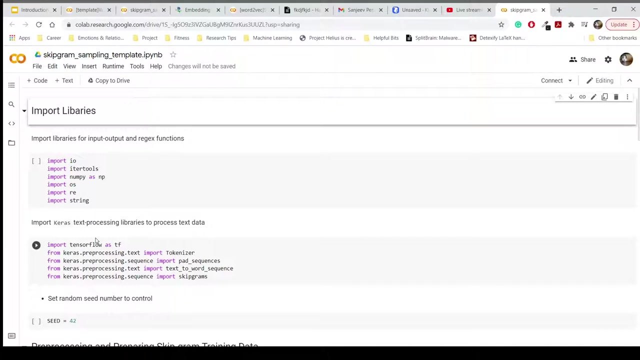 um, okay, yeah, for some reason, my mouse just reaching out and it's kind of annoying. this is my first time streaming on OBS, so I have more problem than this. all right, I open another here. okay, so we are another first step to creating a script voter, to creating a skip wire model. right is that we have to create to training the training data and 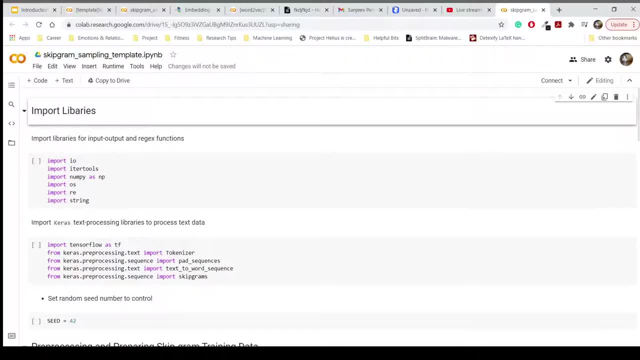 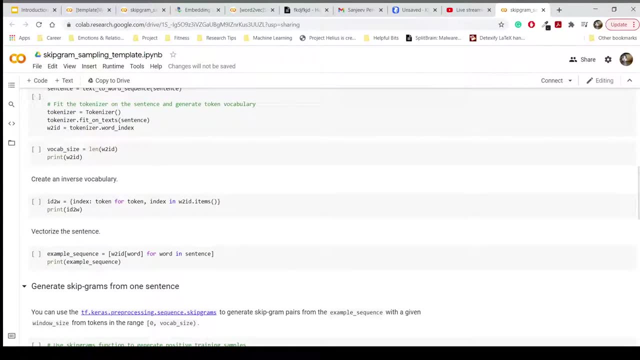 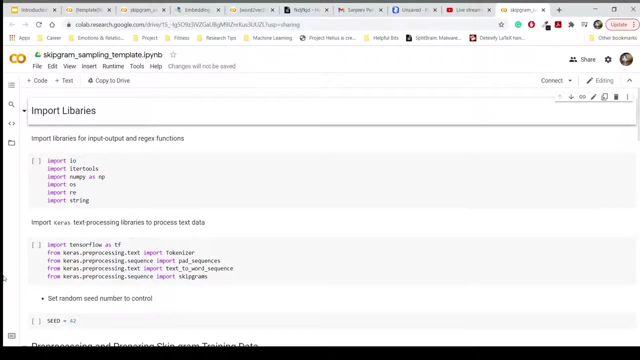 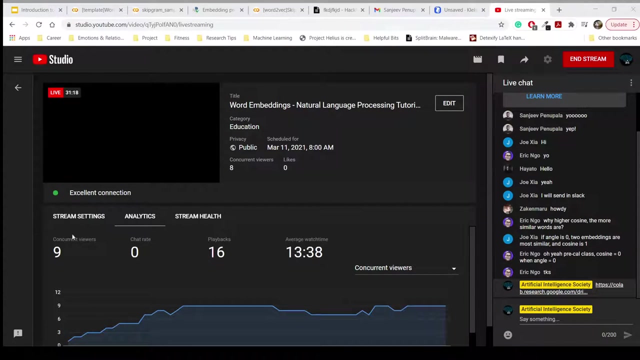 that's what we call theèresia chart, skip gram sampling method, and so here we have like a notebook. here i have like a notebook. uh, for everyone it's like template notebook, so we can take a look at that. um, i try to provide some intuition on it along the way. um, with this, i'm sorry. 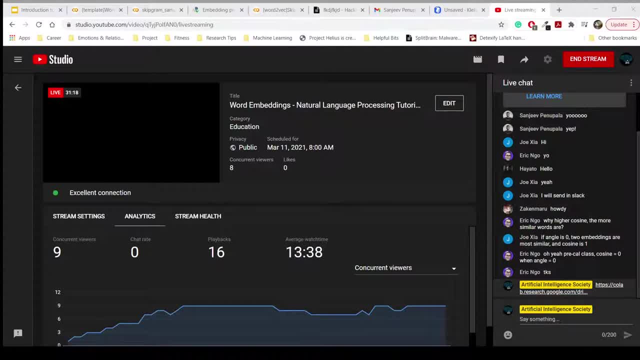 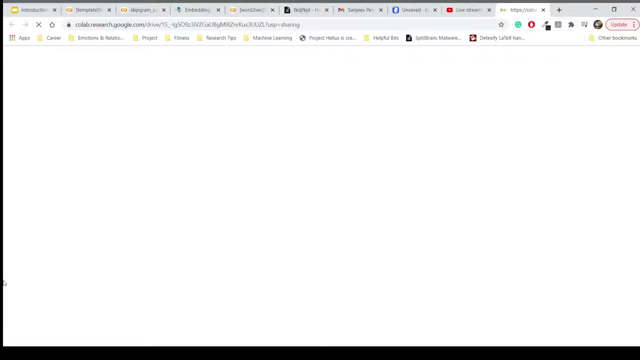 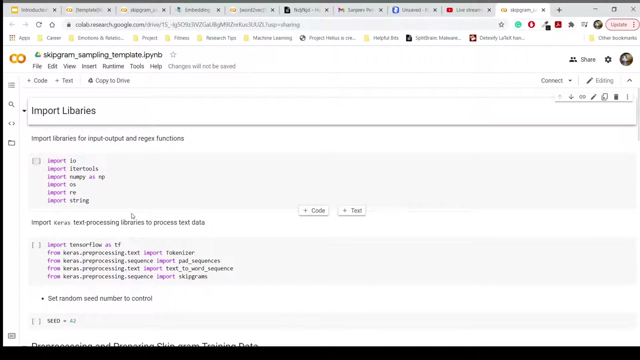 okay, that's actually annoying. next time this corner is ready, you will be something. okay, all right, okay, um, so the first step: if everyone's already uhi got video, uh, have the notebooks up. uh, yeah, let's open it. um, okay, so we connect. first thing, first we. 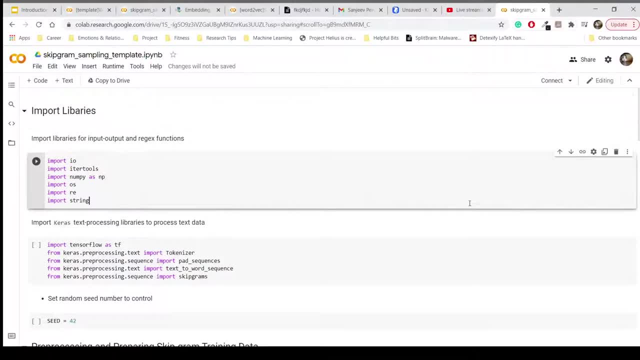 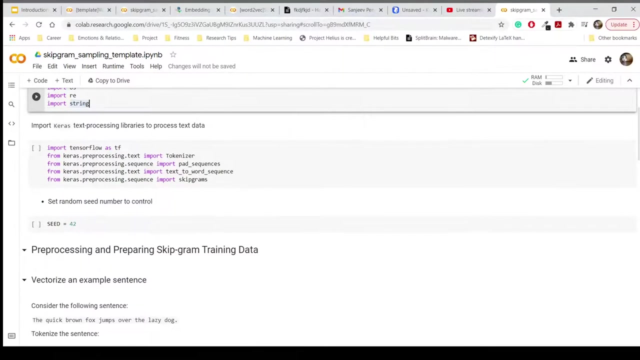 will connect to the server. all right now that our notebook is connecting to a host, we take a look at what kind of libraries do we import for creating the training example. so it is like an isolated notebook from the main notebook where we train the actual two world to break. 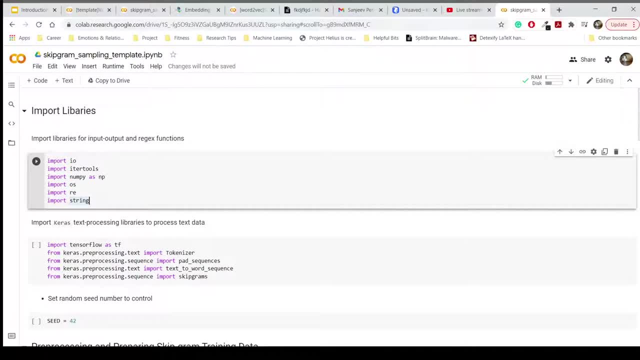 vectors. but, um, here we take a look at how we generate the same training sample first in isolation, so we, you guys, can have a more like intuitive understanding of how it works. uh, all right, so here we import, like io right into two stuff with that really standard stuff. 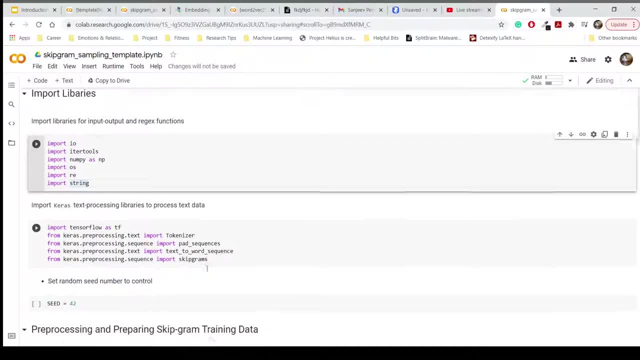 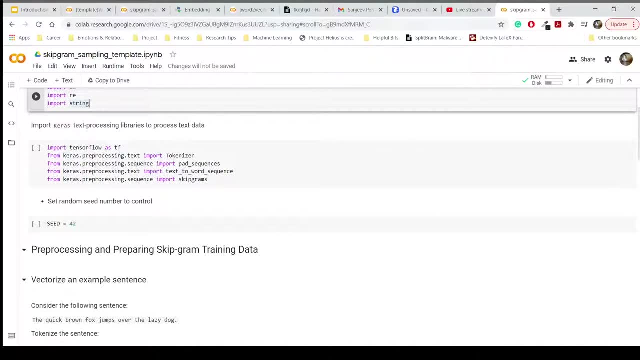 library, standard python library, and then we improve uh, because this workshop we go probably we're going to use tensorflow and one thing that naturally, that just come naturally with tensorflow nowadays is the keras processing libraries. it's a very, very helpful processing libraries, so we improve uh some, we import some of them here to use to uh to use with processing our text. so here we 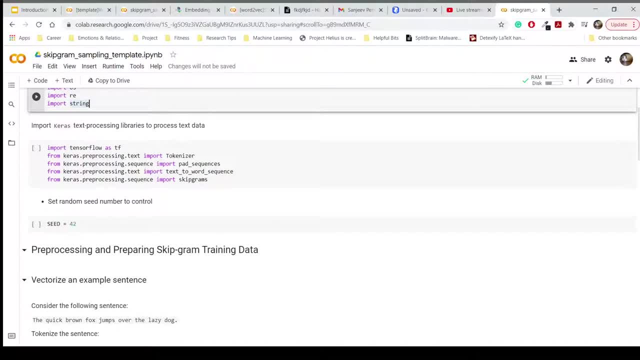 in hot case of our cf, we just have something called tokenizer. we'll see how it works, like why we use it later on. it's a sequence thing, so that we can pass sequences, it's not really necessary text to what sequence and the skip ground itself. i mean we just have a method called super method for generating sample. all right, so the first step. 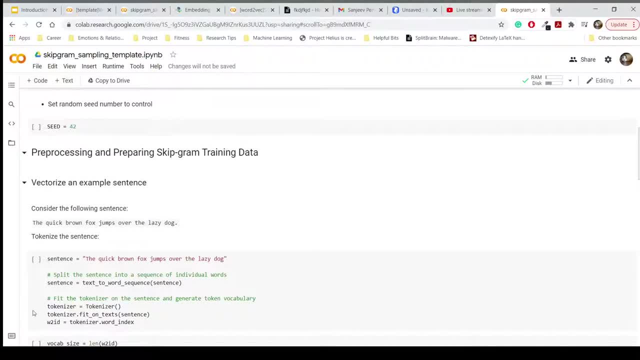 um, we are taking a look at one particular example. example sentence: to quick brown force: the jump's over the lazy dog. everyone probably seen this import something, um, so the first thing we do here is vectorizing the sample to sample sentence: um, i'll try to provide more intuitive music, so i. 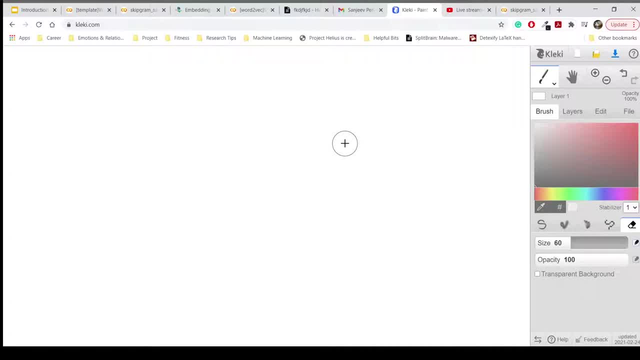 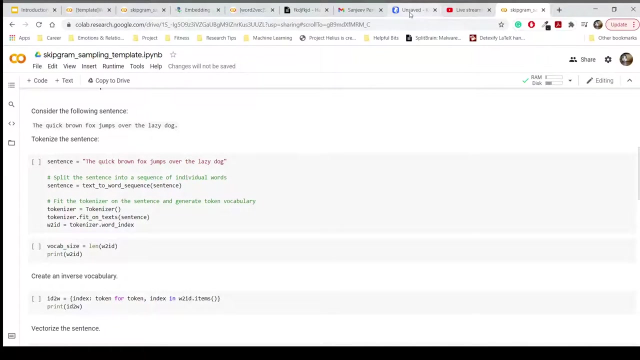 just have this guy up right here, okay. so what we want to do when we vectorize, when we meant, like, what we meant why, by saying that we want to vectorize um a sentence, okay, um, skipping to the quick band, force, jump over this dot, all right. so, for example, i have 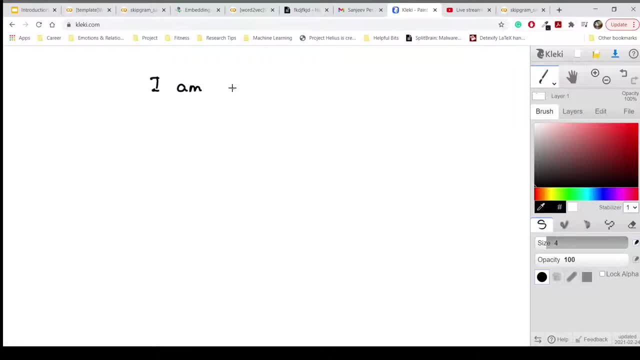 a sentence like i am a cat, right, okay. so if we have a sentence like this, uh, to come here, we're probably not going to understand it by itself. so what we do, the first thing is we vectorize this sentence. vectorizing consists of two steps of kind of like two steps. first thing is we split the sentence. 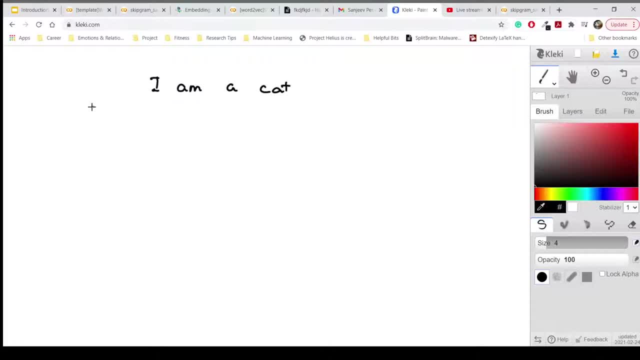 and second is that we tokenize the entire sentence. um, so the first thing, first we do. so what we do here is tokenizing, right. so for this sentence, right, we generate a set of token, and to generate this set of tokens, we need to know what kind of words are in this sentence. 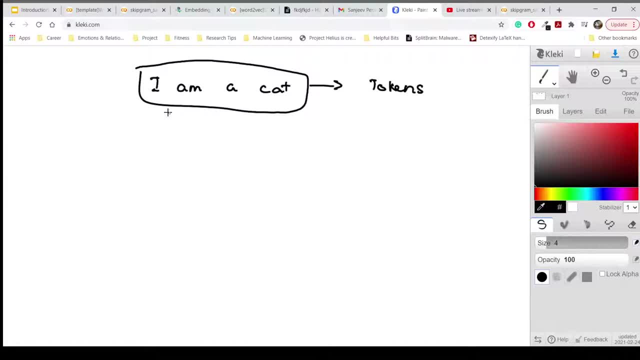 in the first place. so to do this, we just construct a library, uh, a vocabulary, which is basically like something that translates from word to numbers, right? so i will be like one is like hash map and will be like two, uh will be a three and cat will be a four, right? so what we meant by factorizing this is that we take this sentence: 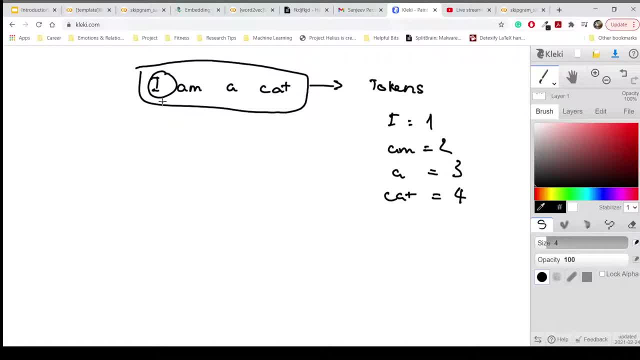 and we split it into tokens, a sequence of token. so we have an array here and i will be 1 and will be 2.. we're just translating it from the vocabulary here that we have. so each entry of this thing, of this vocabulary, will um, will represent, like one item, still one like. 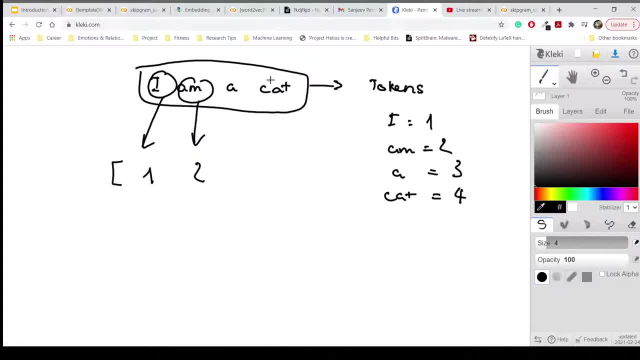 but a number is upper, see. so we have like here as a lower and this will be lower, and then next we're like one, a single unique word in the sentence. So if you have sentence that kind of like: have overlapping thing, overlapping word. 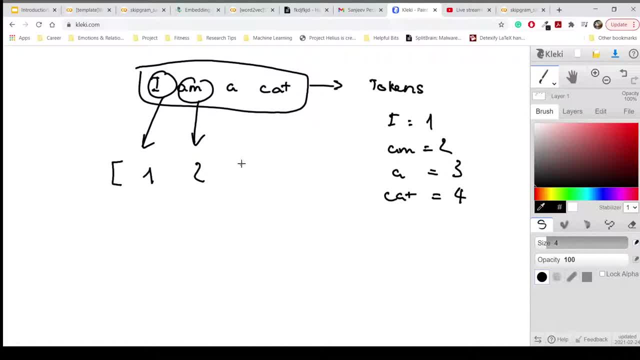 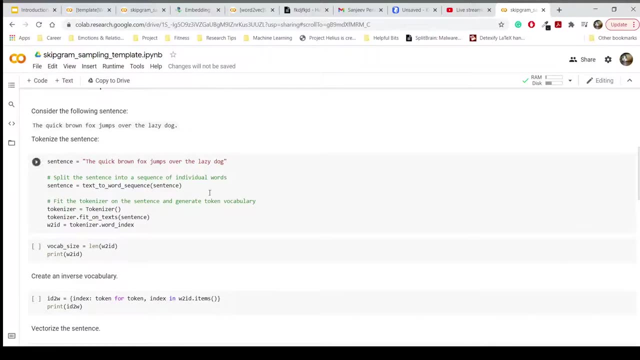 you still like view one entry in this visionary vocabulary in three, four right. So this is what we feed to a computer by tokenizing it, tokenizing a sentence, And that's about what we do here. If someone have a question, ask it now. 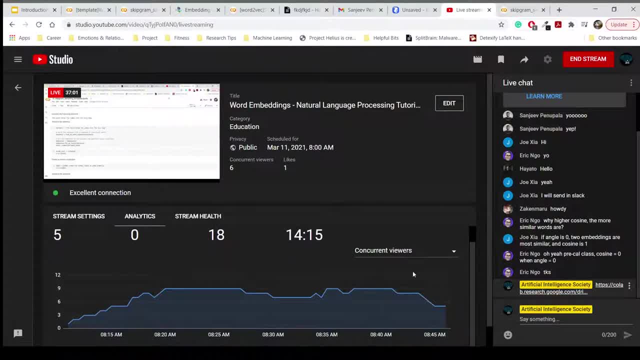 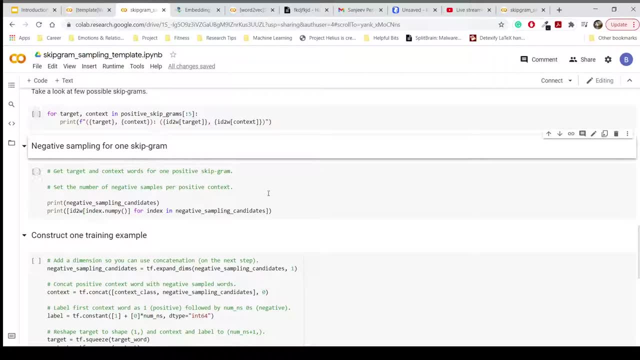 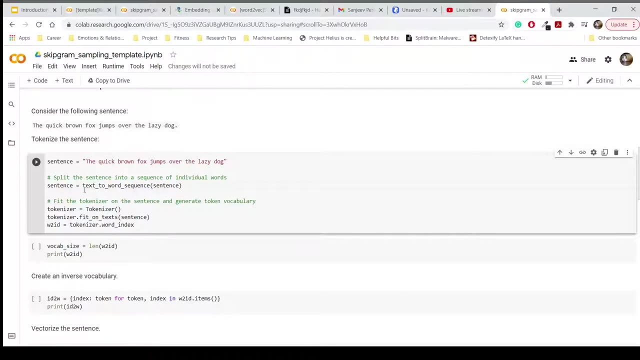 Everyone's still with me so far, All right, Oh, sorry, Okay. so okay, here we go. So here to tokenize a sentence. we have sentence here, We turn it from text to word sequence and we feed it to a computer. 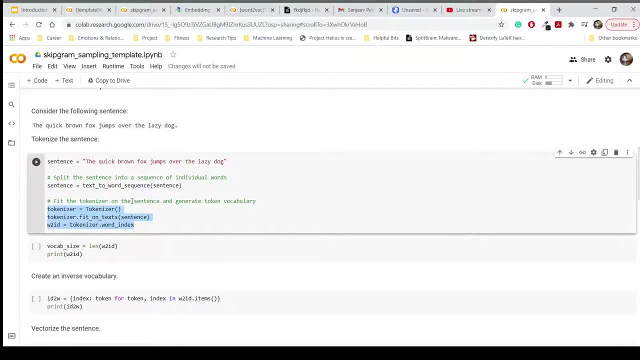 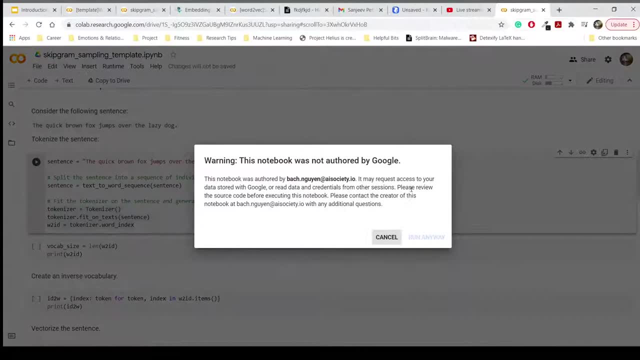 We feed a tokenizer on it using the Keras tokenizer, And after we feed it I just run the code. so far Run before. Yeah, don't worry about it. You can just copy the drive to save a version of it to yourself. 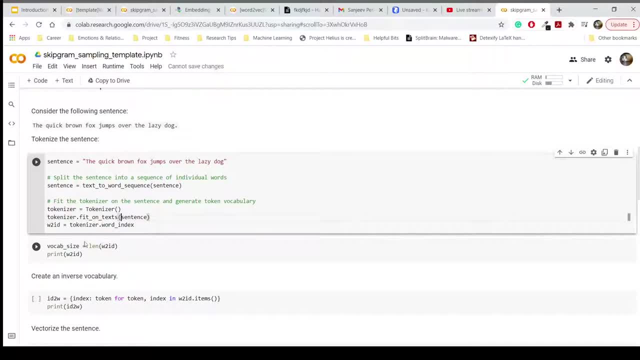 Now that we feed like a tokenizer on it, we can check what here we call the word2id dictionary, And so we take a look at how this dictionary like, took a nice to sentence here, And we can see that the dictionary is assigning each word. 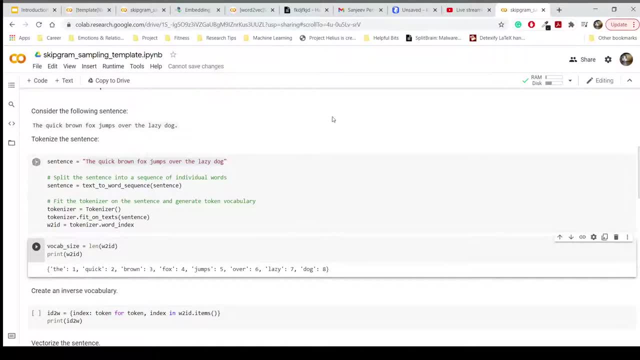 in a sentence, an unit ID right. One thing to note about the Keras tokenizer is that the more common the word is like, the smaller integer you know it to be. So you see that the one word here, There's a word here. 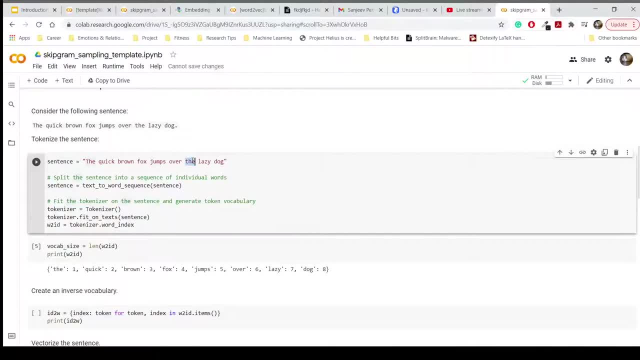 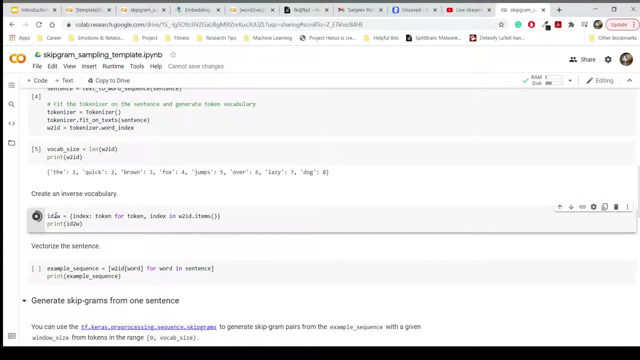 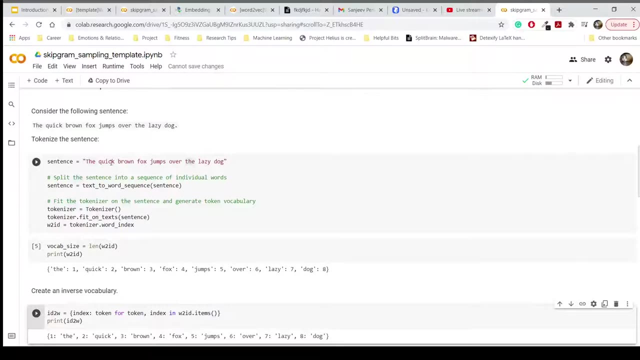 occurs two times in a sentence, right? so it's the most common word and it's also the word we like the smallest ID, and also we create an inverse vocabulary so that it can translate from numbers to words. and to factorize this sentence, right, we can just run a simple loop with the dictionary comparing it, and we'll. 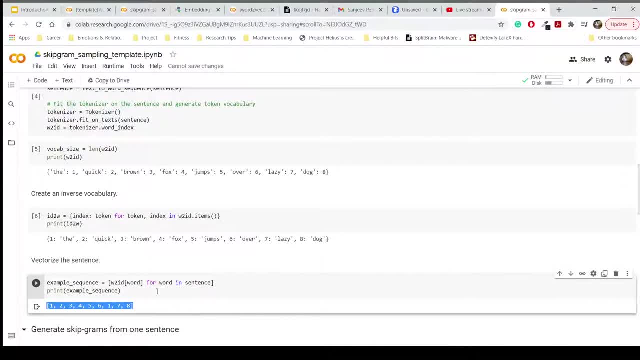 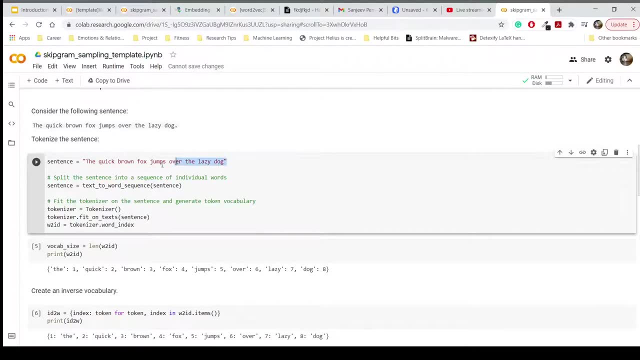 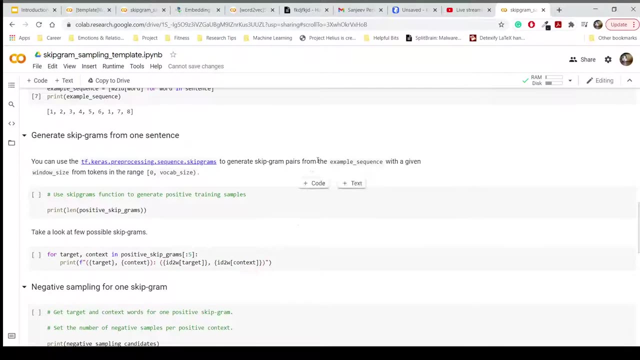 have like the sequence of vectors here, and this is the fact, like it is like a number representations, the tokenized representations of our sentence to quick run false jumps over lazy dog. all right. so now that we have like a sequence of numbers, what do we do, right? well, funny thing is, keras blubbery has 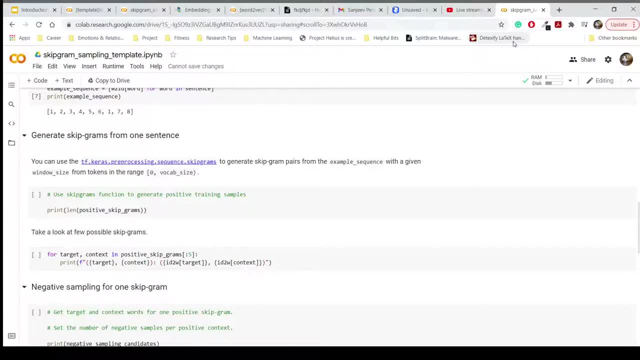 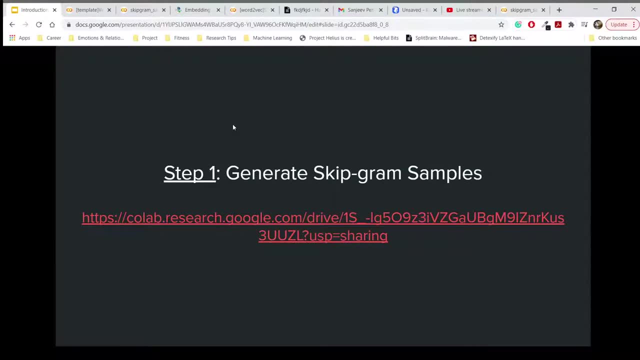 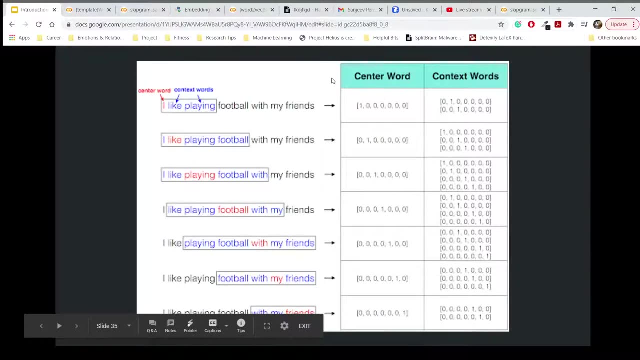 something called to skip, a function that can generate us like a set of skip gram, and if we switch with this slide right you search, it is like we can see how the skewer function itself works. we have like a sequence of words that we feed into a skewer function and 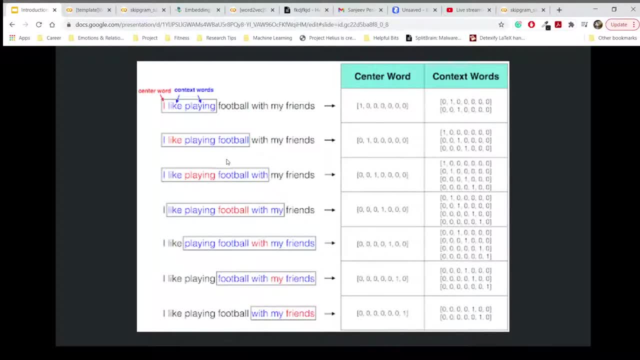 given the context window right. so, for example, like to work before the target word and to work after target word. if you generate, like some training sequence to it and here you can see that to work, it is going through the sentence I like playing football my friends, gradually and generate these. 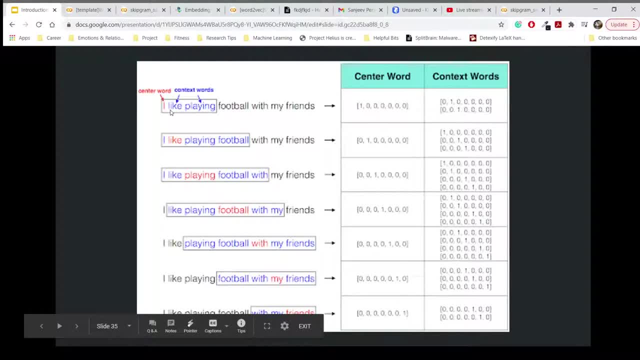 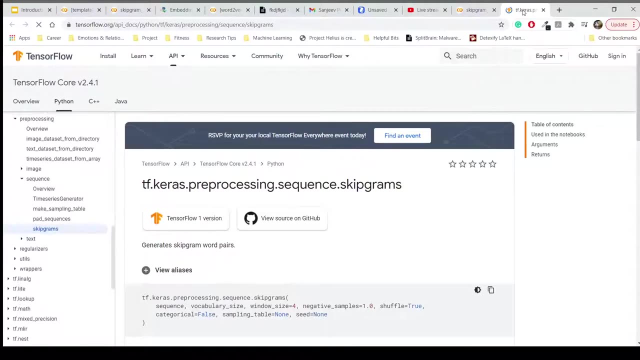 like training, instant right. so we have I being the target word and the two words near it after it, but like playing as a context word, and that's how the skewer function just basically work, and so we just take a look at what kind of parameters it requires us here so that we can use it. okay, so we need a sequence. 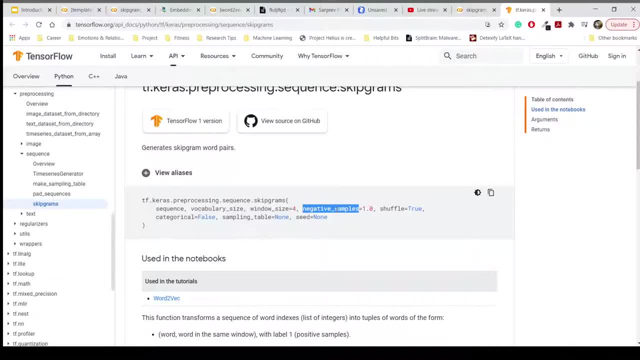 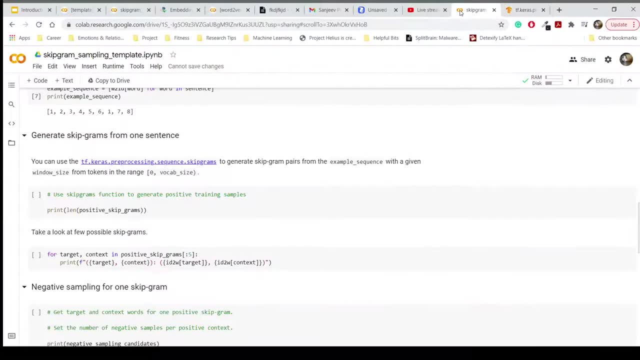 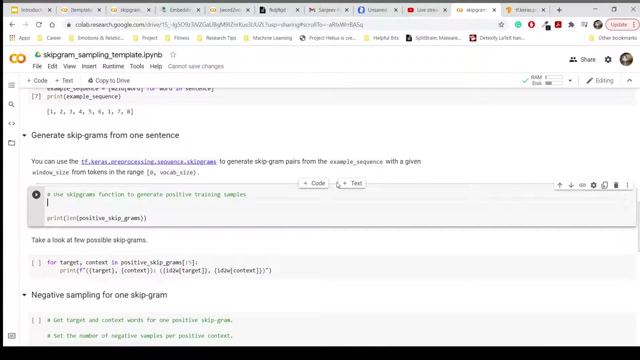 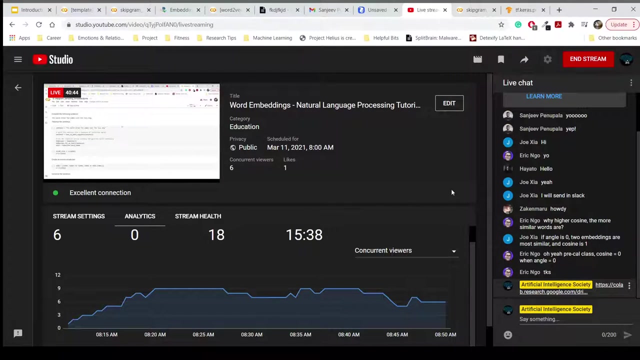 of vocabulary size for window size and a specific example, great, and where we wanted to be shuffle or not, I mean I don't care, but so what we want so to generate that we'll probably do start doing some code here. anyone have a question so far? okay, no question so far. 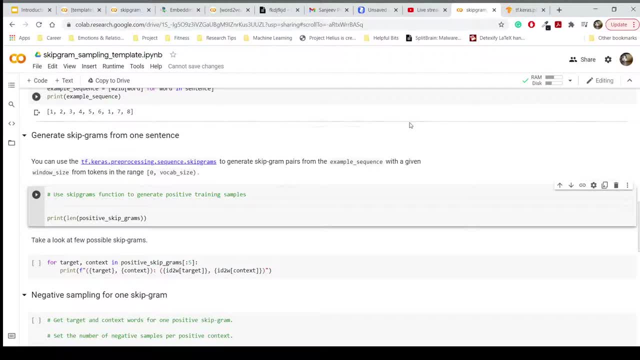 it's too fast. let's take a look at the and I'll show you guys, like the, we'll see. okay, so now if I put this the query category, we will see. that is all gon. let's see what happens if we though that here we want to set like as we seen before, right, we want to say like. 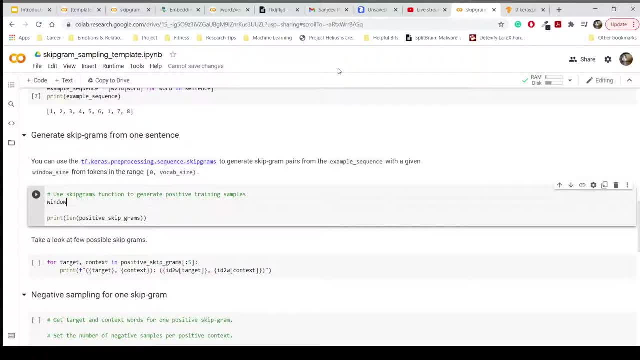 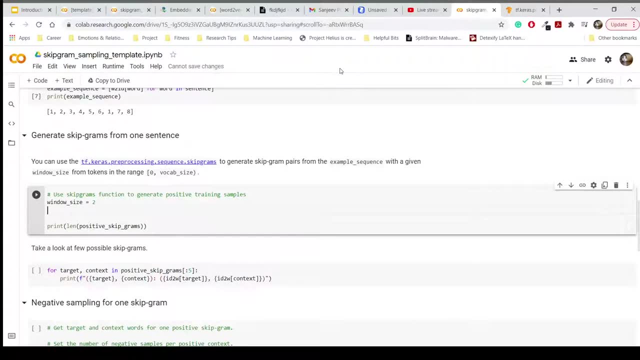 something called a context window size of two and we start by generating what we call the positive scheme grams. we just leave, like the second entry here blank because we don't want to take the second output of this function. tf keras pre-processing sequence is a previous function, very nice. 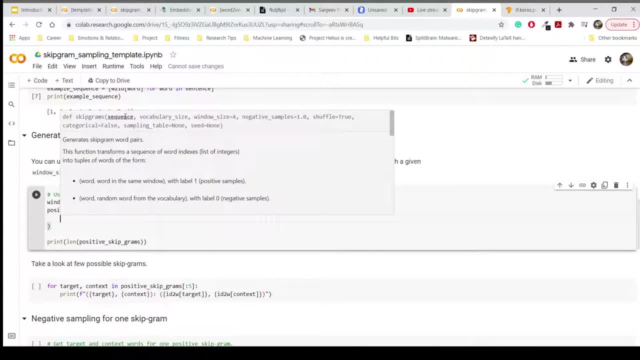 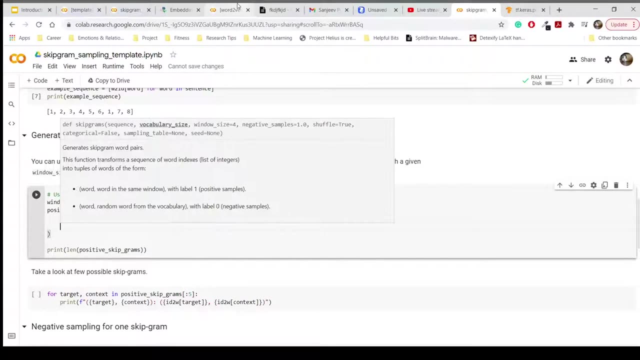 so here we already have the first thing. first we need to fill out um the sequence thing right, and we can. i see that the sequence is just either example sequence or regenerate from the last step. uh, the second variable that we have to fill out is the vocabulary size. 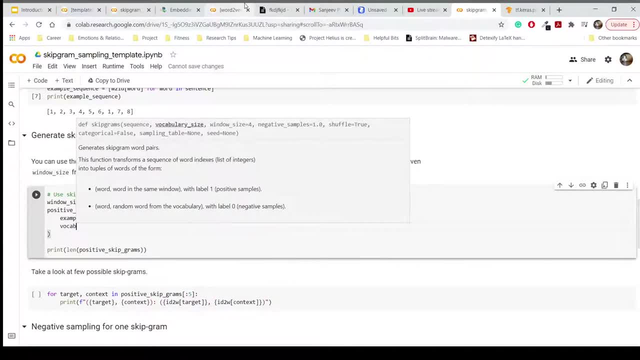 vocab subs can be very and can someone here give me a? uh, a quick prediction of what we want to feel for the vocabulary size? is for our " poor, yeah, anyone here wanna guess? uh, how? what do we feel for our vocabulary size? like, what is the scope on? like the number of other words that we're considering here? 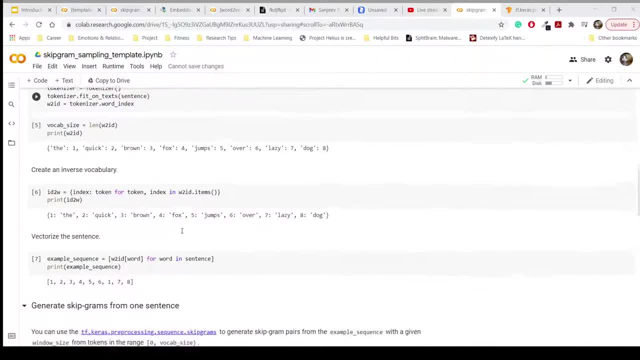 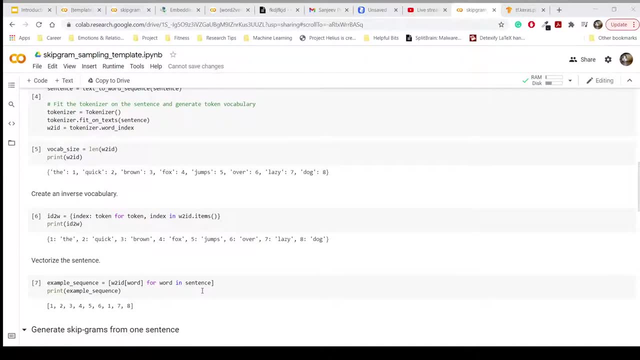 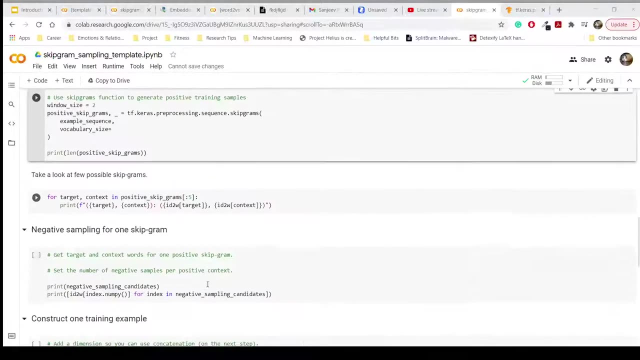 remember that we have acostable column on the left bottom and kind of, let's see what children write on us have a tokenizer and we have dictionaries of other words. so what is like the length or like the size of vocabulary? all right, no one's answering that, so, okay, this is a really simple. 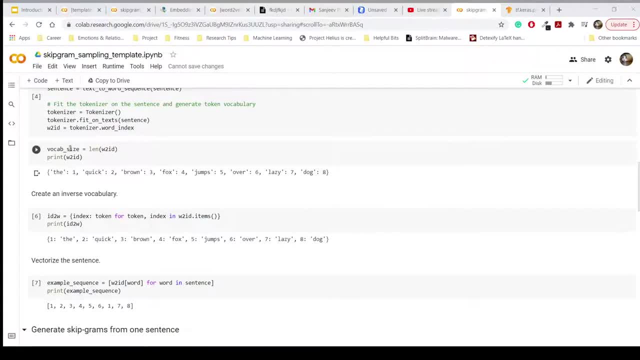 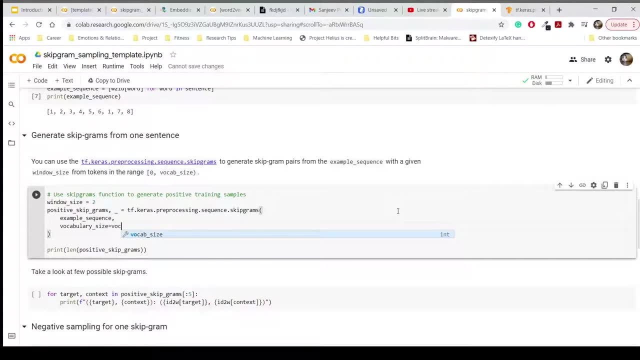 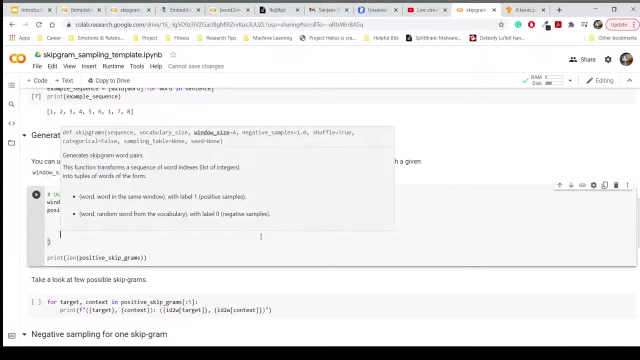 one. so don't have you, don't have to worry about it, it's just a vocab size that we already denote here. right, so we get the length of the tokenizers and we just put it here, because tokenizer already encode every single word in our vocabulary. okay, so for window size, we already set it up. 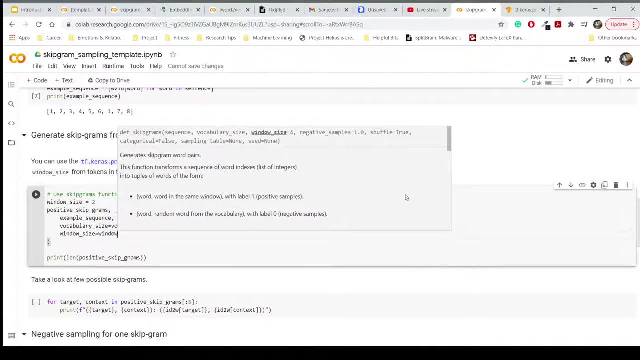 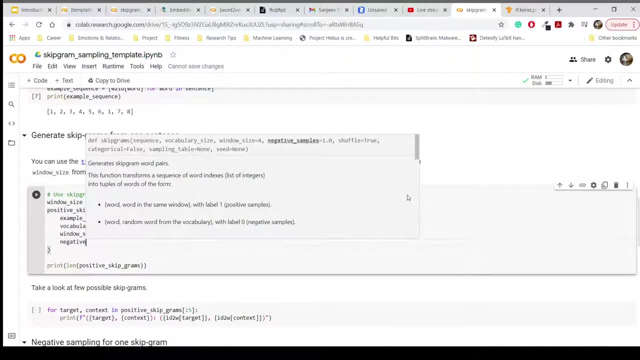 up there, so we just equate window size. and lastly, we have a negative sample. note that we just set this in the one generic function. so let's look at example. um, yes, we have question. let me check the worst number in the training sequence. uh, no, it's a vocabulary. 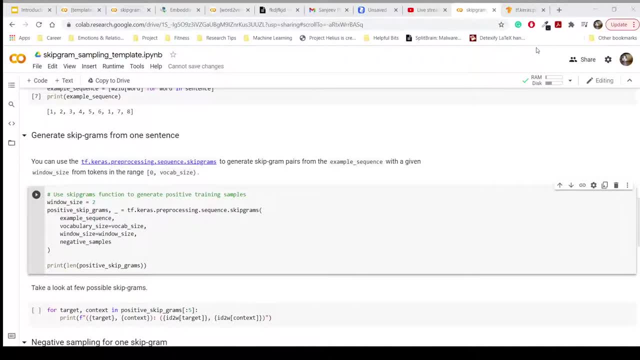 oh yeah, yeah, all right. yeah, michael got it, so okay, so we're just going to do on um. so, from for negative samples, we set it to zero because we are not um trying to generate any genuine negative sample from this function itself. it is kind of like really hard to. 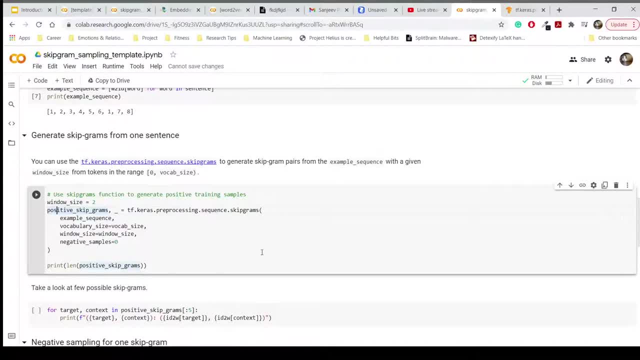 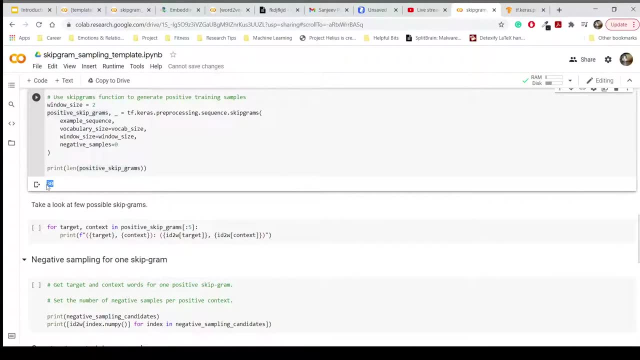 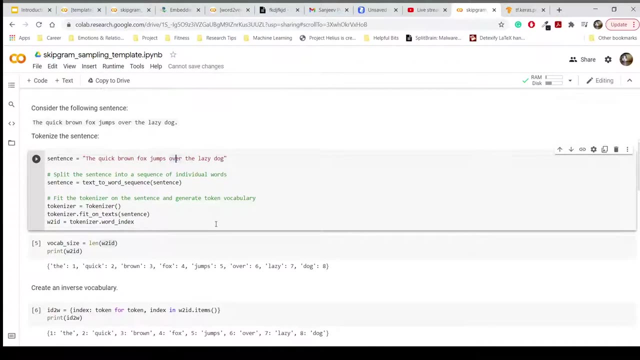 process these kind of negative samples and we take a look at creating this example anyway in our separate way. and here we go from. so, from this mirror sentence we are like 10, like maybe one, two, three, four, five, six, seven, nine nine word long sentence. we generate 30 positive, positive skip. 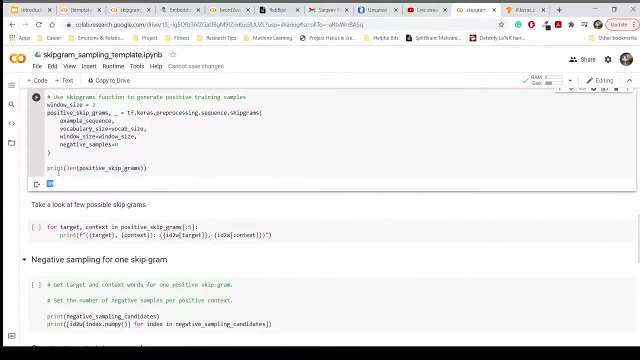 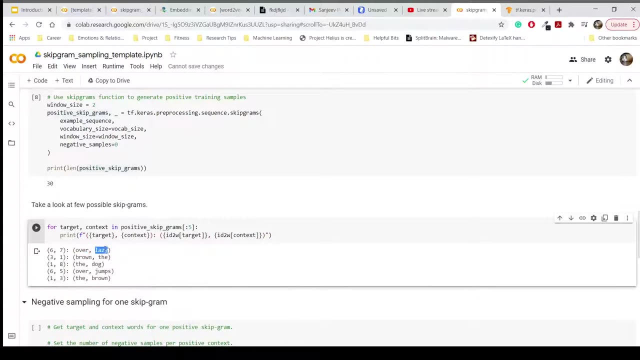 grams right, and that's quite a lot because we're sliding a window over, like each span of text of the sentence. so that's how we generate these many sentence, many instance, and we just take a look at few possible skip gram. we have the word target word over right and the lazy word is in. 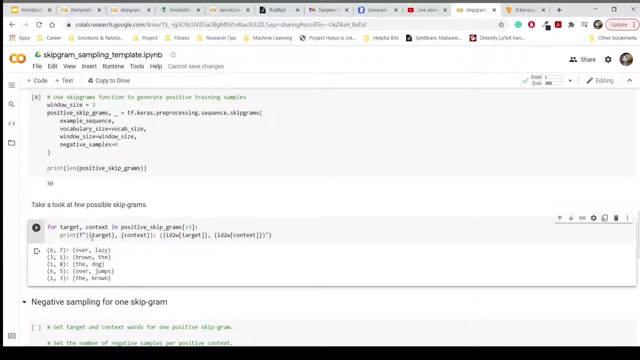 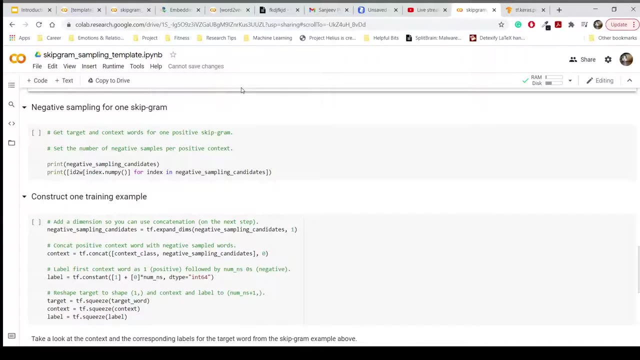 the context of this word, and also we have a couple other words in the context of our words too. the word on the left is like the target word and the root on the right is the context word. okay, so now that we generate the positive instance for the classifier. 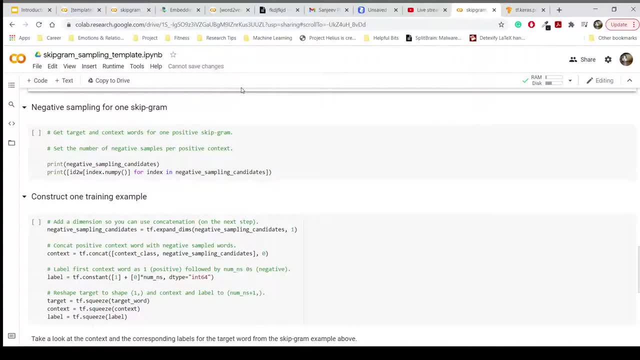 how do we generate the positive instance for the classifier? we generate the negative instant for it. right, we need something to balance out, to put the data set, because we don't want to have everything to be positive. and so for each um, for skip gram, for for each positive sample, we can't have like how many um, we kind of have like uh, how many, uh we. 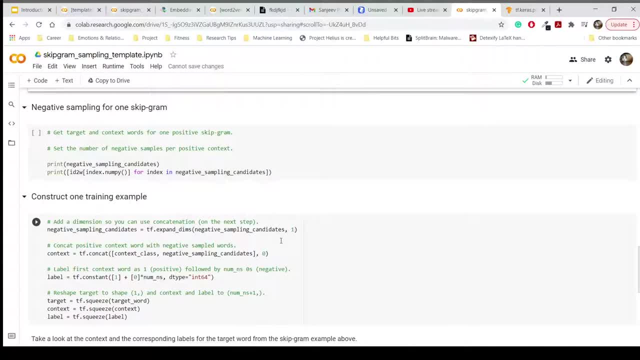 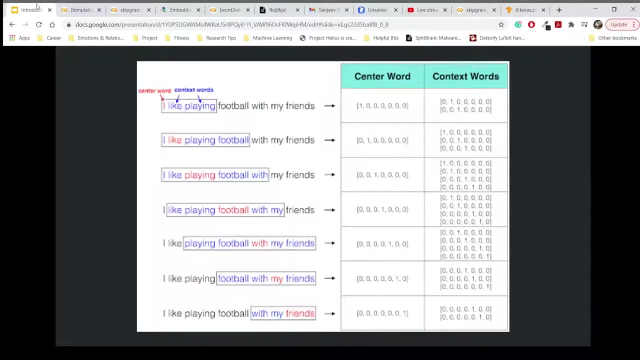 kind of think about like, if you have one positive instant, we have like two or three negative instant, right? so it is like this very specific ratio that we just set for ourselves, and so what we want to do here is that we want to- um, what we want to do here, right, is that we just 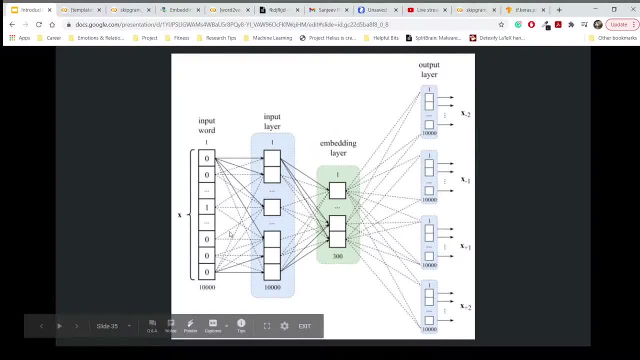 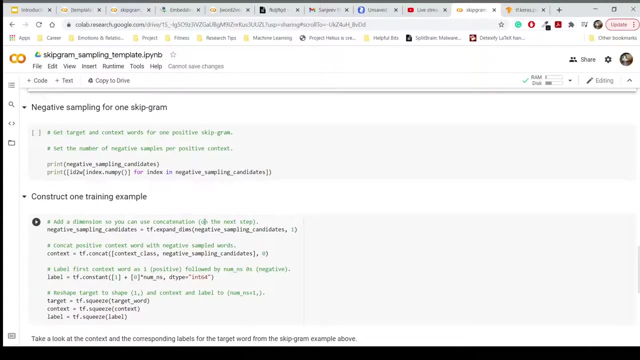 want to like, uh, randomly, um sample from, like the negative, um sample the negative samples from the vocabulary. so everything that's not a context word, we just sample it as like the not context word in vocabulary. and so we do that with a function called. we just do it, we like a function call to. 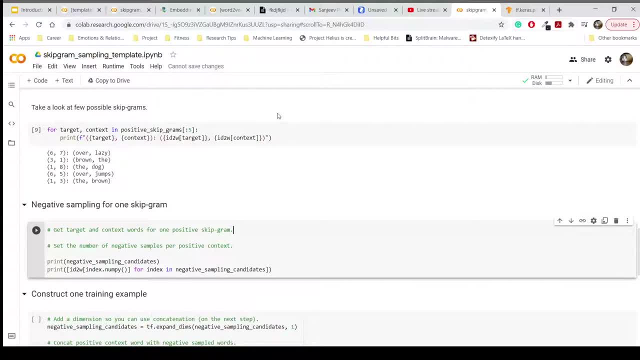 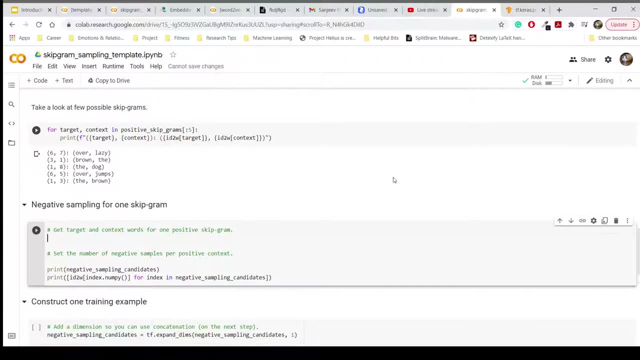 uh, to tf random log uniform candidate samplers. so yeah, it's a bit confusing to say so i just type it down first thing: first we just set the target work and the context to the, to the function, to the first positive six gram for ourselves, right? so you just get the first pair of positive skip. 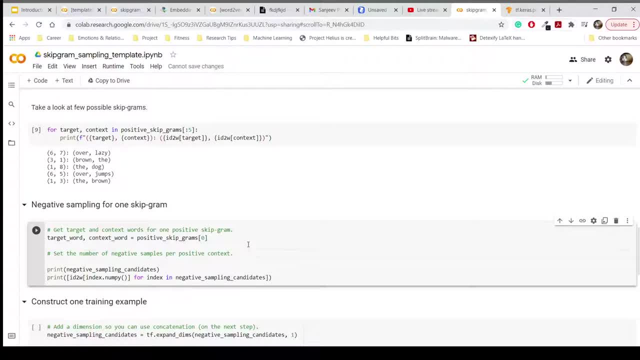 gram and we create like some negative sample for it and it is instant. we want to create like four negative samples per every, like per every positive samples. so we have number numbers of negative samples set to four and for because when we create we use like the functions intensive flow we need. 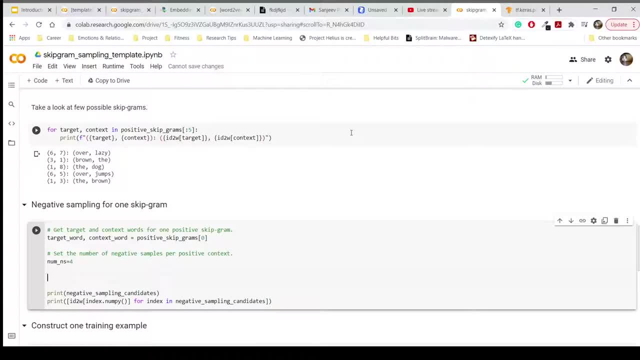 to know about the true class of um, like what is the real context context word for this target word? right, we just fetch it from what we generated from the sample where we just get here. so contact class will equal to tf. we set the constant here: intensive flow. 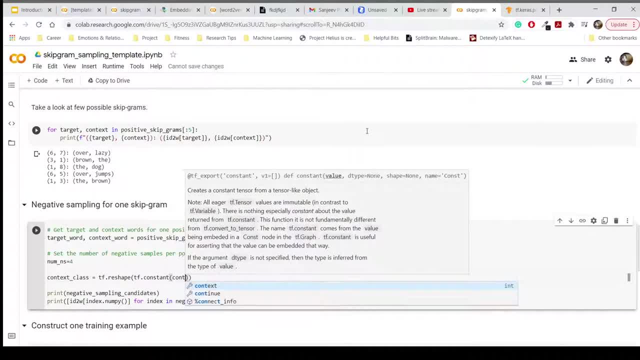 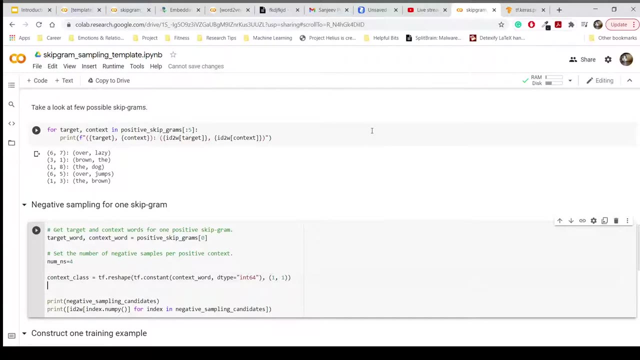 of a true word, a true class. the attack is an integer in 64 and it says: you set one one, it is a tensor of size one, one down, and we create the negative sampling candidate from here. so we call it and they: yeah, we got t sampling candidates. we leave the same two blank because we don't get a couple to form a function. 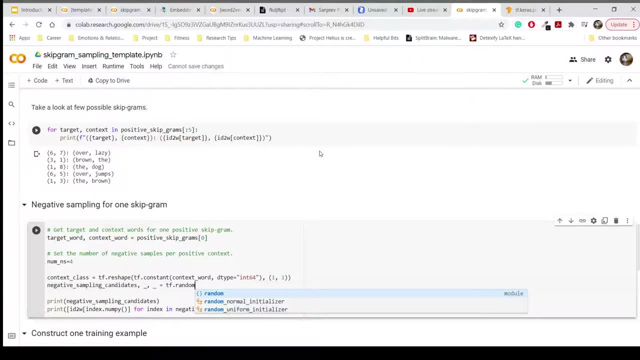 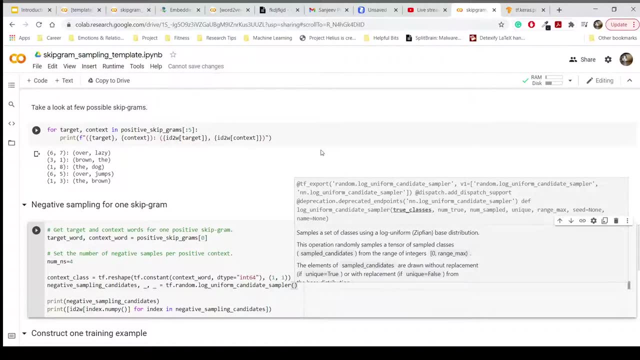 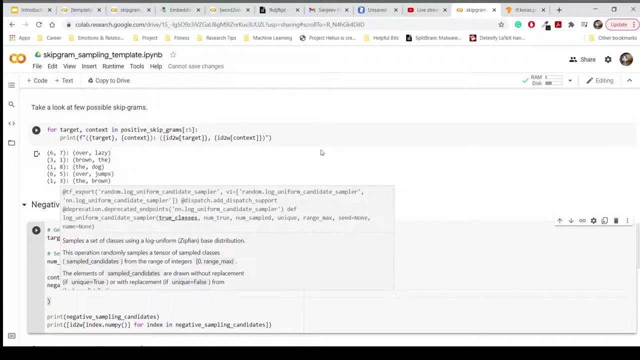 and we use a function call to log in uniform candidate sample. what this function do is that it take in the vocabulary any sample, randomly sample all the word except the word that is correct from the vocabulary. so naturally we have an attribute to this function called the true class right. so we know what is good from sampling to from. we simply 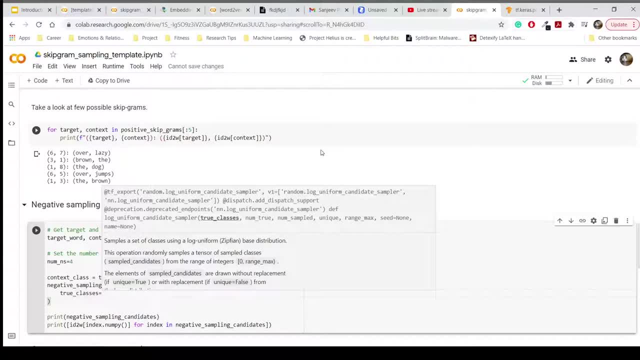 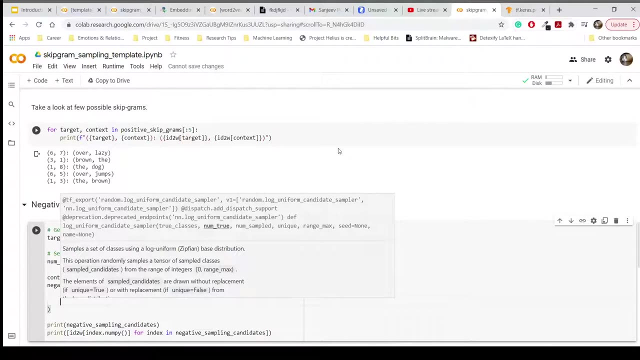 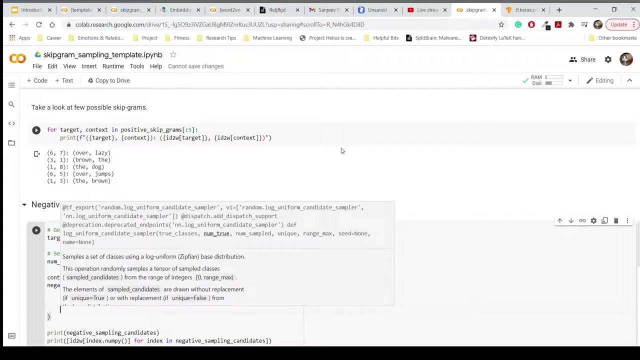 the vocabulary for negative sample, and by negative sample here we just mean that the word that is like, not actually in the context of target work and we can just have it as a contact class. uh, number of choose instant equal one right number of sample. we set it to the number of negative sample. 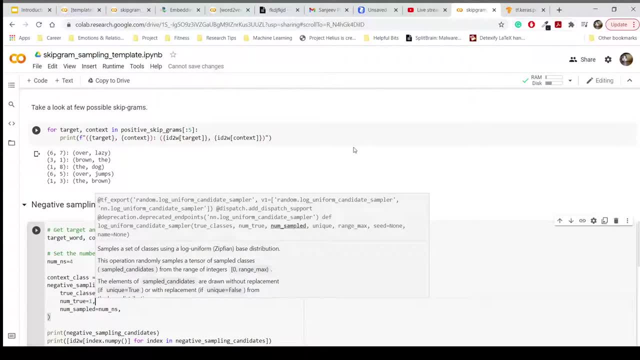 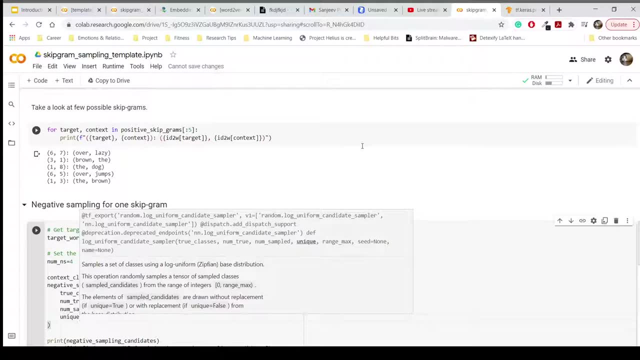 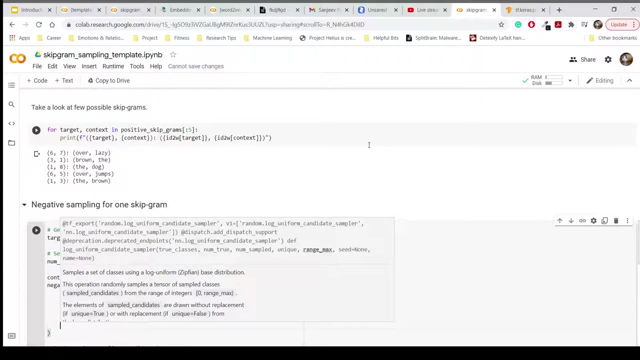 and we can do random right here. this set everything to be kind of unique. so we have true here, unique because we want them to be really. we don't want to have like overlapping sample range max. when we set vocab size we have to sample across the entire vocabulary. so that's why we set the range match here to the entire vocabulary. 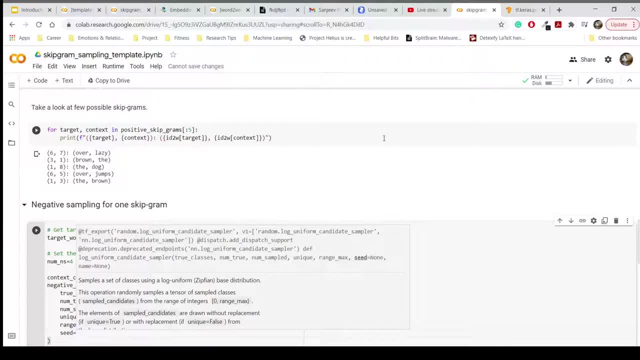 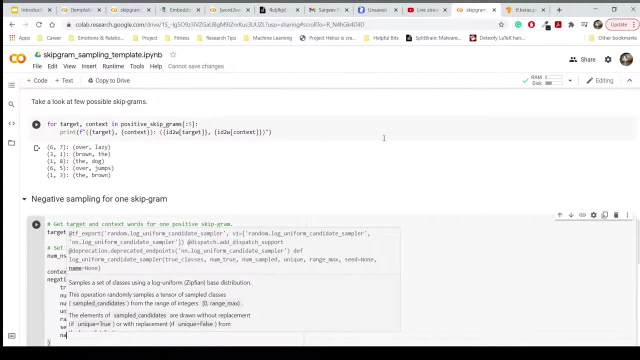 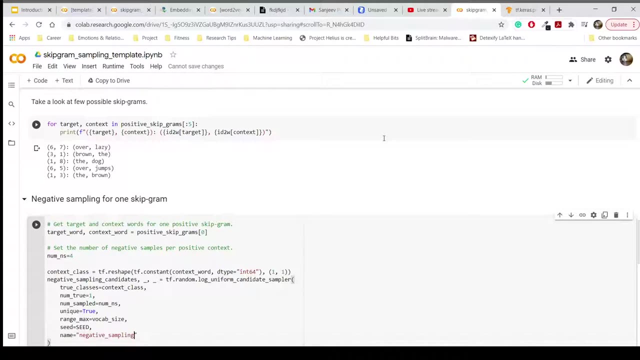 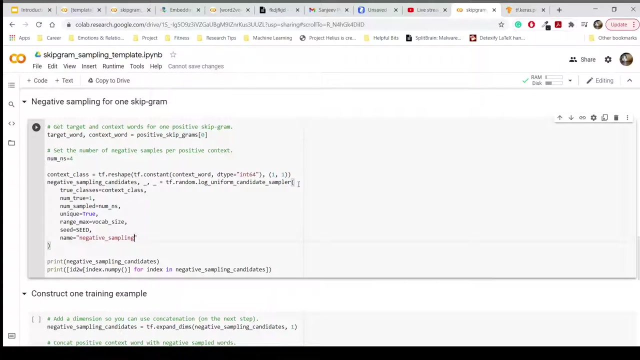 and Then we control the randomness of this sample by using the seed that we set before And we set a name to operation called the negativeSampleOperation. okay, So what this code do, like I just repeated real quick, is that we sample everything else. 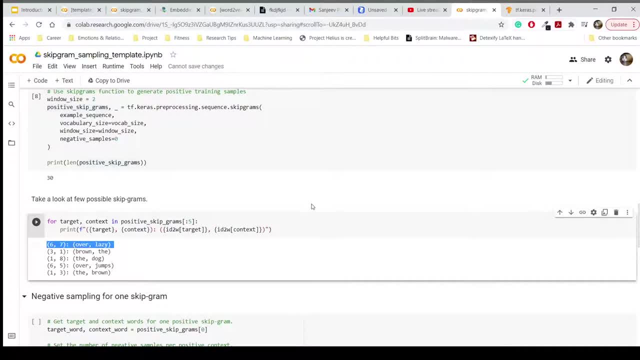 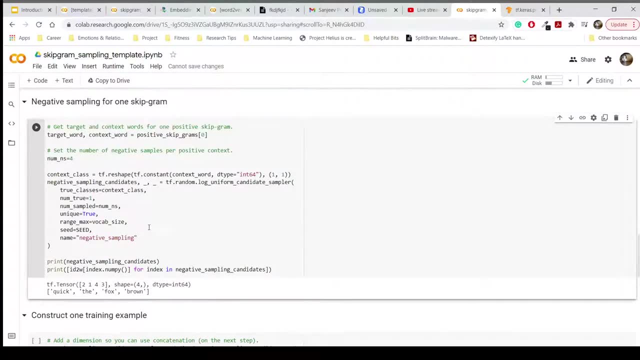 except for the context word that we got from the positive skipgram as negative sample. And here we can take a look at the candidate for the first like negative candidate for the first pair set here. So we have four words here, right, It just basically pick out randomly four words that are like not in the true class of over. 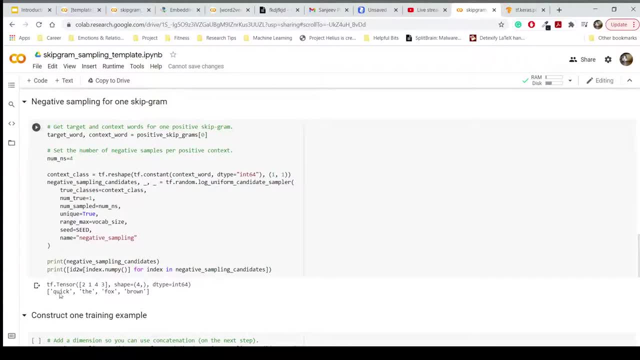 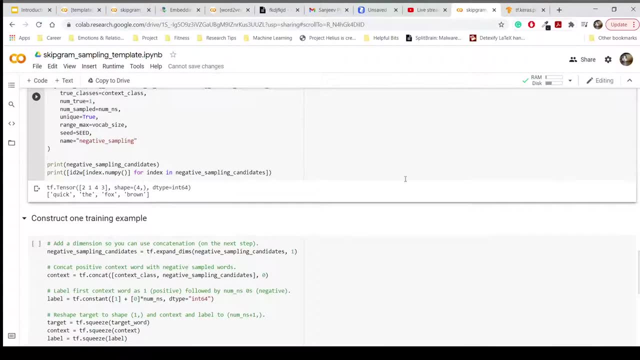 So the first target was over right, And they just pick these four as something that's not occurring, Yeah, Over. And now that we already have the negative samples, we try to construct one like training example. Let's see if we have any questions so far. 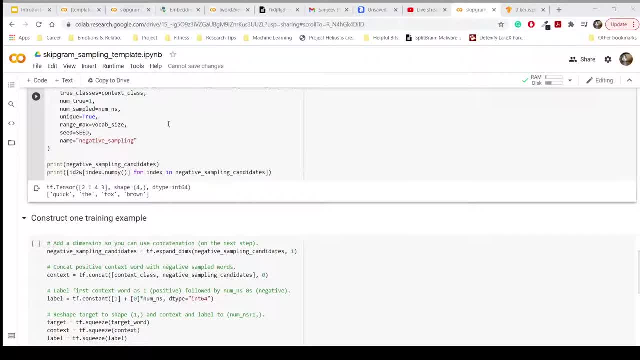 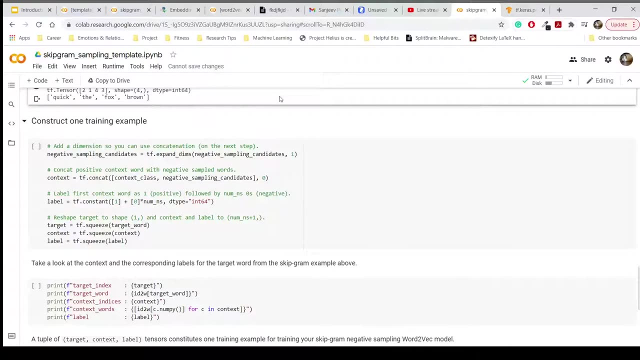 Okay, No questions so far, all right. So now that we have a negative samples, We try to construct one training sample And here are some code to just do it. So what we are trying to do here, right? Um, I just switch this on real quick so we can have- we go view- a quick intuition of 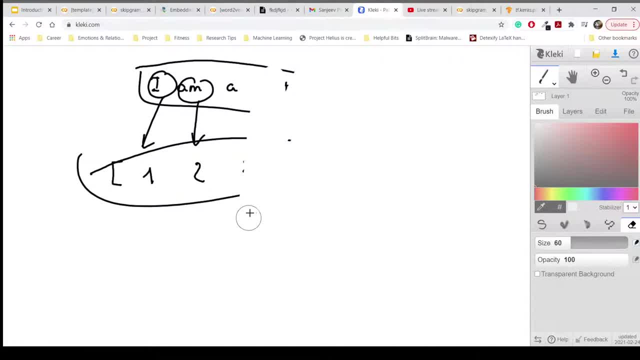 it Okay, Okay. So now that I have a pair word, Uh, cat and cute, Right. So this is the target word and here's the context word. And because this is like a true class, like the positive skip grand sample we have, like 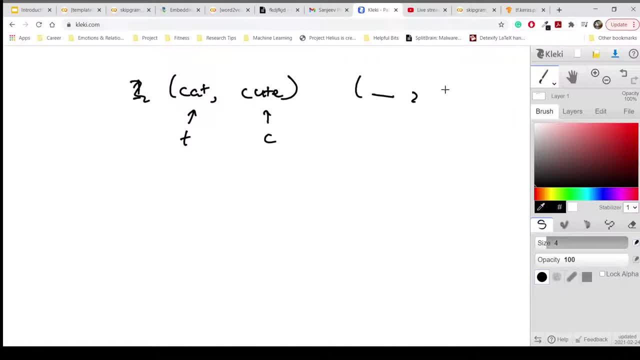 a couple of like negative sample, which is cat and dog Right, Which is basically just negative, Because why would you have dog in the neighborhood of text text of cat uh truck, for some reason? And um, what do you call uh hand right? 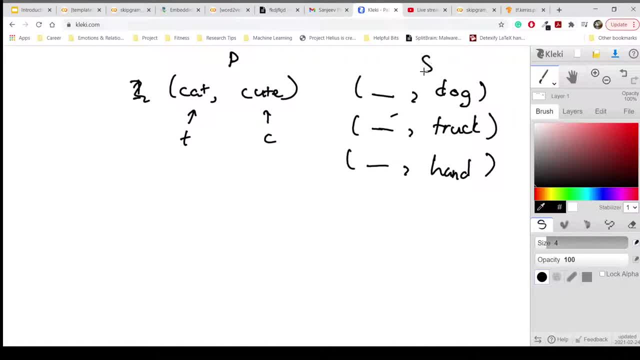 Okay, So here is our positive samples and our negative sample. What we do here now is that, uh, we have a true class. Uh, we have target word, which is cat, right, We feed it to the classifier. and also we have- we feed it- a vectors of like context word here. 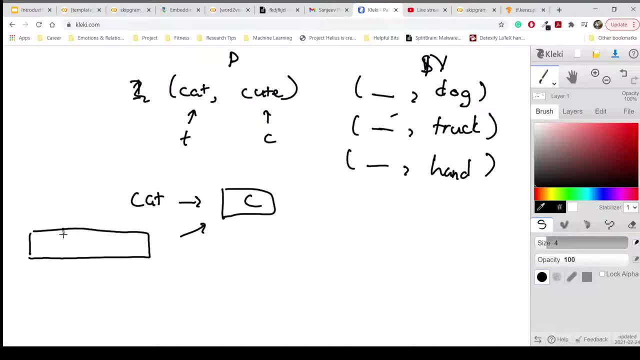 And the context word here is just like a training sample, which is cute, Right, And the three other negative um samples, and what the classifier try to do now is that you generate like a vector Right Classifying if this word is going to be likely to occur near cat. 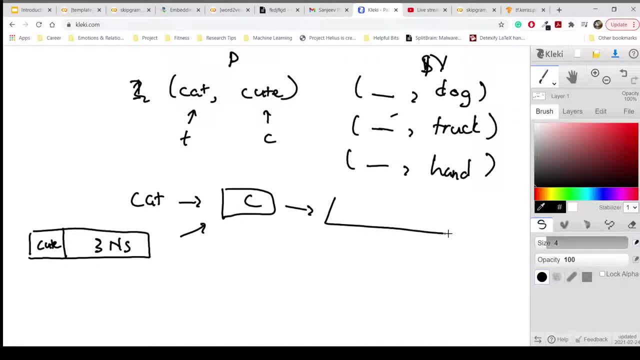 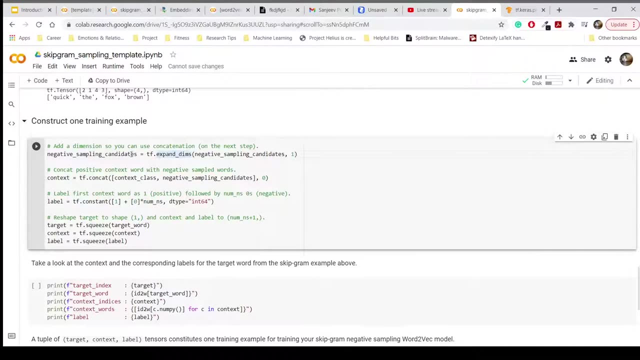 And because we all know that Q is a real class, you classify something like: we have like three negative, negative sample here, So we have something like one zero, zero, zero And that's one of our training sample. And in this skip gram code we just have here constructing uh vectors of negative sampling candidates. 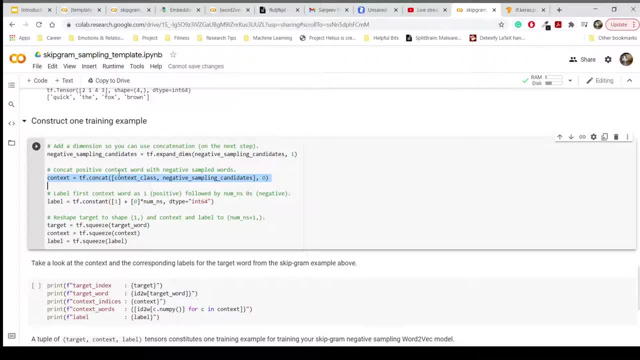 Uh, we, uh. we concatenate like positive context word with these negative sample word. We label them, So one for the one for the positive one and zero for all the negative samples and we squeeze them to some of these like global vectors. If you run this code, we take a look at the context and corresponding labels for our target. 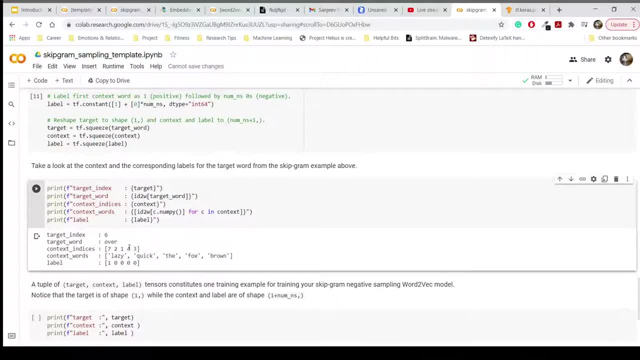 word Right, So just target word Right, Okay. Okay. So we have a target number And these are the context. What are we generate? Lazy is the true context word And the other guys, I like to fake one. 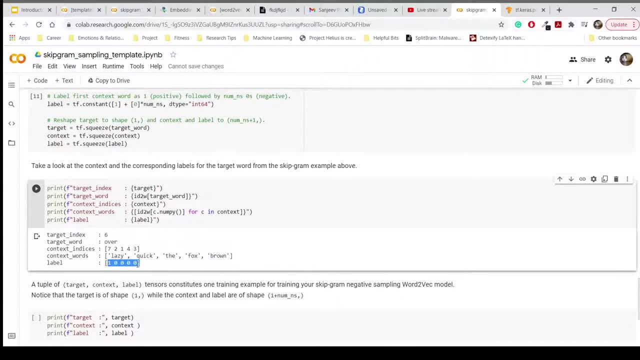 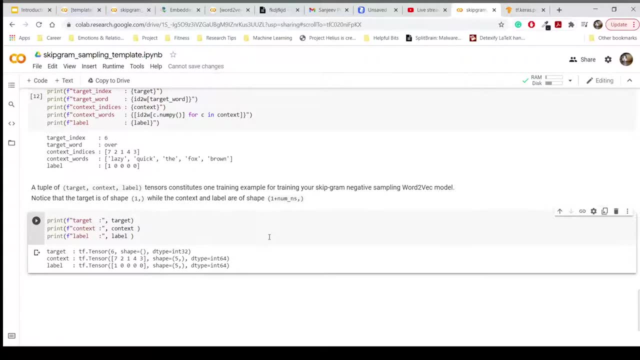 So to classify correctly, classify these guys Right. So we want zero, zero, zero, And that's one afternoon sample. And so, what case what? we feed your model itself. we feed in a target numbers because we are denoting every single word as the integer. 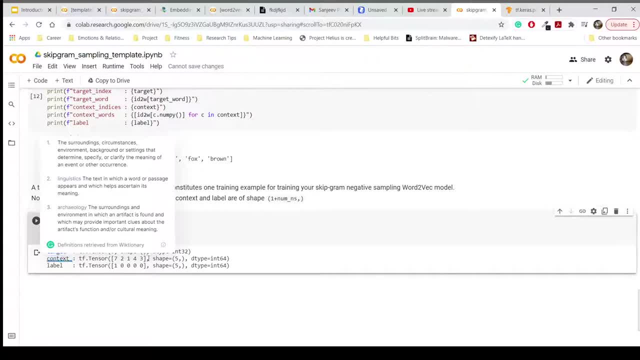 Right, So we just feed the model integers, Okay, And the context vector Right, And the model will try to generate this label. which label, if this, this guy, this word will be in the context of the first word, or not? 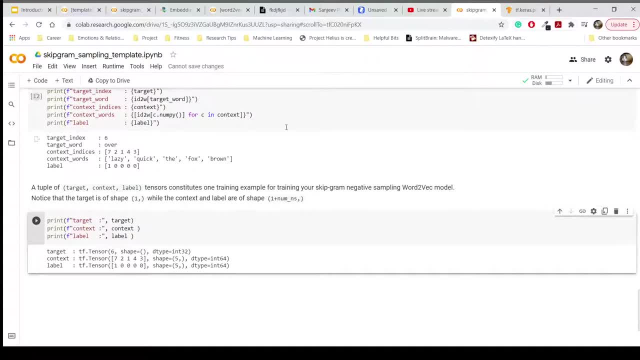 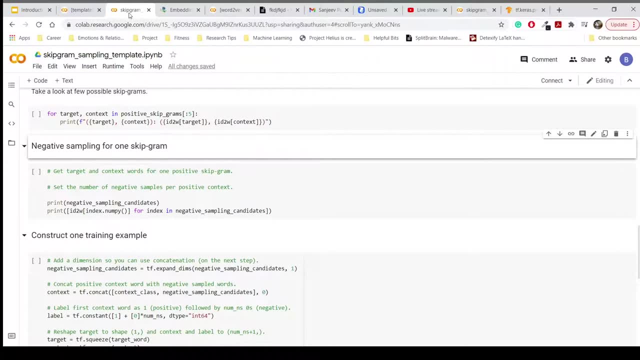 Okay, Now that we know how to construct a skip grant sample, a skip grant training sample, right Now that we know how to construct a skip grant training sample, we take a look at how we can create the model itself, like the neural model. 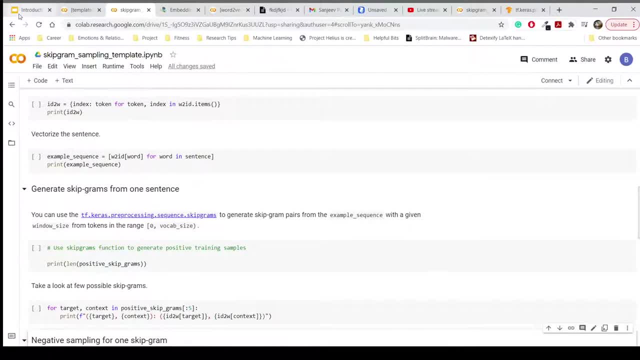 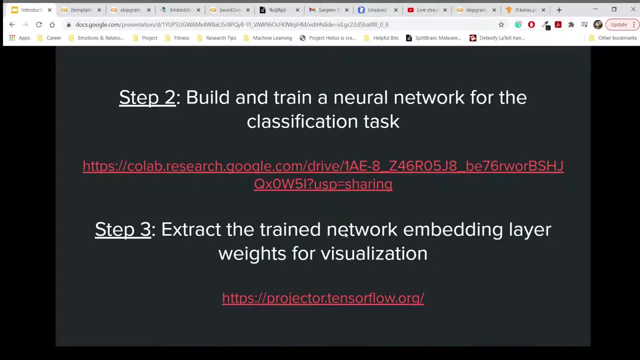 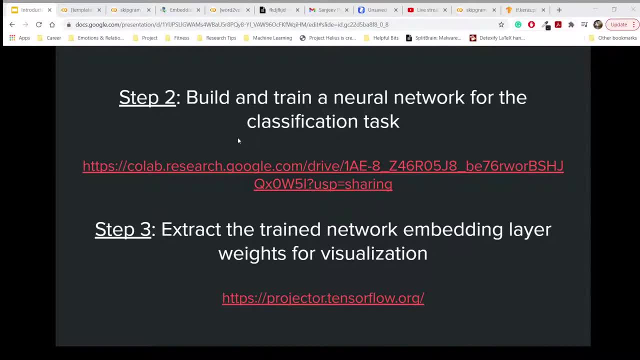 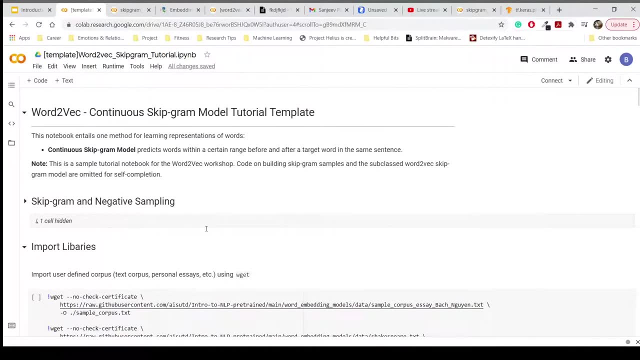 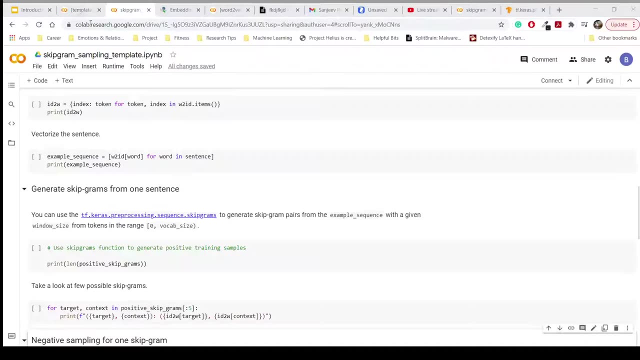 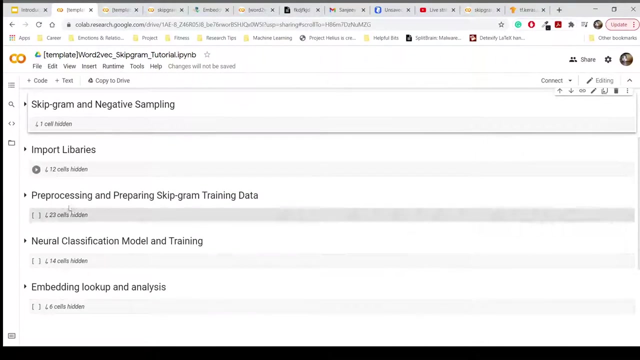 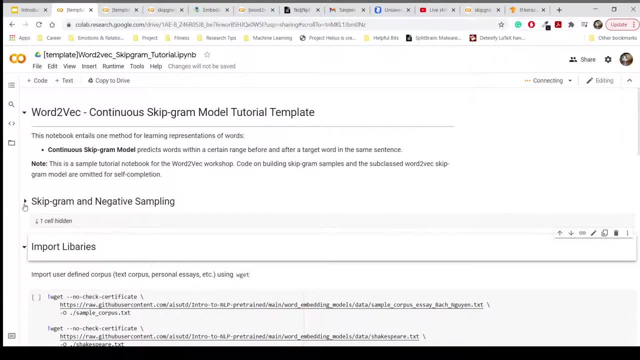 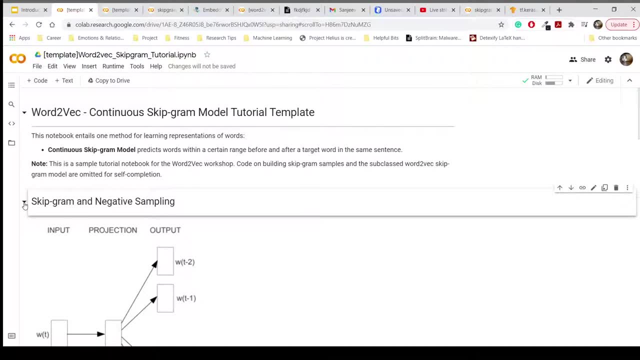 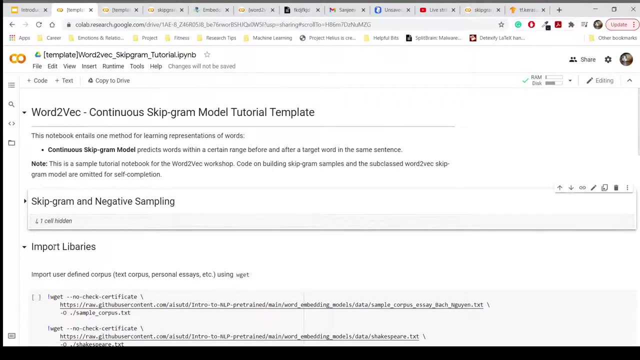 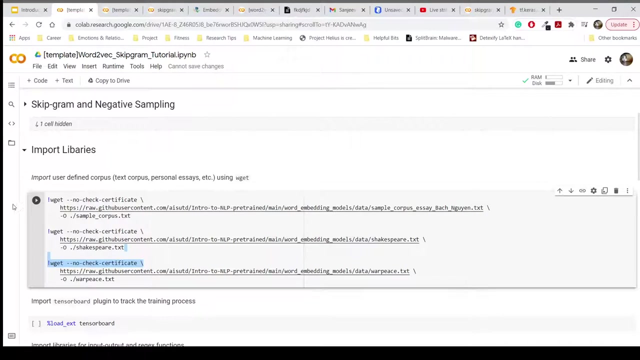 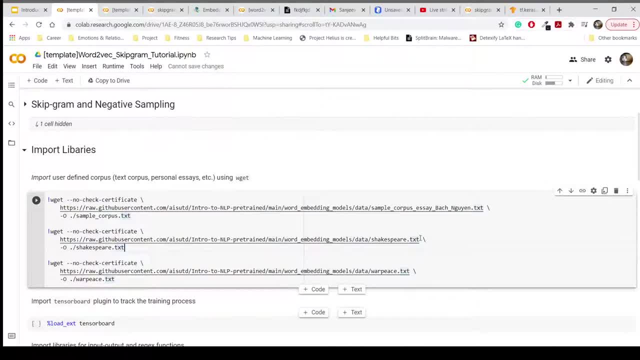 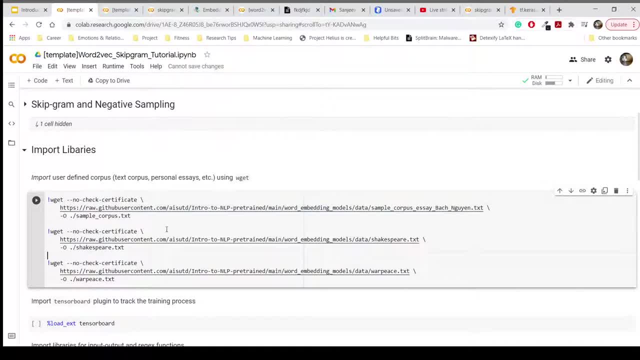 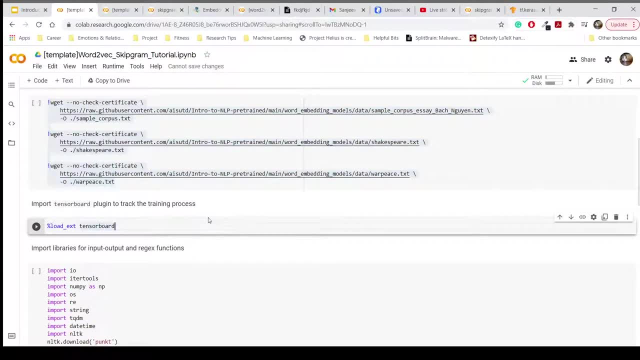 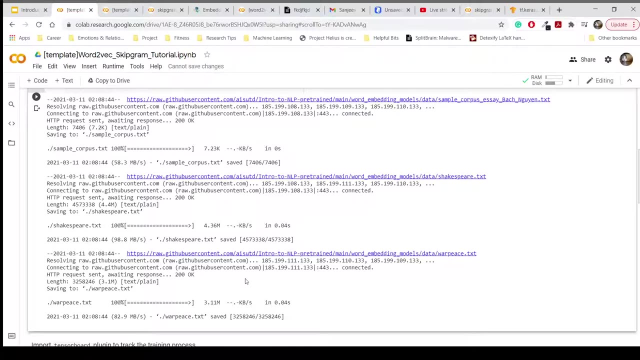 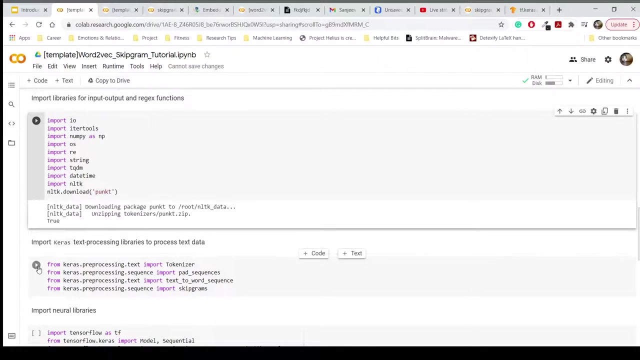 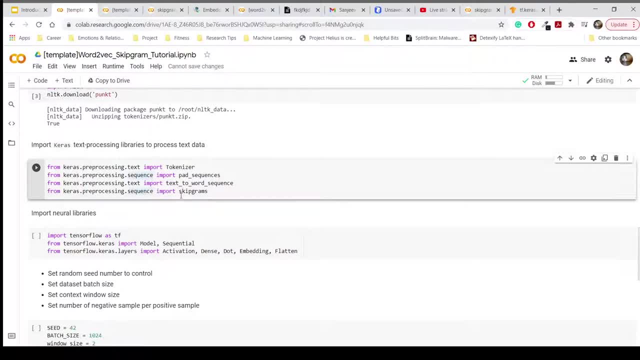 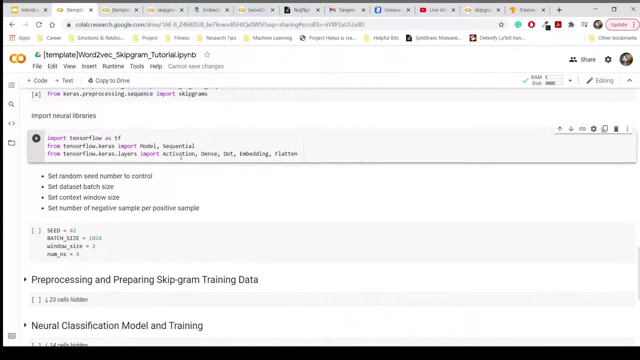 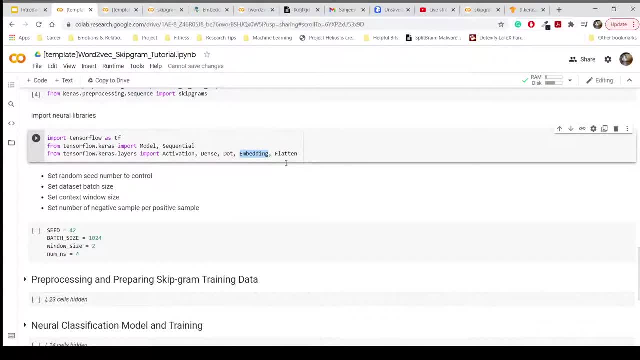 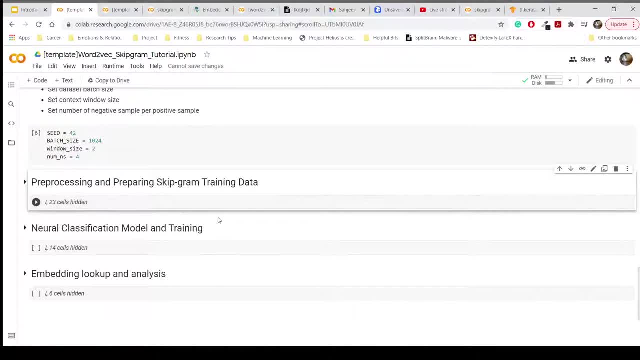 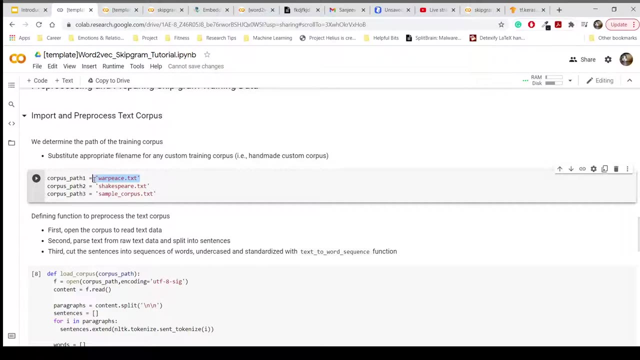 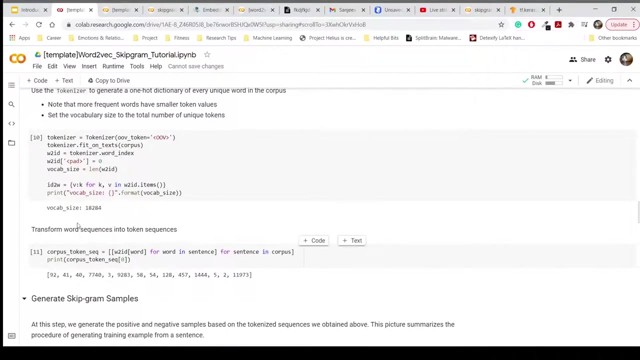 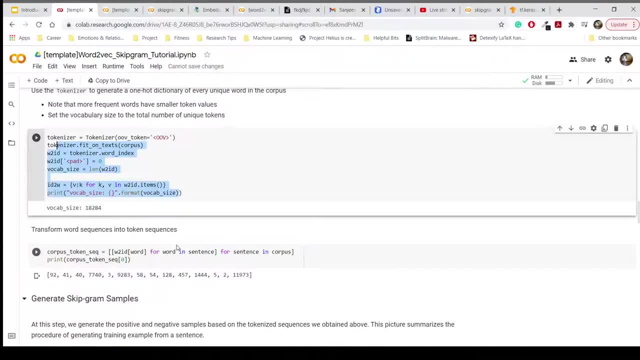 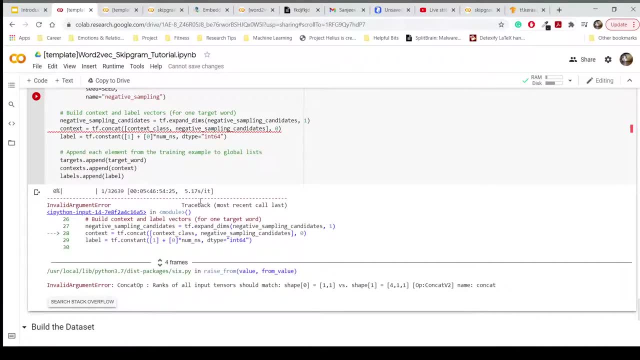 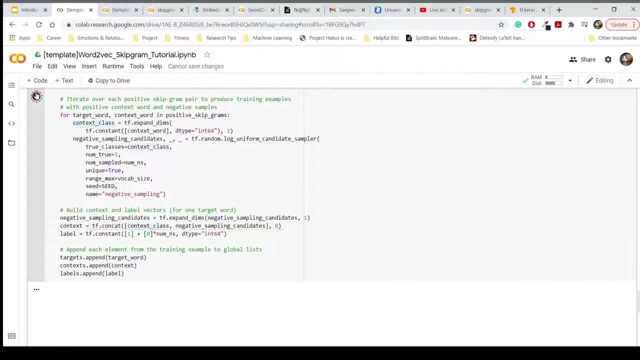 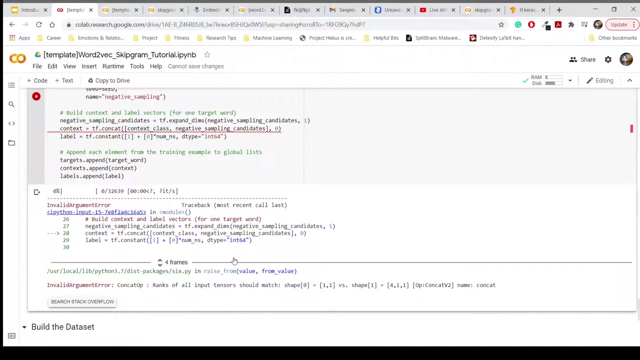 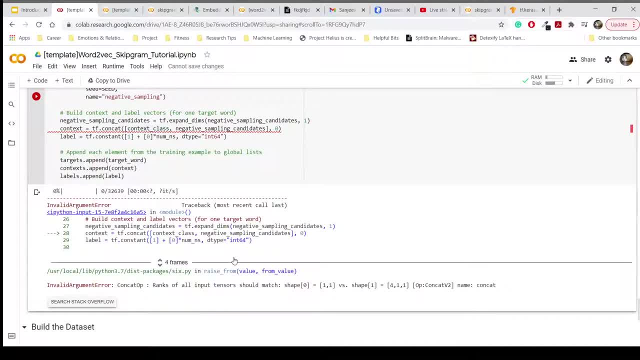 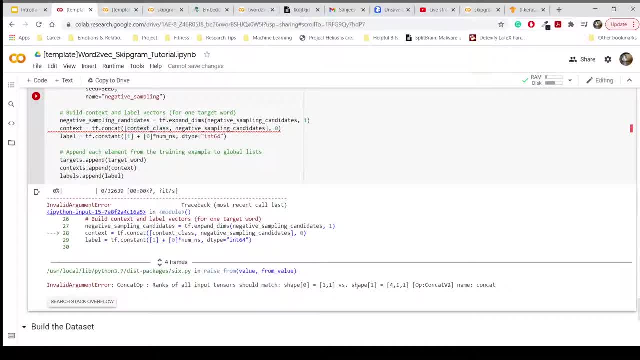 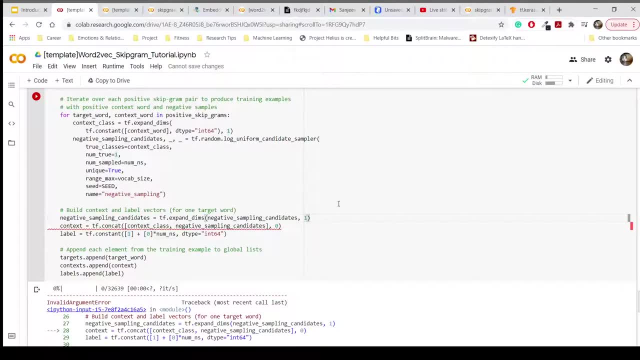 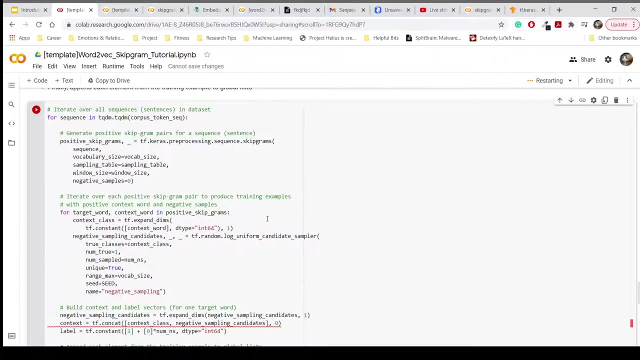 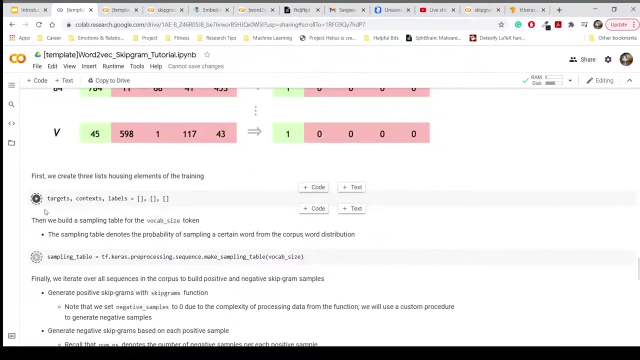 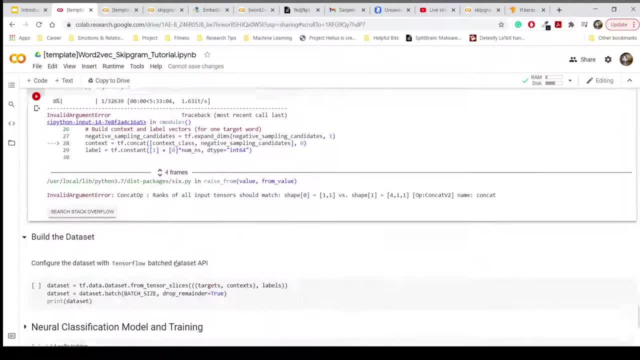 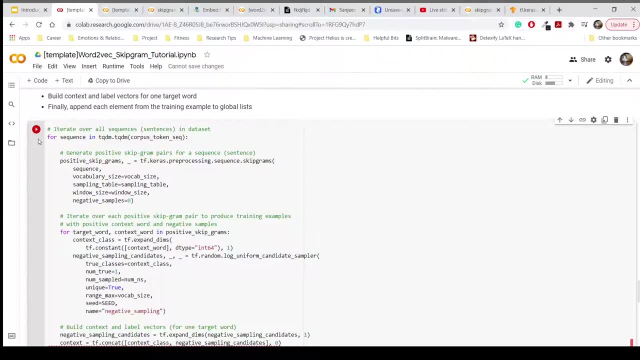 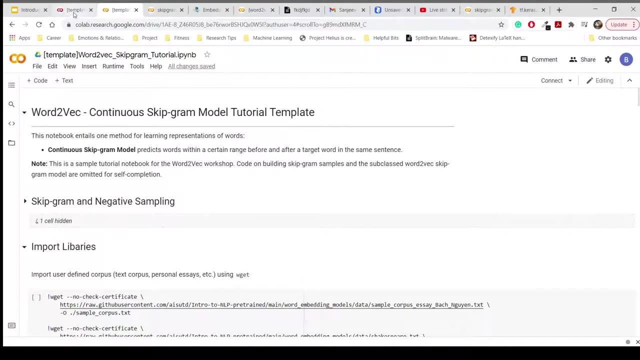 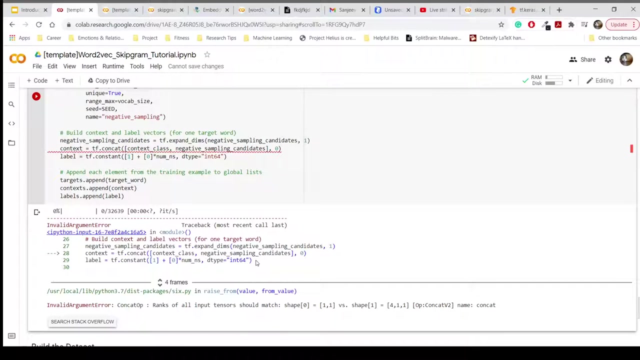 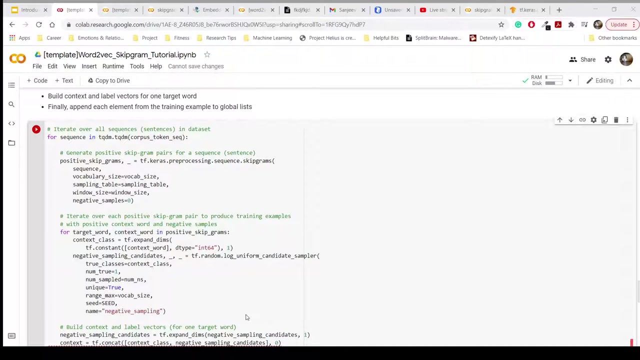 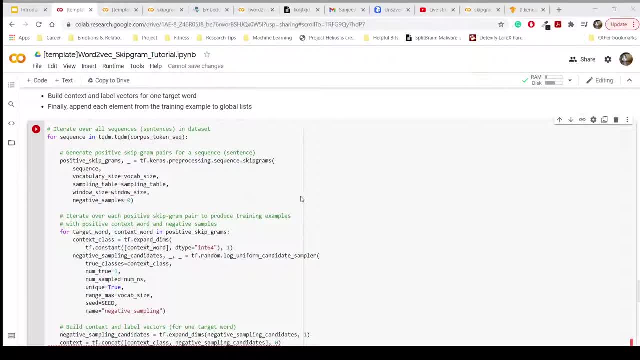 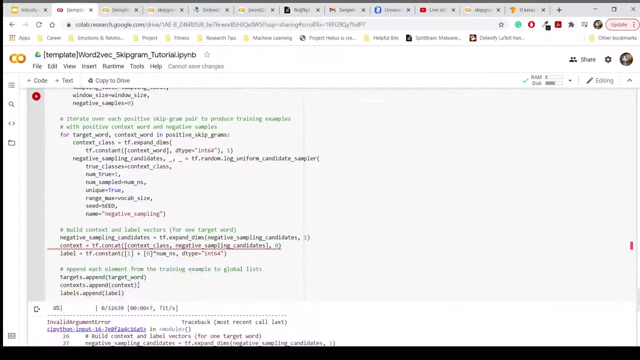 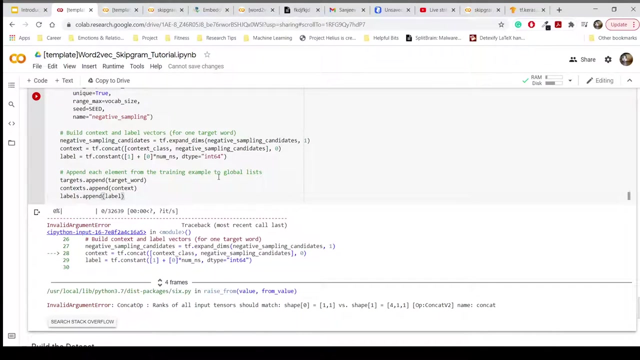 You don't have to take a look at the code, because it's just the same as what I demonstrated before, but I just put it in the loop so that we can do it over all training samples. See you later. If someone hears any situation, they'll report it. 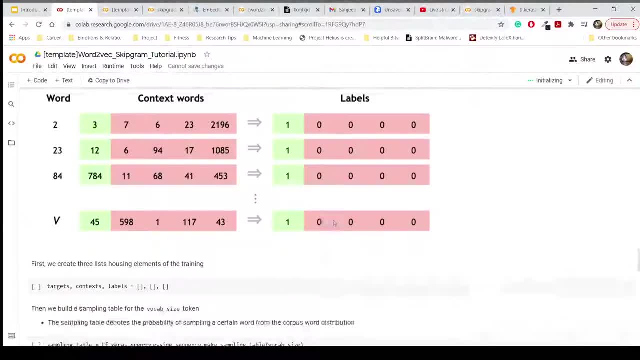 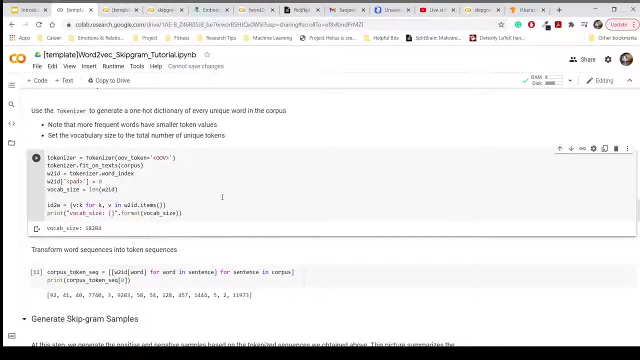 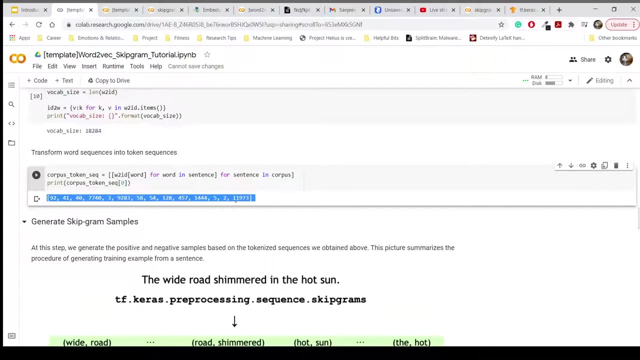 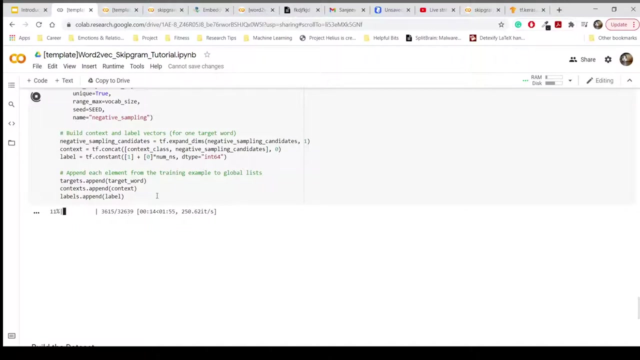 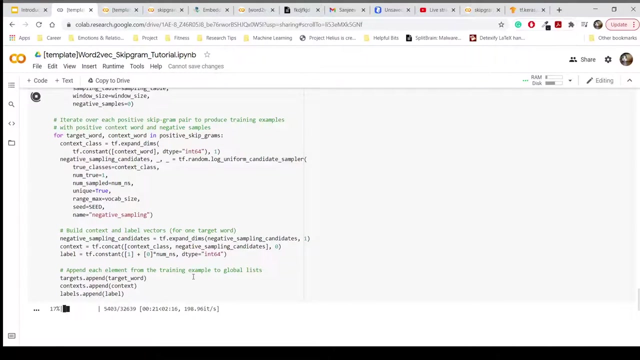 It's like a sample sequence of it's like a sentence, but we tokenize it and vectorize it And what we got here is a sample And here we are running the code to loop like the skip-gram generations That we just taken a look at before. it's gonna take a while- two minutes. 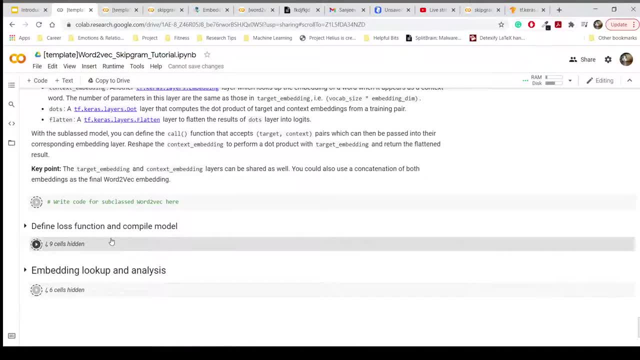 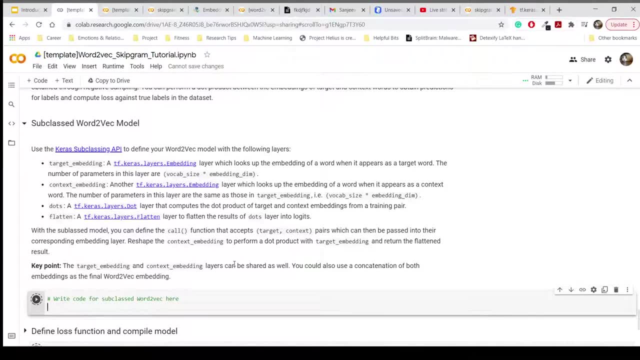 And meanwhile, we're going to build our neural model for that. So, yeah, I have some notes on how to generate, to create like a neural model, right, So let's just create one from scratch. What we can do here is, instead of using our standard, adding layers to approach, to TensorFlow. 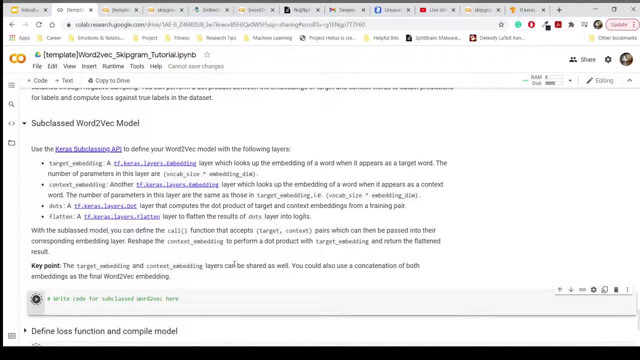 we use subclass. we use a method called subclassing- model subclassing- And what I mean by model subclassing is that we just define our own neural models instead of having to create a sequential one and just add a layer to it, right? 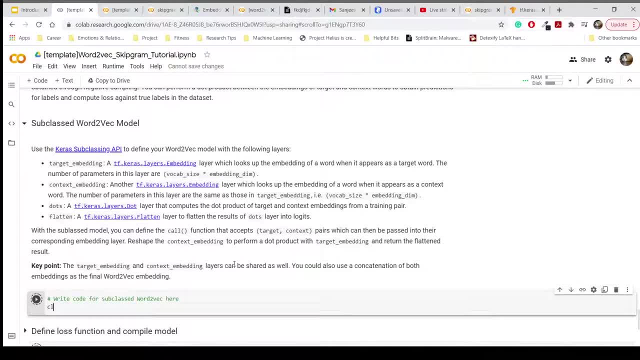 So first thing we do here is creating a new class called work to vet, because that's the model we tried, And we subclass that from the Keras model library. And the first thing when we do to subclass a model is that we have to define an initiation. 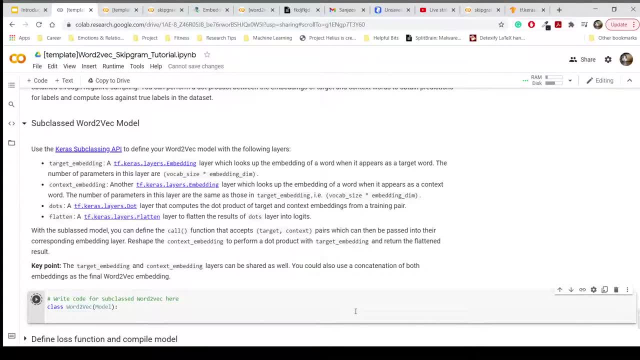 to it. So the initiation function looks something like this: right, We just define the init. This is what we recall when we create a model. So self-snare-thing will cap size. So that's it, Thank you. This is one parameter that we need, and also the embedding dimension. 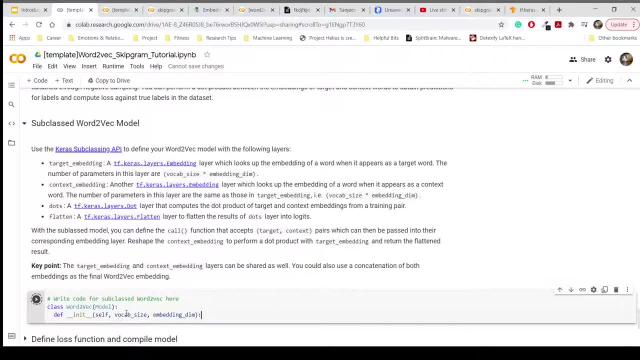 So what model we attempt to do here? is it reduce the vocabulary size to embedding dimensions, which is originally like around tens of thousands, to like a couple of hundreds? embedding dimensions, right, Okay, So we just super set a name to it. Word to vet. 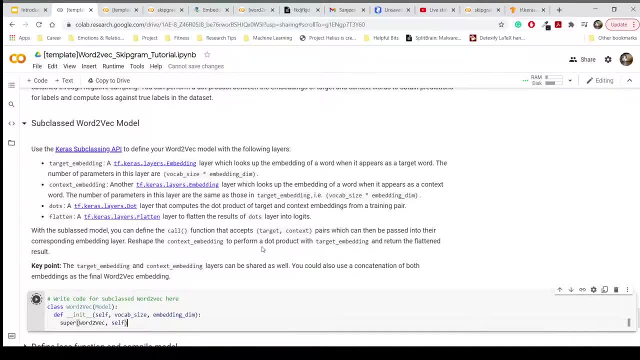 So the model can recall. And first, because in this model we have two embeddings type right. First is target embedding and second is context embedding. So we want to create like an embedding lookup layers, like you have seen before. We can take a look at the function here. 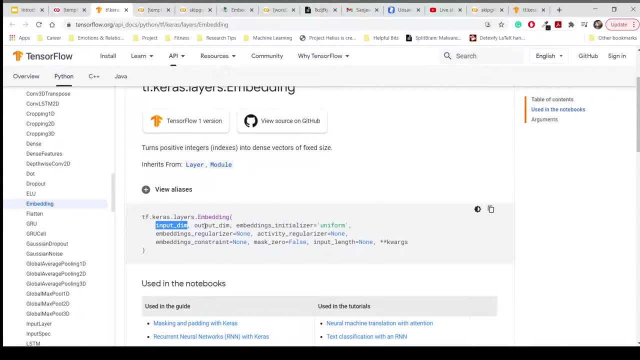 Okay, So this is kind of like a standard layers with input dimensions and output dimensions. right, All of these are variables you don't have to care about unless you're doing like advanced stuff which involves like importing like an embedding layers that you trained before, something like that. 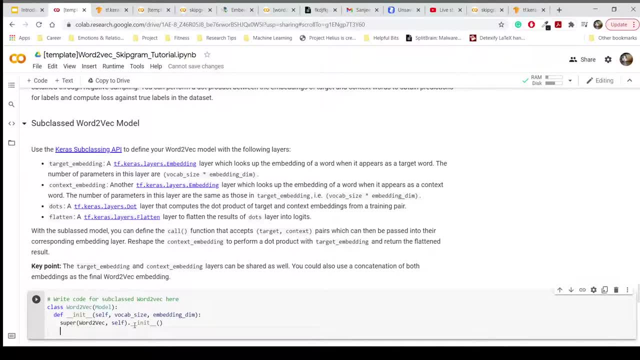 So what we're trying to go for here is that we have to define a context, a target embedding layers that encode to target. what are we trying? Okay, To encode, like the target word in training sample. So we create a target embedding layers. 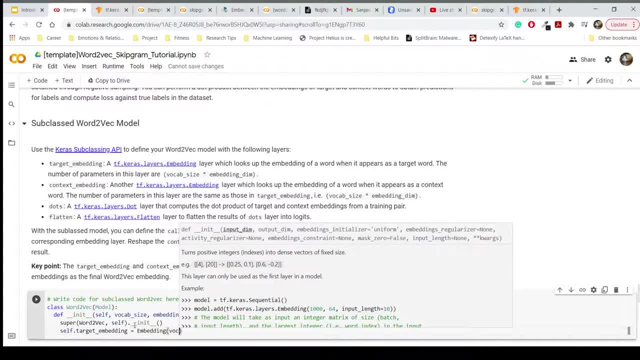 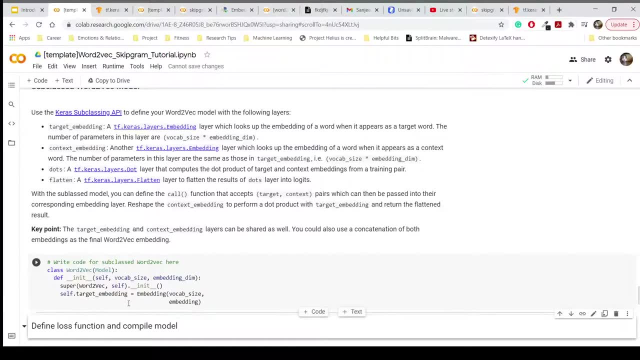 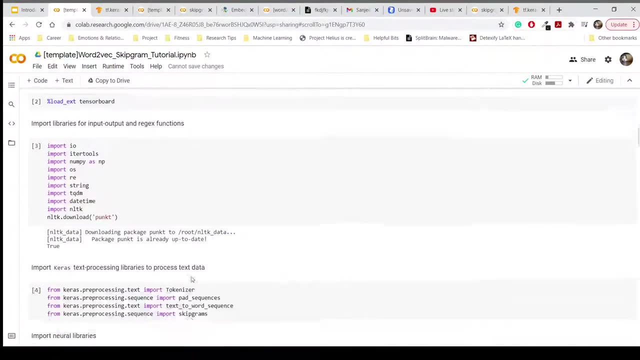 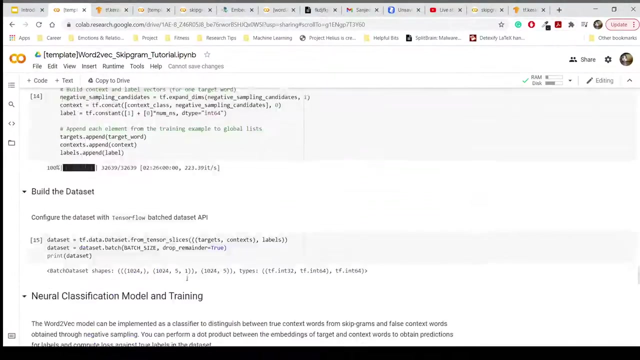 Embedding with embedding class Vocab size is basically the vocab size we take a look before Embedding dimension Here. so here we set the embedding dimension somewhere. Wait, where did I set that Okay? Oh yeah, we put it in layers. 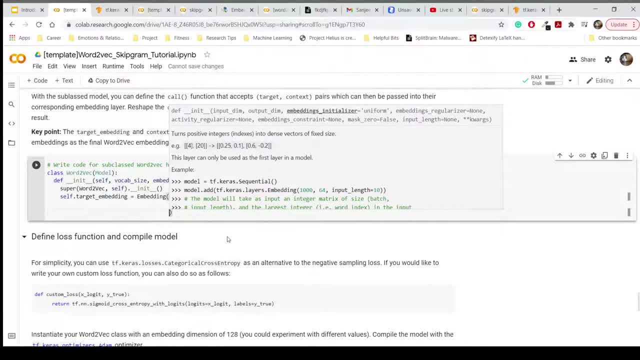 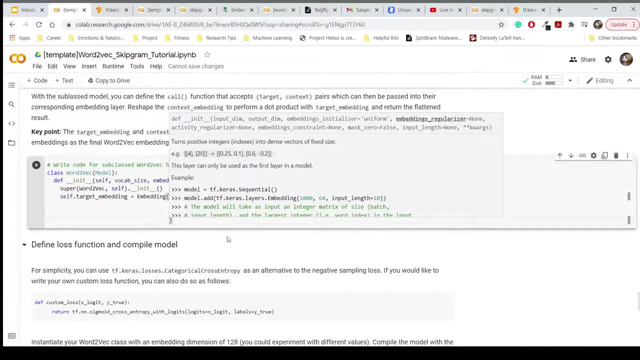 So okay, So we just have embedding dimension here. Input length is one, because we only have like one positive, instant positive. No, we just have one target word, right. So the input length is one And name to this thing. We assign a name to this embedding layer. 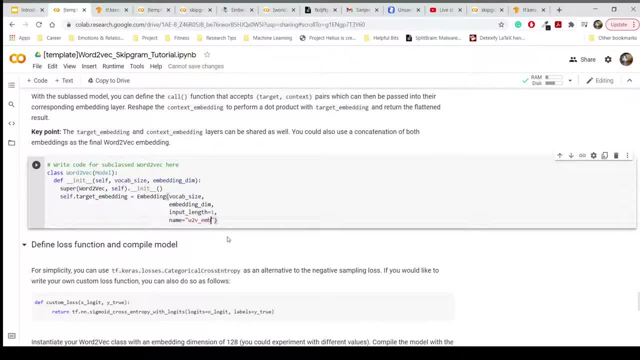 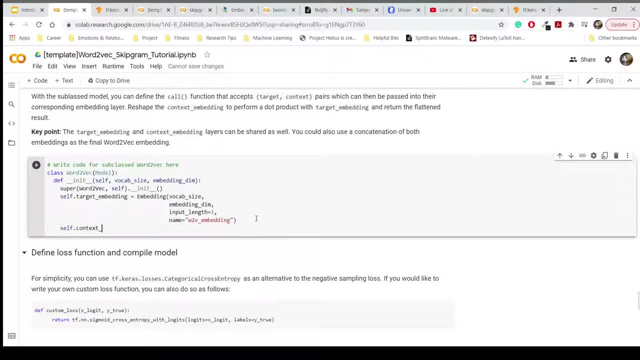 So that we can extract it from the model later. Embedding- All right, Setup- Context Embedding. This is the second one we take a look at. We're encoding like every single context word in the second vector we put into a model. 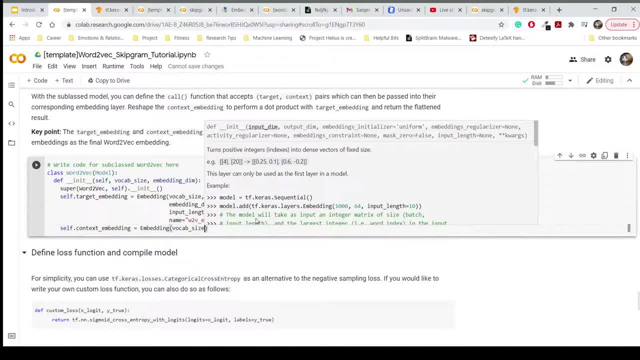 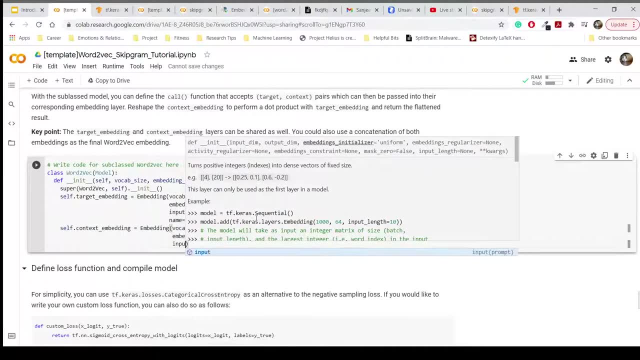 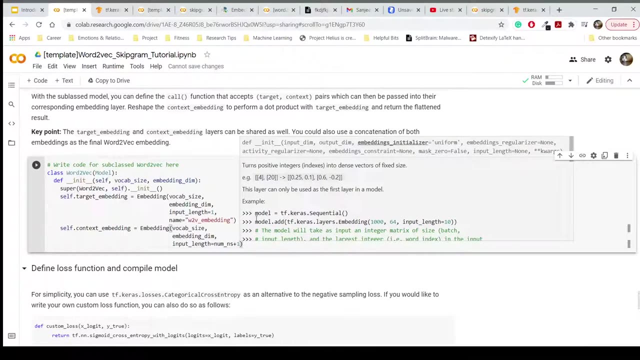 So here will be something like vocab size, like before, Same embedding dimension And input length is equal to number of negative samples plus one. Why number of negative samples plus one here? Because we have like we are putting like in the context- which consists of one positive class, right? 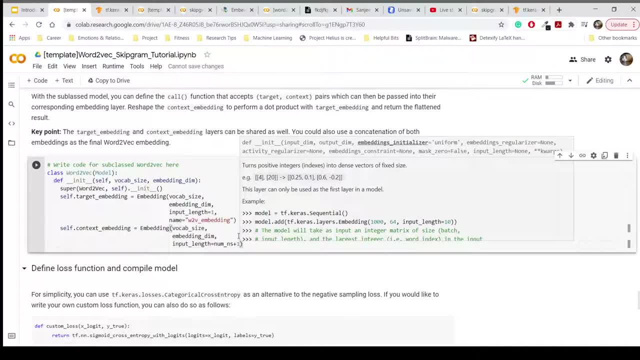 Like the class where the words actually the context or target word and some number of negative sample which it is cases for. So that's why we add one to a number of negative samples And assign it as an input length to the context embedding. 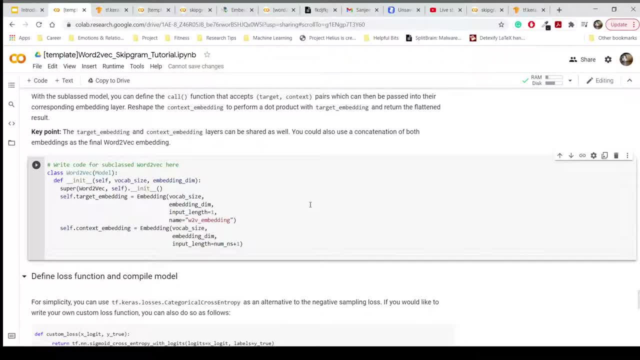 And to calculate the similarity between these vectors we use the dot layers. Why we use dot here and not the cosine is because cosine is actually a normalized versions of the dot product similarity matrix. But why is this normalized? Because the length of the word vector is typically defined by the frequency of the dot. that word right. 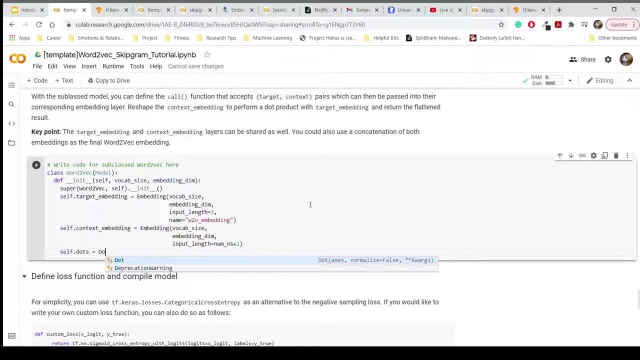 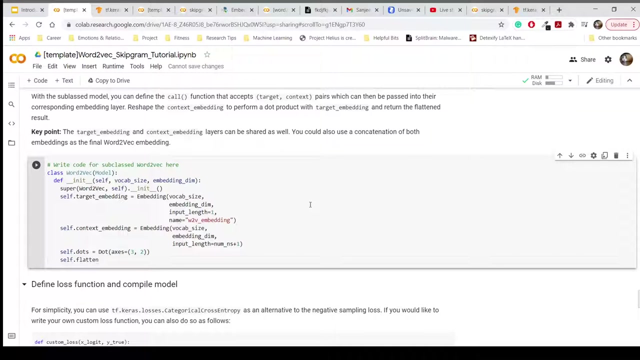 So we need to normalize it. But in this case we don't have to. We can just take a dot product here in our neural model. Asus will be equal to three and two And we just flatten the thing to return Okay. 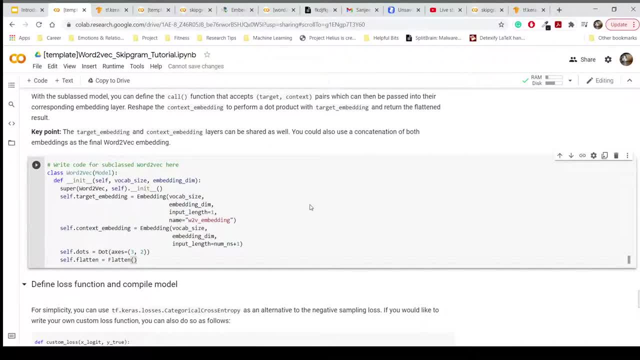 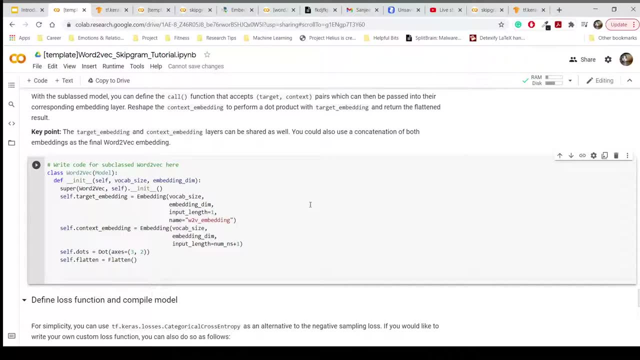 Now that we have defined our kind of layers that we're going to use, we're going to create, We define like a call routine to like the neural model itself, So we call itself. What the call routine do is that we take out some input. 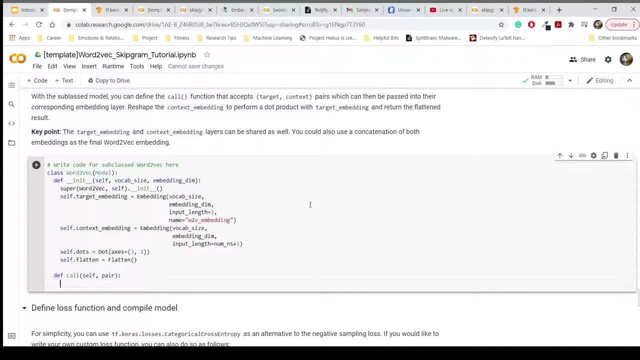 And we generate output from that. So the input we're taking here is a target word And the context of that target word And that is from the pair information that we see from the model. So we get equal to pair. Regenerating the embedding layers. 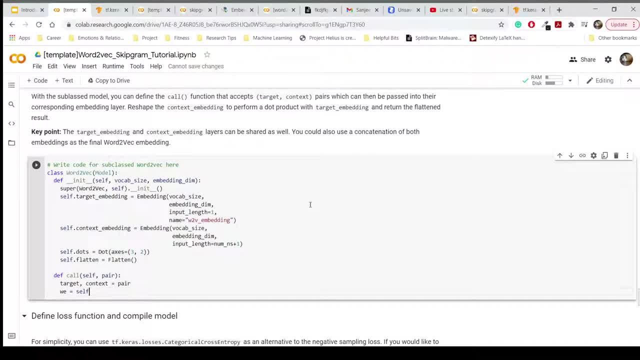 The word embedding layers. right, That is the target embedding That we defined up there with the target, So we can encode the target word itself. And for the context embedding we just use the context embedding layer that we defined, But this time with the context. 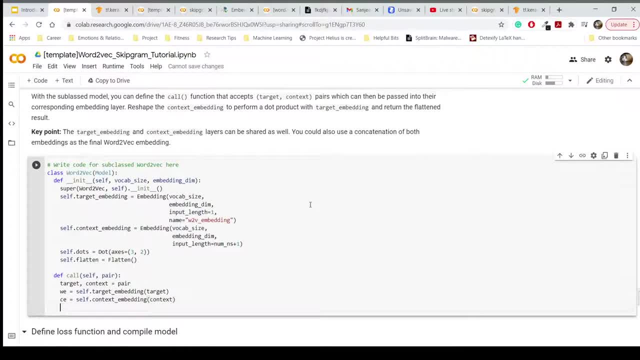 So that we can like encode the context words, We dot them, Calculate the dot, product Dots, The context embedding And the word embedding, So we know how similar each target word to the context word are, So that we can know how to classify them as because or not. 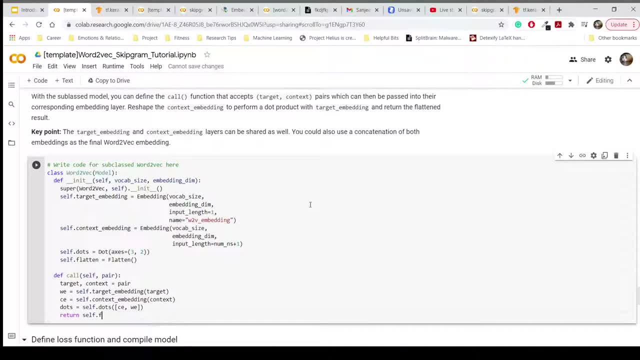 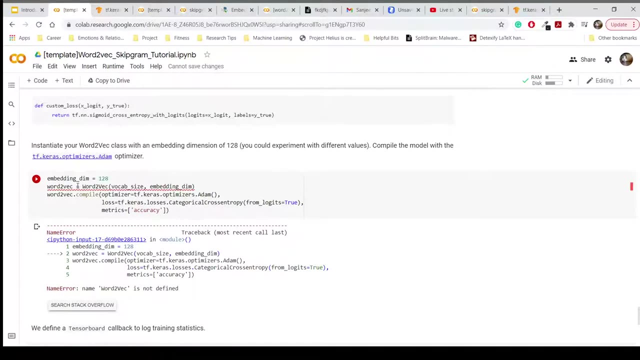 Right And then return The flattened versions of the dot product Now that we can model. Okay, This here we got an error because we haven't defined the model, But now we define the model, We will not no longer get that errors. 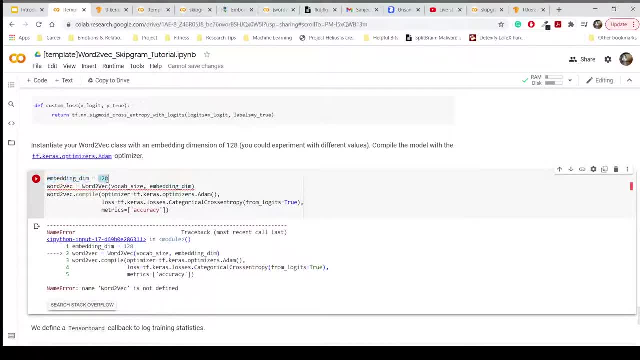 We set the embedding dimensions here as 128.. So originally each vector is like, Each word vector will be like a thousand units long or more, Right, But now, getting out of this, Each vector, Word vectors, We have like a length, of like 128.. 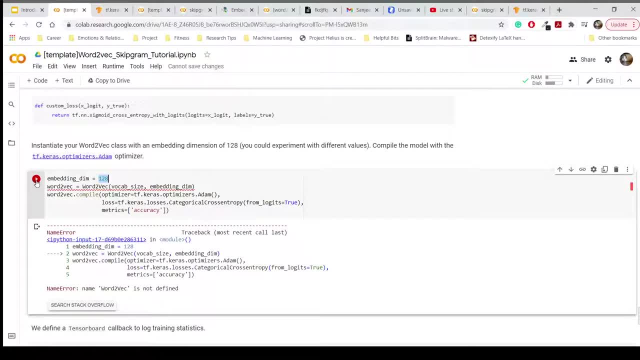 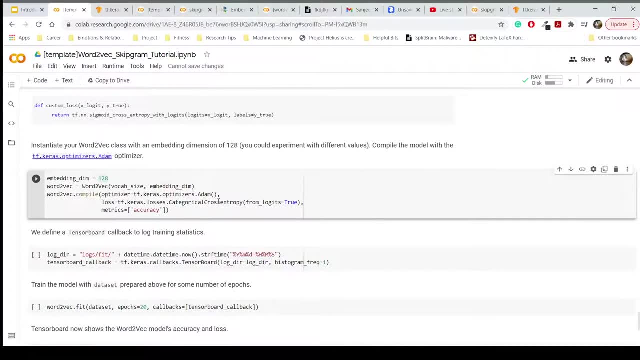 Encoding more meaningful information than sparse vector. And now we train the model For loss function. We just use categorical cross entropy Because It's like we're getting it from logic, Right. We just calculating the raw score, We just unnormalize for the model. 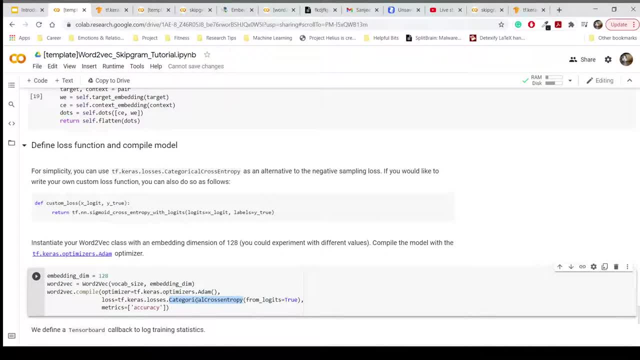 That's why we have to set for logic to true And we use categorical cross entropy, Because we are having like Five, Five vectors, Five labels to classify at once. Okay, So, So, So, So, So So. 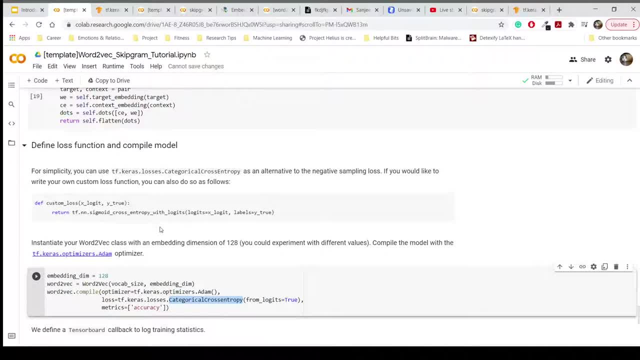 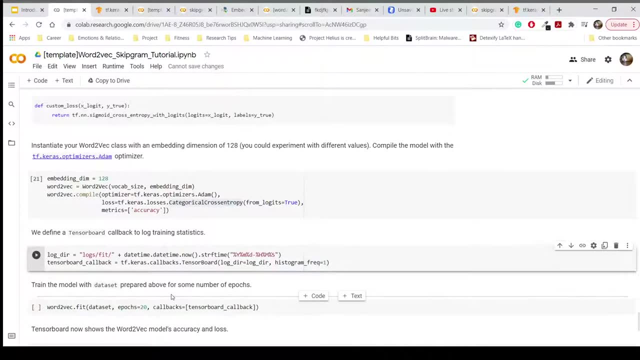 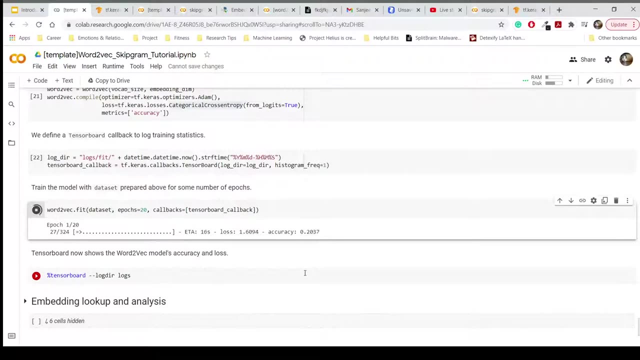 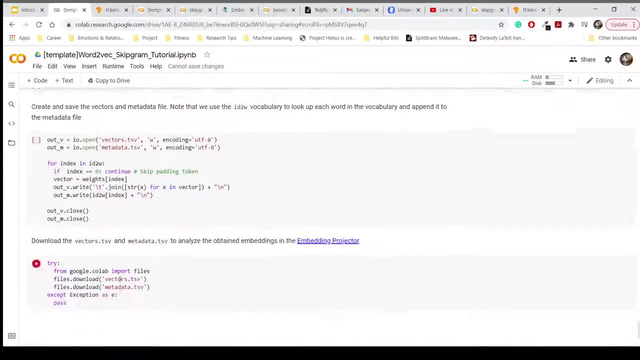 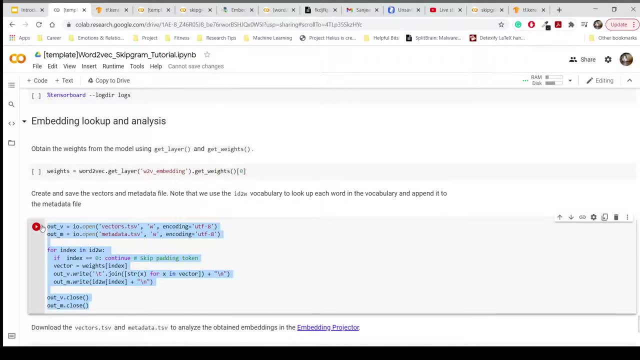 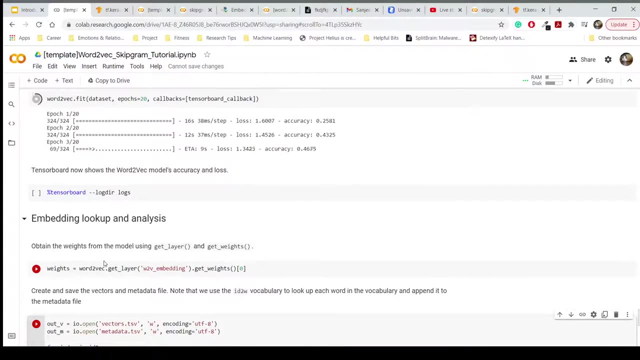 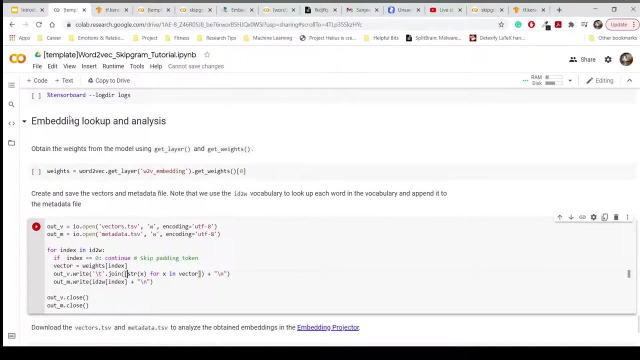 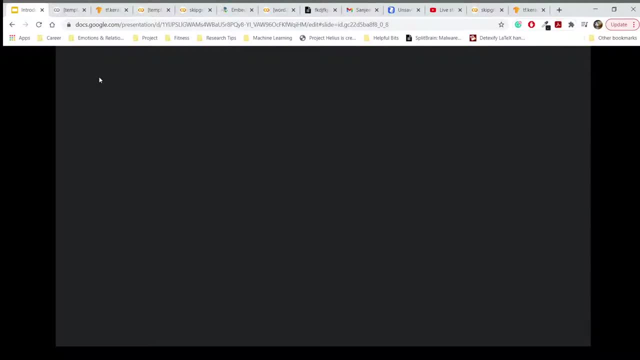 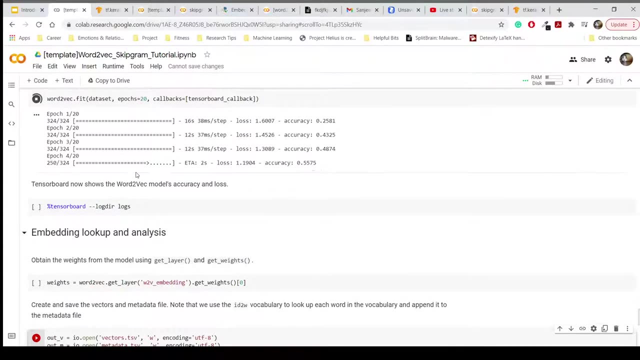 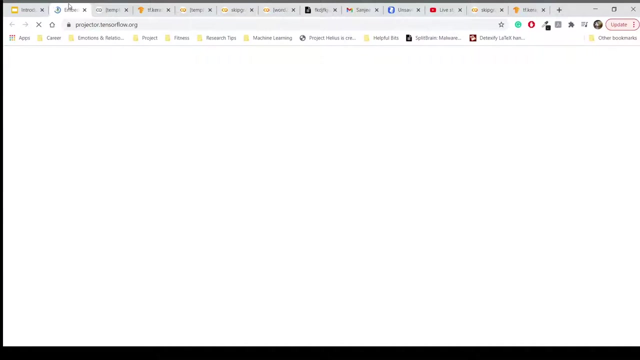 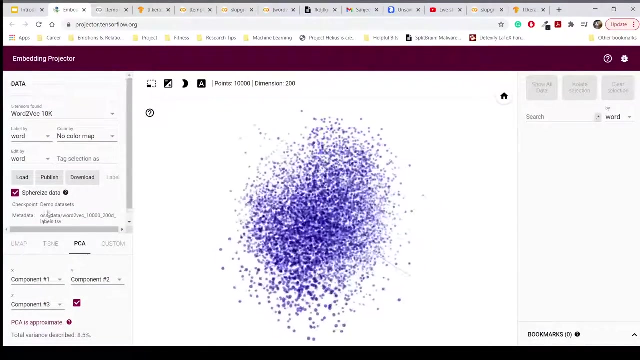 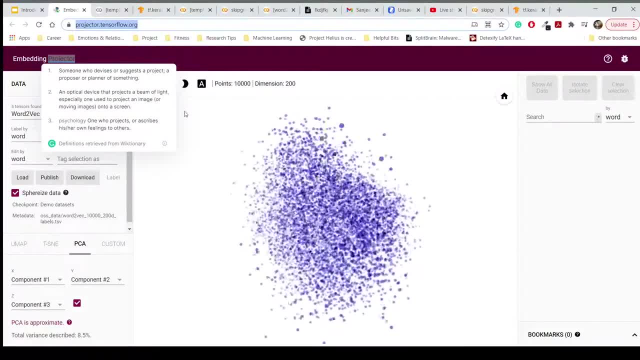 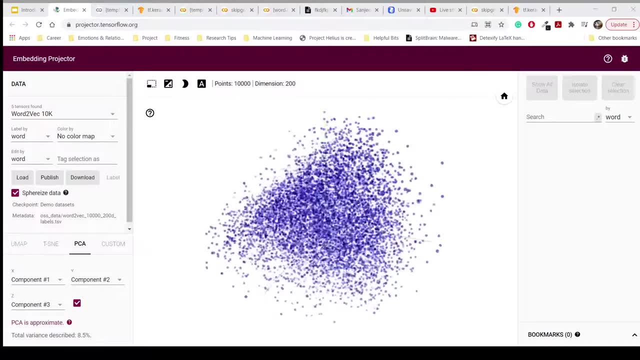 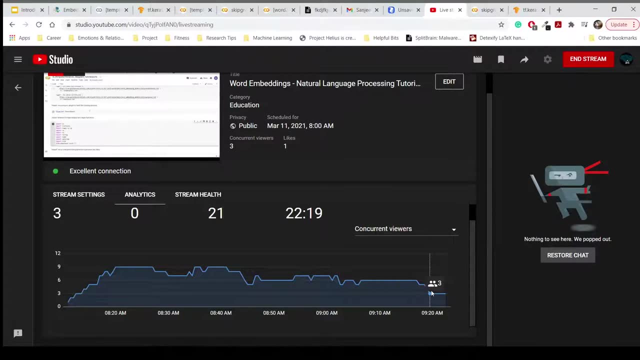 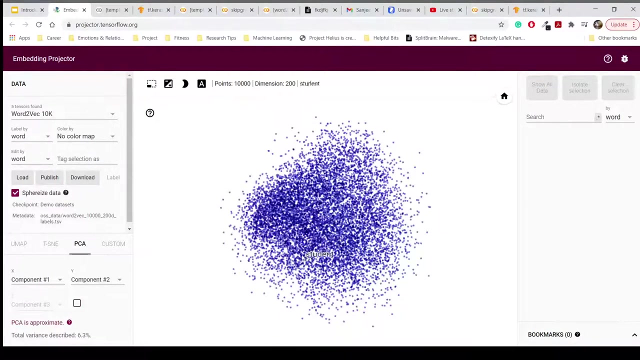 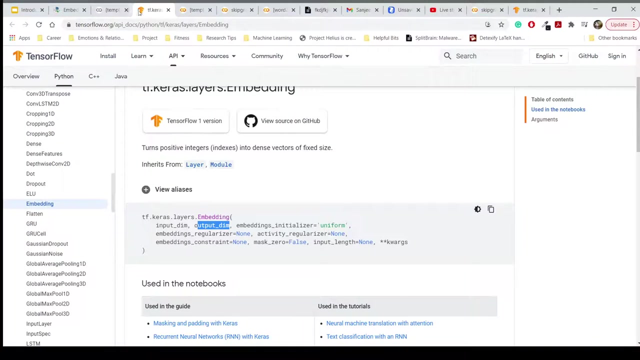 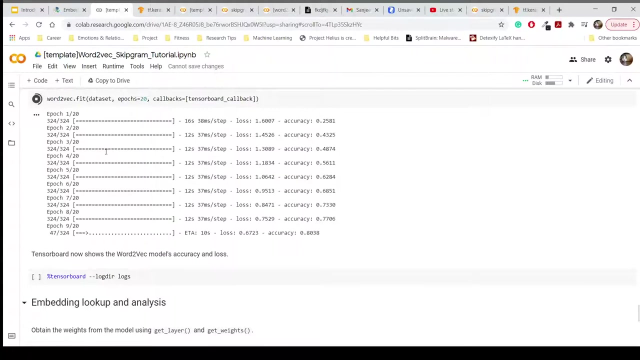 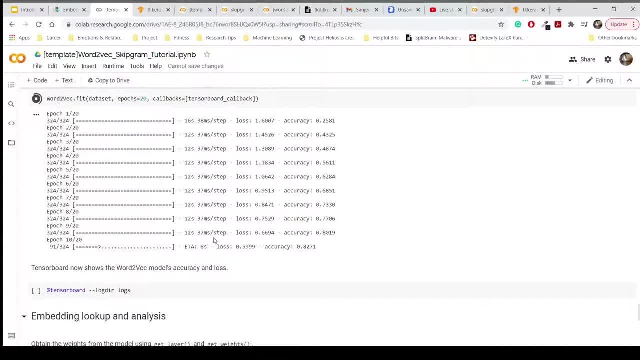 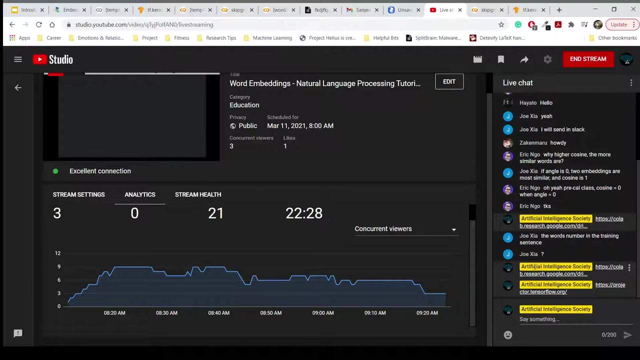 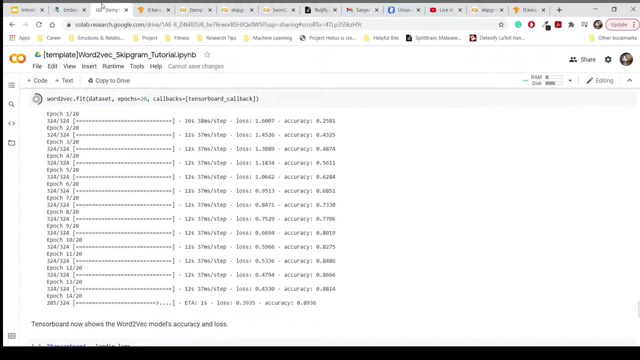 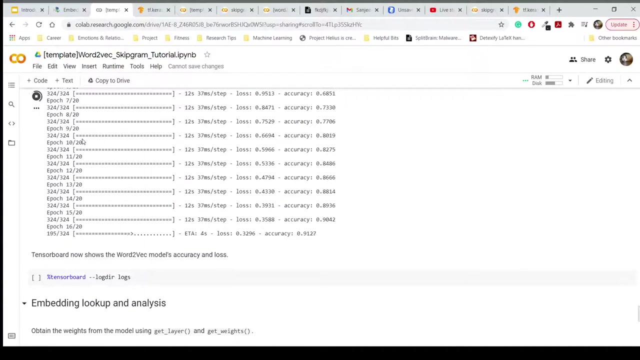 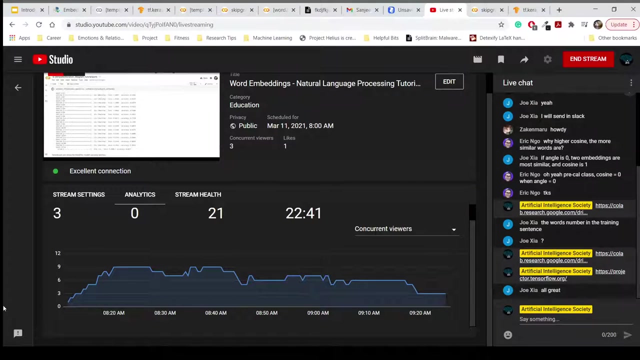 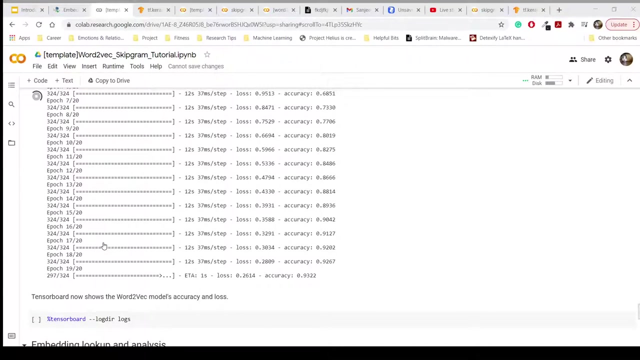 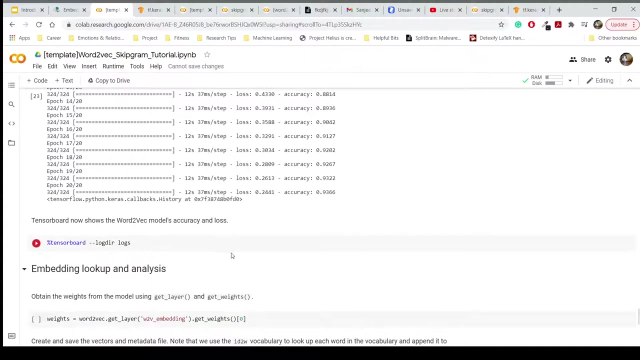 so, yeah, it's getting more and more accurate. everyone have any questions. so far, all right, all right. so so, so, so, so, um, um, um, um, um, um. okay, so i'm out of fish training. we can take a look at some of the training statistics here, seeing that, 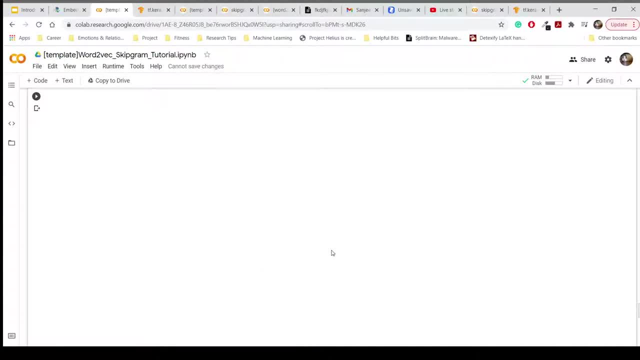 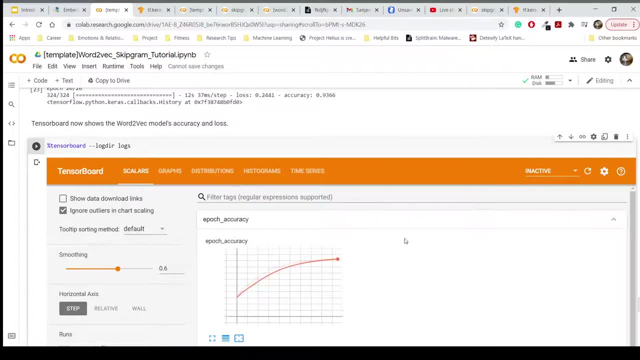 accuracy is accuracy is increasing the loss, and more is increasing the loss. and more is increasing the loss and more is decreasing, decreasing, decreasing. that our roof is being fitted pretty, that our roof is being fitted pretty, that our roof is being fitted pretty nicely, all right. and we visualize that in terms 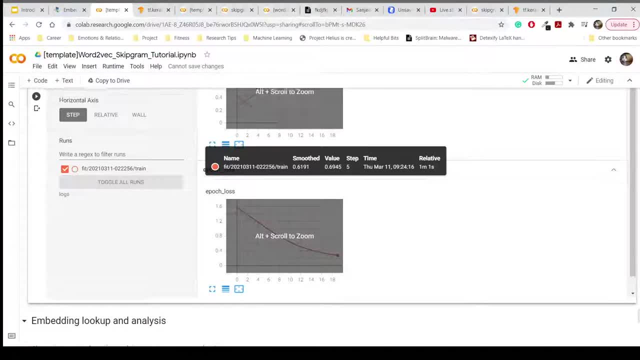 all right, and we visualize that in terms. all right, and we visualize that in terms of what you see a nice curve here, of what you see a nice curve here, of what you see a nice curve here getting closer to perfection, getting closer to perfection, getting closer to perfection. all right, 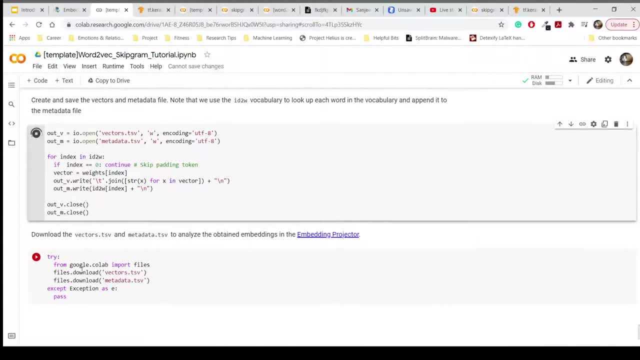 so, now that we are already training, so now that we are already training, so now that we are already training models, we just get the weights for the models, we just get the weights for the models. we just get the weights for the models and we use them to. 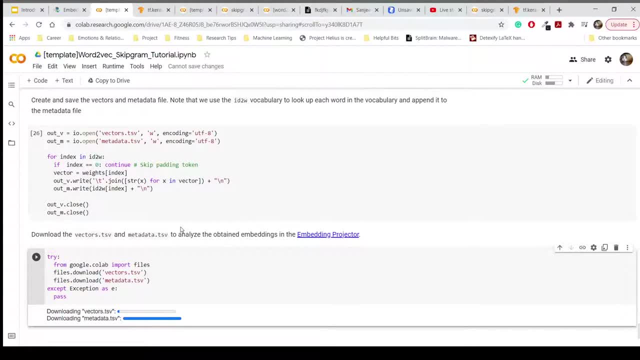 models and we use them to models and we use them to look at what we have, look at what we have, look at what we have. we have them up so we can put them in. we have them up so we can put them in. we have them up so we can put them in the visualizer. 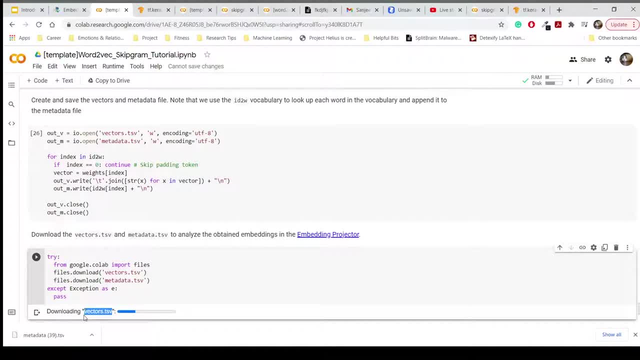 the visualizer. the visualizer, the vector files is a bit big because we, the vector files is a bit big because we the vector files is a bit big because we are downloading every single vector, so are downloading every single vector, so are downloading every single vector, so every single word in the vocabulary. 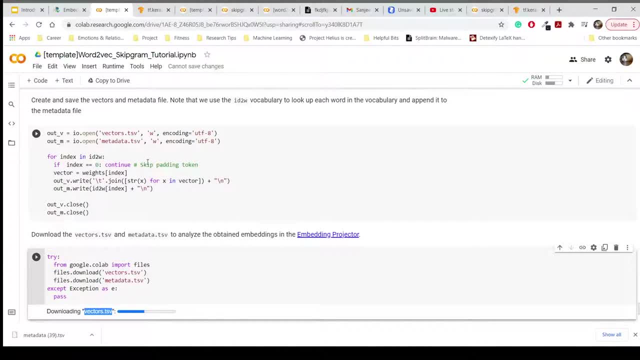 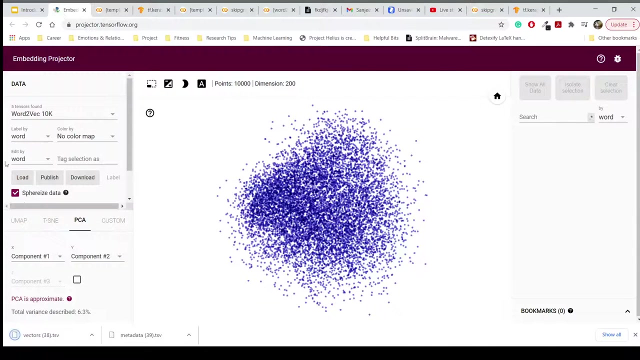 every single word in the vocabulary, every single word in the vocabulary. that's gonna take a while. that's gonna take a while. that's gonna take a while, all right. so here we just load the data. all right, so here we just load the data. all right, so here we just load the data from. 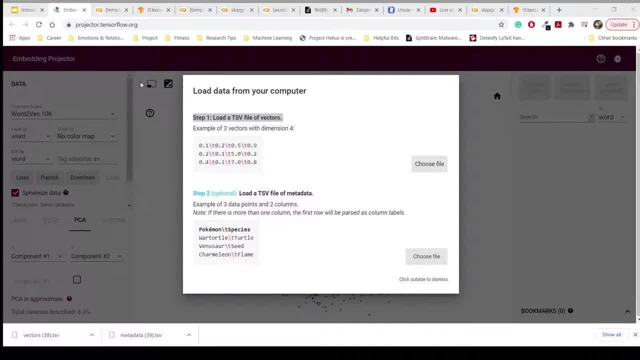 from from model no tsv5 vectors. right, we can just model no tsv5 vectors. right, we can just model no tsv5 vectors. right, we can just load it here. load it here. load it here. this is a vector files where we have the. this is a vector files where we have the. 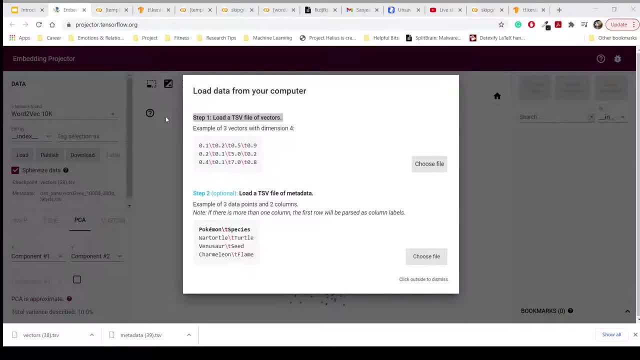 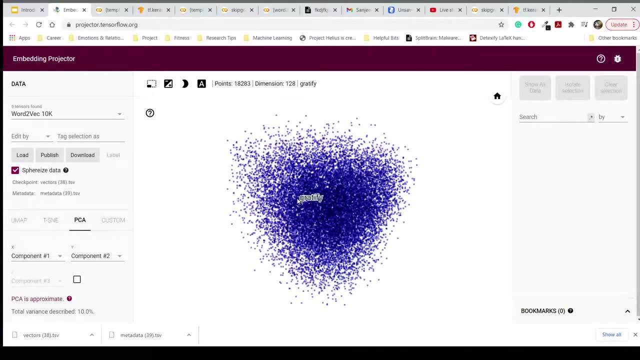 this is a vector files where we have the actual word vectors, actual word vectors, actual word vectors and the file metadata which has the list and the file metadata which has the list and the file metadata which has the list of words, of words, of words according, according to each vectors. 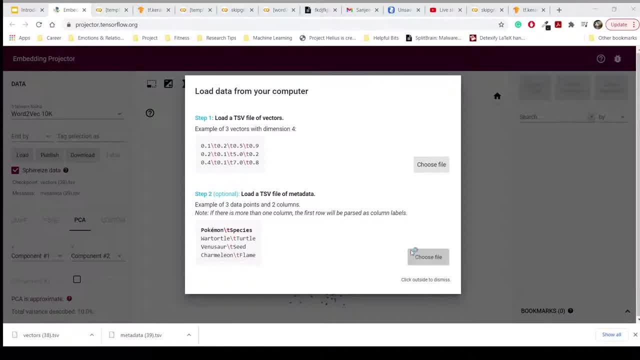 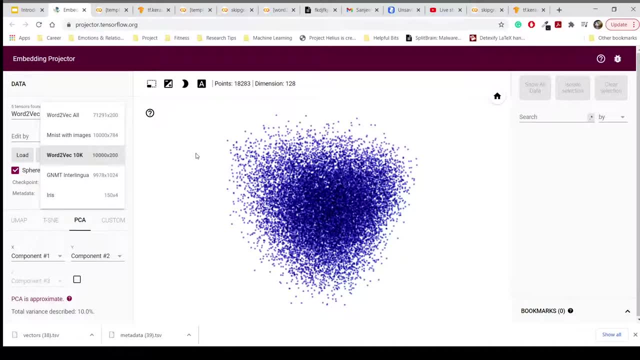 vectors, metadata, all right, so here, all right, so here, all right. so here it's a, it's a. it's a visual, visual, visual, visual and visual, and visualizations of, and visualizations of, and visualizations of what we trade. this is a very very what we trade. this is a very very. 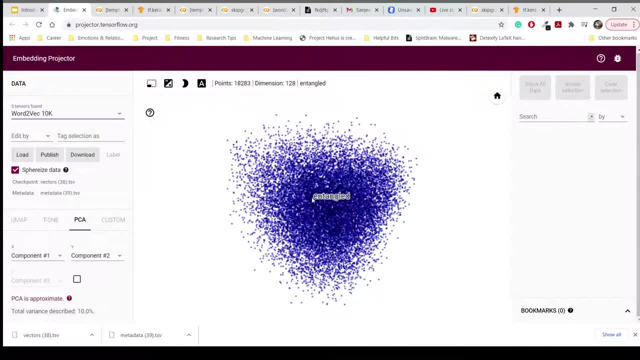 what we trade. this is a very, very confusing clowns of points, right, confusing clowns of points, right, confusing clowns of points, right. but if we could just one thing, but if we could just one thing, but if we could just one thing: entangle right, entangle right. 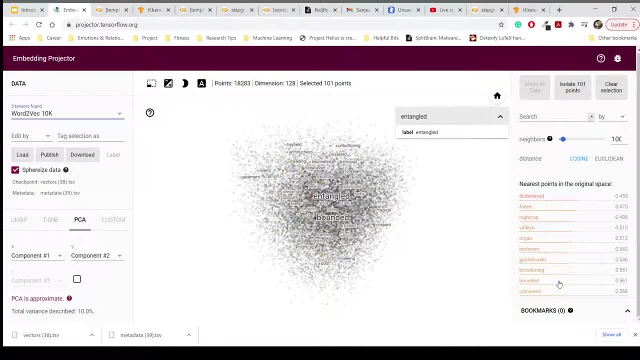 entangle right. you can see that here are the list of. you can see that here are the list of. you can see that here are the list of words that's like most similar to it. words that's like most similar to it. words that's like most similar to it, tell it, but like how much? how similar to. 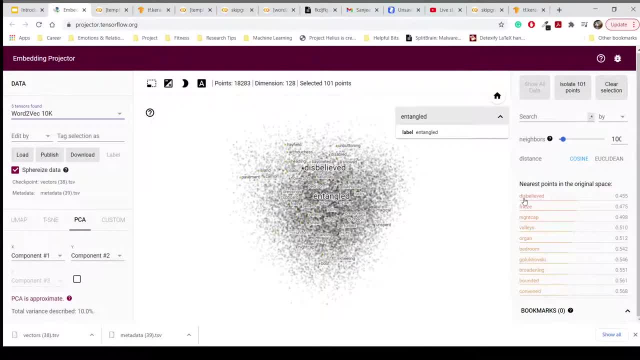 tell it, but like how much, how similar to tell it, but like how much, how similar to it is. it is, it is and and, and you can see here this belief is, you can see here this belief is, you can see here this belief is really really close to entangle, so just, 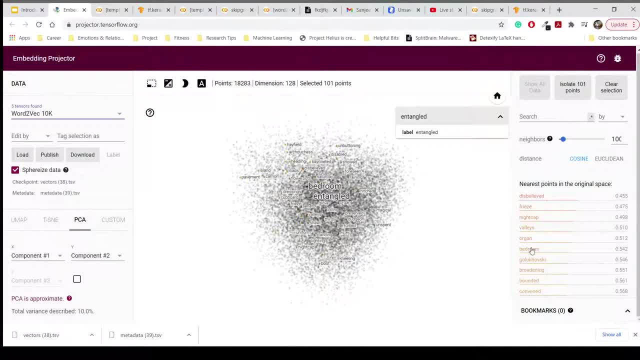 really, really close to entangle, so just really, really close to entangle. so just think about this. that might be some kind. think about this. that might be some kind think about this. that might be some kind of similarity, right of similarity, right of similarity, right. let's just take a look at like a downward 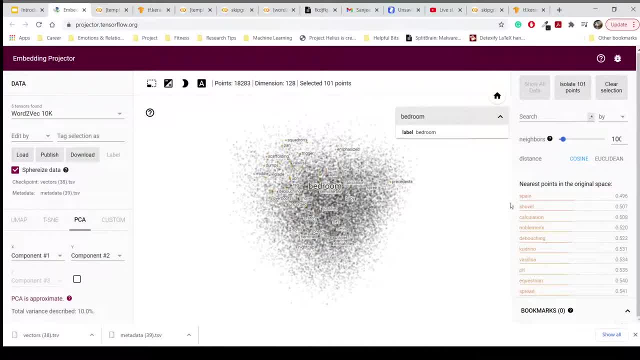 let's just take a look at like a downward. let's just take a look at like a downward bedroom, bedroom, bedroom, okay. why is bedroom similar to spain? okay? why is bedroom similar to spain? okay, why is bedroom similar to spain? that's a good question. 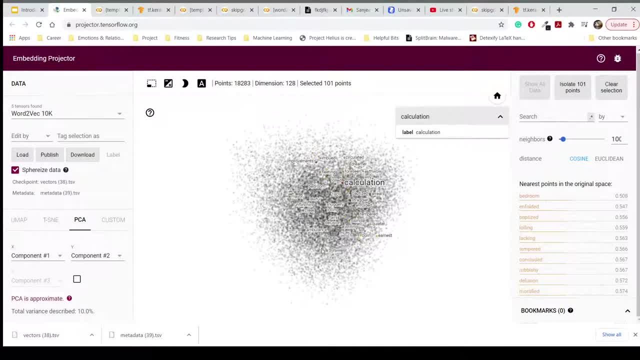 why is calculation? similar bedroom. maybe we'll just have some kind of weird. maybe we'll just have some kind of weird. maybe we'll just have some kind of weird. things that we don't know, things that we don't know, things that we don't know or encountering is really similar. 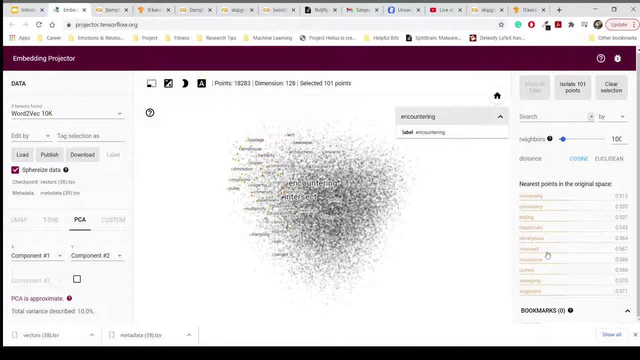 or encountering is really similar, or encountering is really similar. linking, linking, linking. this is very interesting to intersect. this is very interesting to intersect. this is very interesting to intersect. which is like kind of like. which is like kind of like. which is like kind of like. oh yeah, we're just meeting together in. 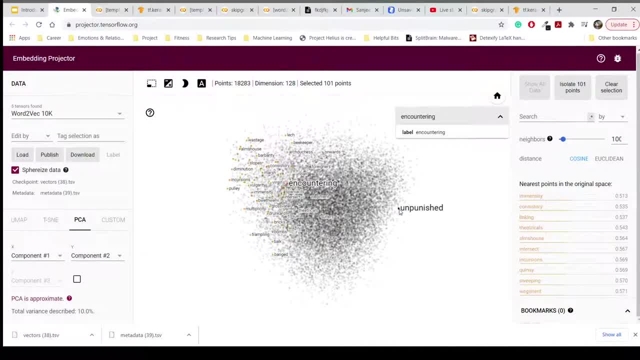 oh yeah, we're just meeting together in. oh yeah, we're just meeting together in some way or another right, some way, or another right, some way, or another right, all right, all right, all right, it's ramping, sorry, rusty scar, rusty scar, rusty scar. this one a very, very like. 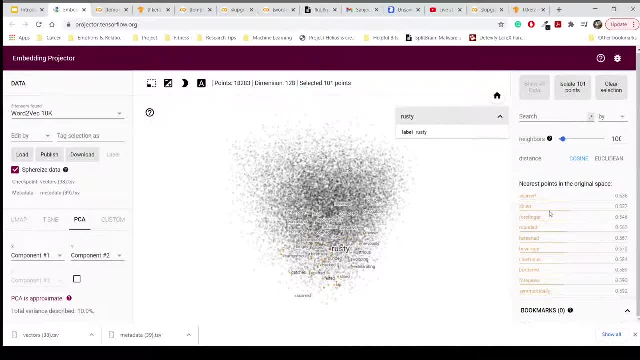 this one, a very, very like this one, a very, very like a very good example. you can see that, a very good example. you can see that a very good example. you can see that rusty here is really close to scar and rusty here is really close to scar and 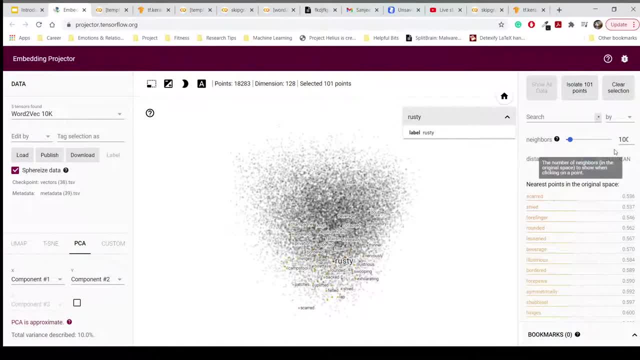 rusty here is really close to scar, and we can all see what this, we can all see what this, we can all see what this similarity, similarity, similarity, them is right, them is right, them is right, all right. so that's the visualization of all right, so that's the visualization of. 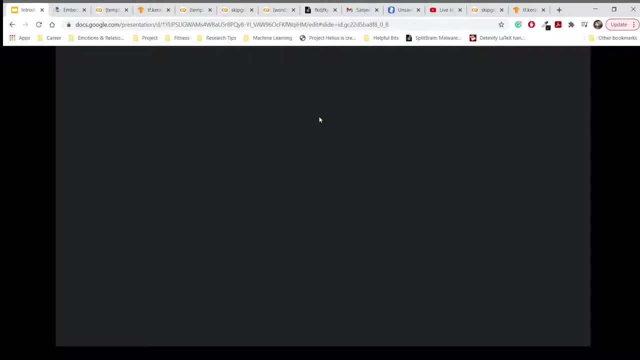 all right, so that's the visualization of how vectors turns out to be, how vectors turns out to be, how vectors turns out to be and, and, and. that's about it, that's about it, that's about it, and so, and so and so. to conclude, what's our embeddings? 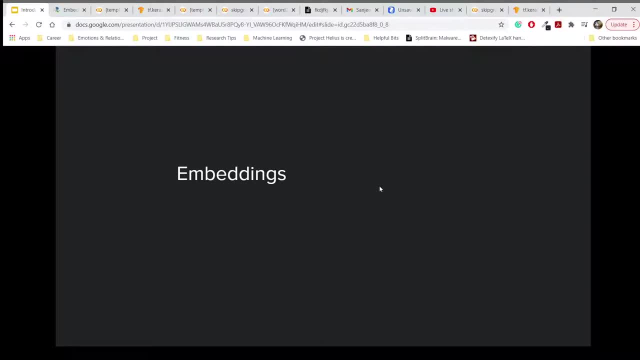 to conclude, what's our embeddings? to conclude, what's our embeddings? um, on a code, okay, on a code. okay on a code. okay, wait a minute. so emily is the way to represent text data. so emily is the way to represent text data. so emily is the way to represent text data in a meaningful manner for computers. 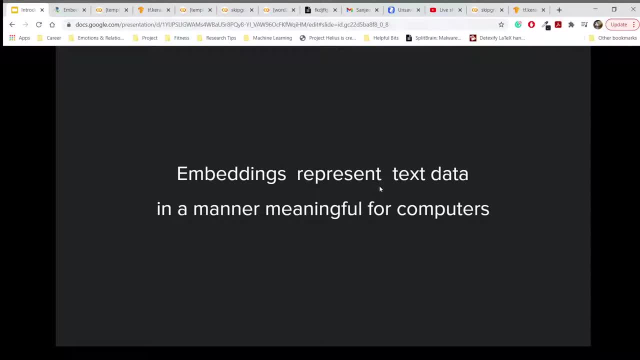 in a meaningful manner for computers, in a meaningful manner for computers and similar. it is similar to how images and similar. it is similar to how images and similar. it is similar to how images are represented by pixel values, as data are represented by pixel values, as data are represented by pixel values as data, and it's an efficient way to vectorize. 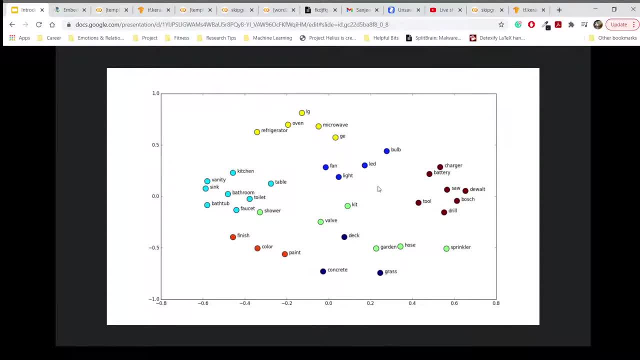 and it's an efficient way to vectorize. and it's an efficient way to vectorize non-numerical data capturing what we non-numerical data capturing, what we non-numerical data capturing, what we care about documenting text. care about documenting text, care about documenting text. part of word meanings characterized like: 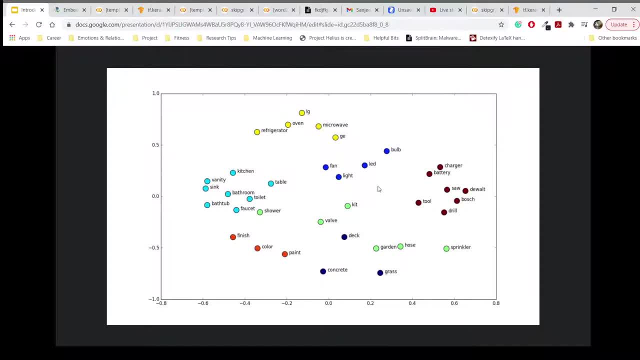 part of word meanings characterized like part of word meanings characterized like web word similarity and relatedness. web word similarity and relatedness. web word similarity and relatedness. right, right, right, and the type of what we see so far is. and the type of what we see so far is. 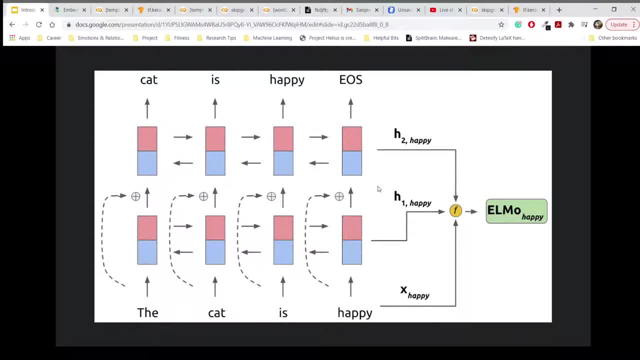 and the type of what we see so far is the status embedding. there's a more. the status embedding there's a more. the status embedding there's a more advanced way to create word emitting is advanced way to create word emitting is advanced way to create word emitting is called contextual embeddings. 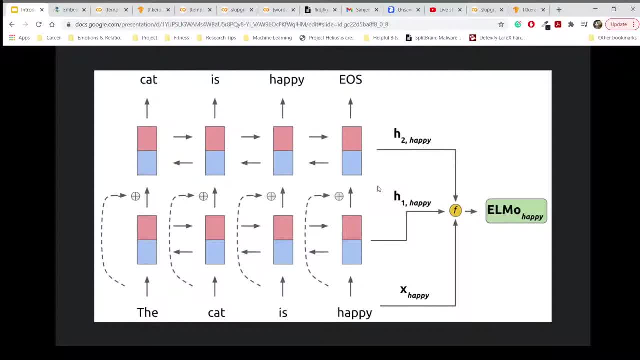 called contextual embeddings, called contextual embeddings which change the, which change the, which change the how the word is represented, depending on how the word is represented, depending on how the word is represented, depending on the context of the word itself, the context of the word itself, the context of the word itself. so, if you have a word, a word in different, 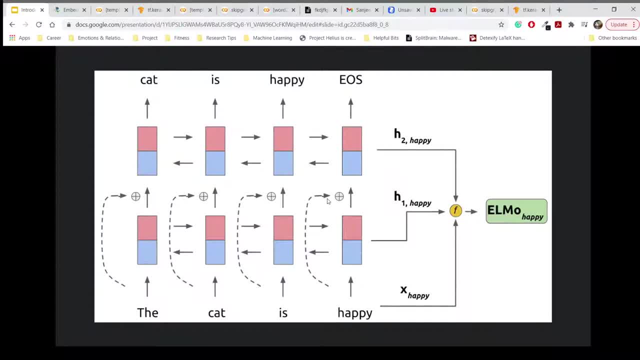 so if you have a word, a word in different, so if you have a word, a word in different sentence, you have driven embeddings sentence. you have driven embeddings sentence. you have driven embeddings and why are embedding important? and why are embedding important and why are embedding important? uh, remember that embeddings are. 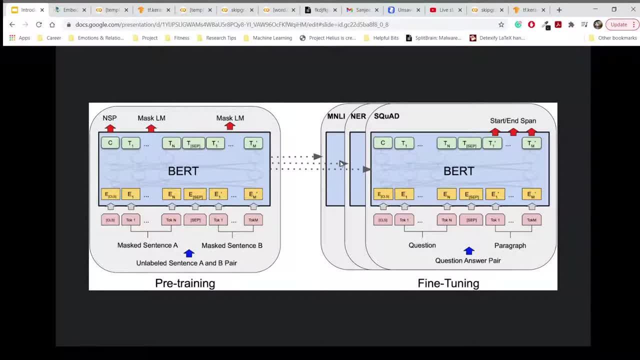 uh, remember that embeddings are. uh, remember that embeddings are learnable, right. so we learnable right. so we learnable right. so we, there we can. they can be adapt to any there we can. they can be adapt to any there we can. they can be adapt to any downstream tasks. 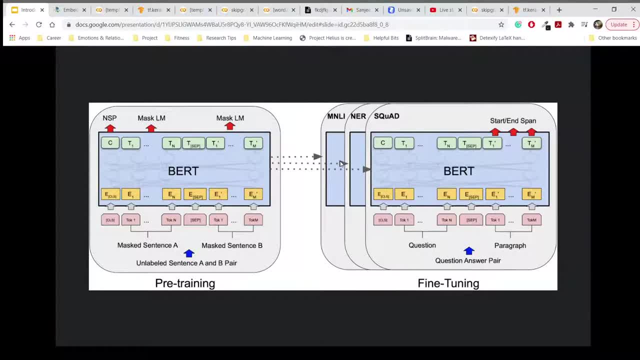 downstream tasks, downstream tasks, and should it be sentiment, and should it be sentiment and should it be sentiment. classifications or summarization, classifications or summarization, classifications or summarization, and the model to and the model to and the model to. tomorrow learn the word representations. tomorrow, learn the word representations. 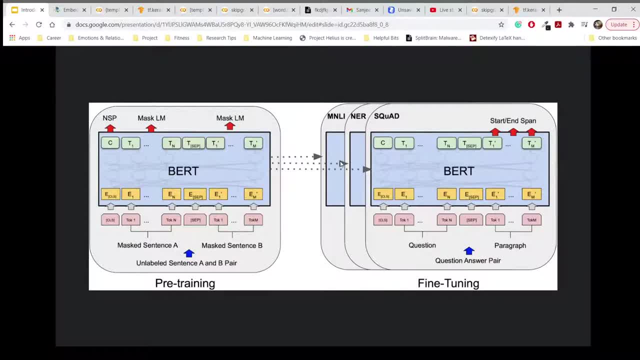 tomorrow, learn the word representations that's most meaningful for that certain that's most meaningful for that certain that's most meaningful for that certain task and change what representation to task and change what representation to task and change what representation to start information, start information, start information. and bird is a pre-trained model that 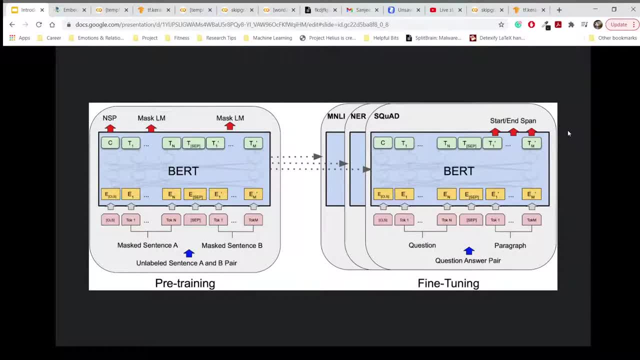 and bird is a pre-trained model, that and bird is a pre-trained model that. use a kind of everything called workpiece. use a kind of everything called workpiece. use a kind of everything called workpiece, embedding, embedding, embedding. and also birds- a very, very sophisticated- and also birds, a very, very sophisticated. 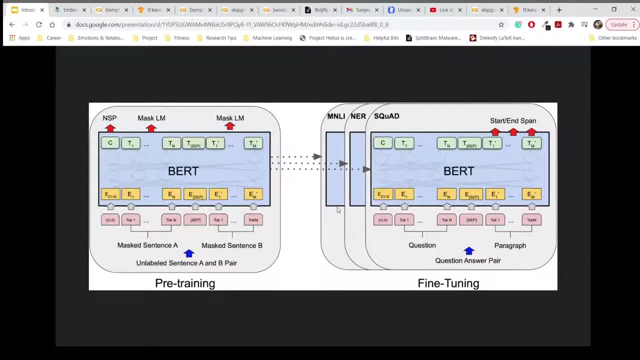 and also birds, a very, very sophisticated and language model that we're going to and language model that we're going to, and language model that we're going to take a look, take a look, take a look down the line in this workshop series, down the line in this workshop series. 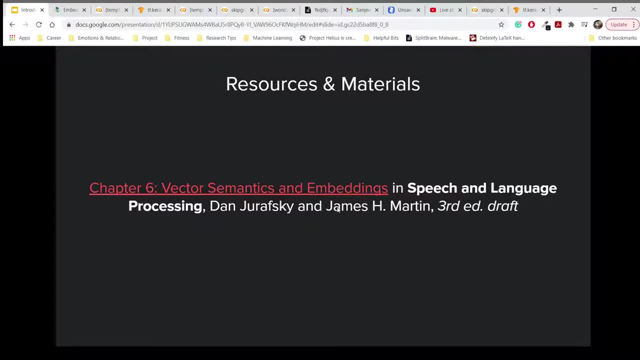 down the line in this workshop series and that's the end of our workshop. and that's the end of our workshop. and that's the end of our workshop. special thanks to, as team, for giving us special thanks to as team, for giving us special thanks to as team, for giving us opportunity to bring the 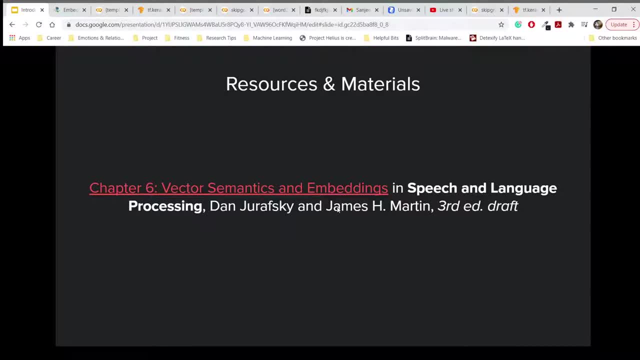 opportunity to bring, the opportunity to bring the content to you, and the workshop is an content to you, and the workshop is an content to you, and the workshop is an adaptation of material from textbook, adaptation of material from textbook, adaptation of material from textbook, speech and language processing. 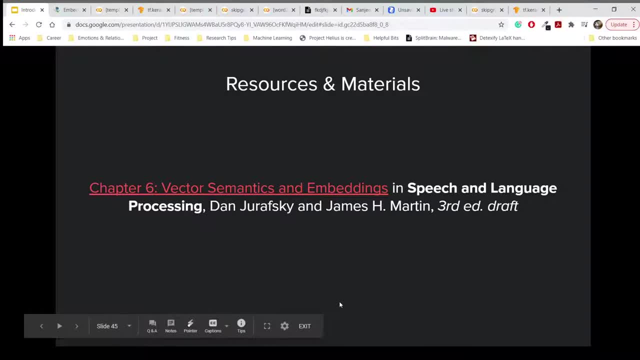 speech and language processing. speech and language processing as very wonderful textbook and as very wonderful textbook and as very wonderful textbook and annual like, but you care about nlp. you annual like, but you care about nlp. you annual like, but you care about nlp. you should probably check it out. 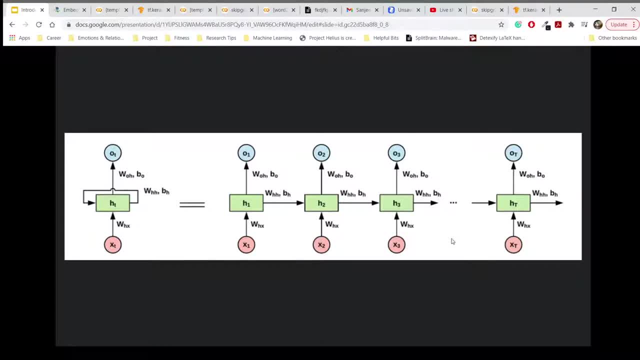 should probably check it out. should probably check it out on the next workshop series. we'll take a on the next workshop series. we'll take a on the next workshop series. we'll take a look at one more of the fundamental. look at one more of the fundamental.